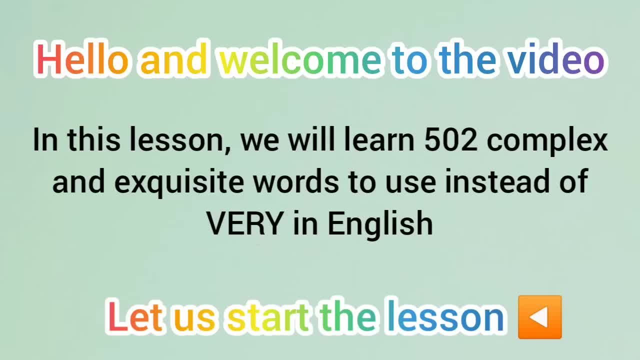 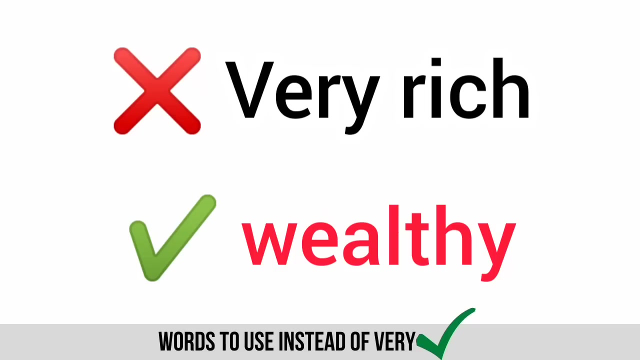 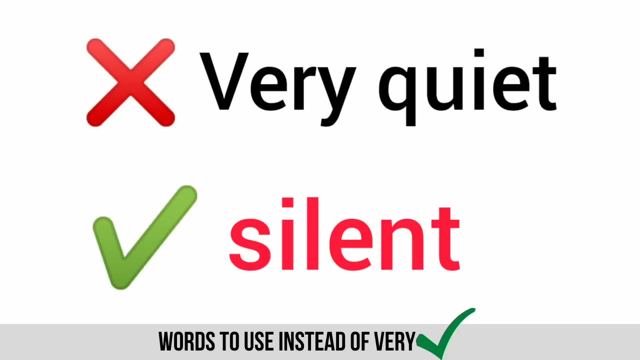 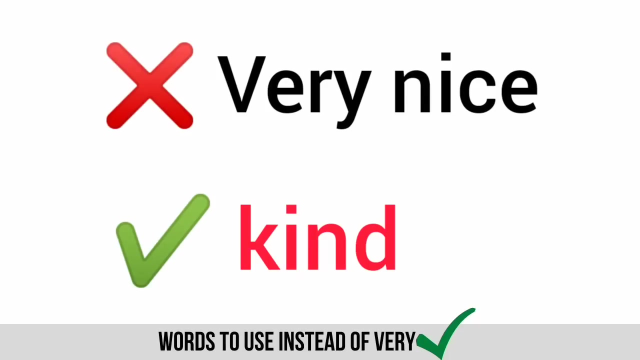 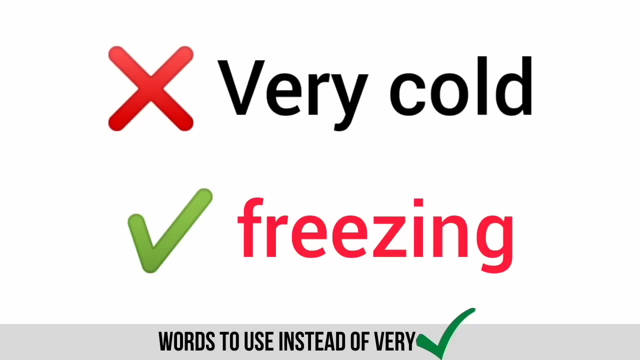 Hello and welcome to the video. In this lesson we will learn 502 complex and exquisite words to use instead of very in English. Let us start the lesson. Very quiet, Silent, Very nice, Kind, Very nice Kind, Very cold, Freezing, Very cold Freezing. 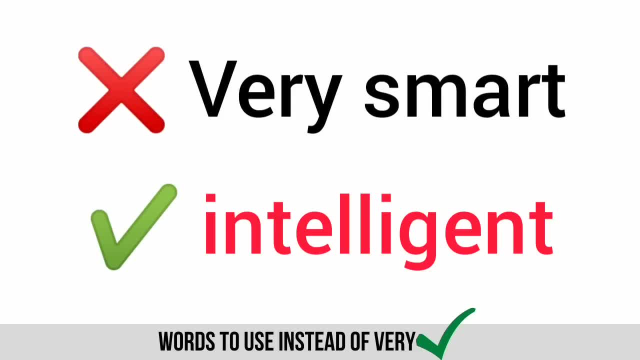 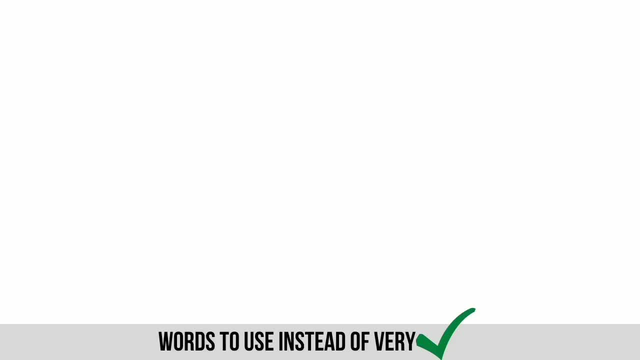 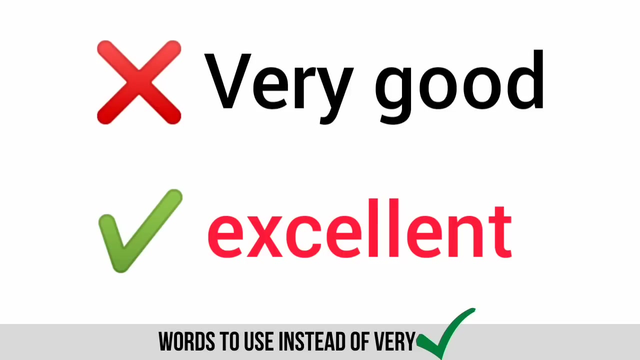 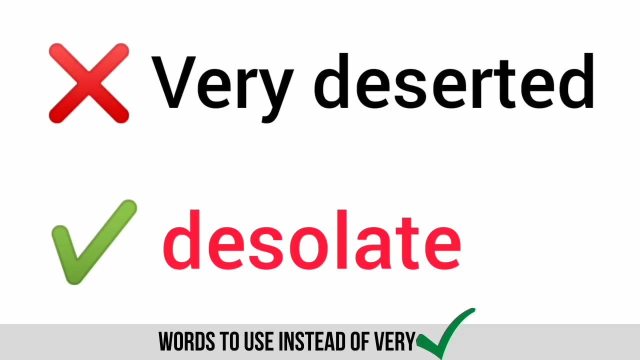 Very smart, Intelligent, Very smart, Intelligent. Very short Brief, Very short Brief, Very simple, Basic, Very simple, Basic. Very large, Huge, Very large, Huge, Very good, Excellent, Very good, Excellent. Very deserted, Desolate, Very deserted, Desolate. 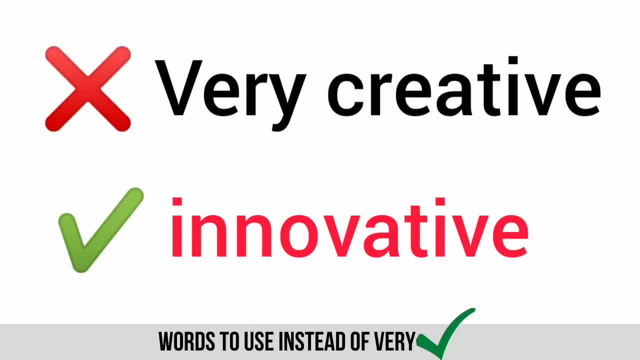 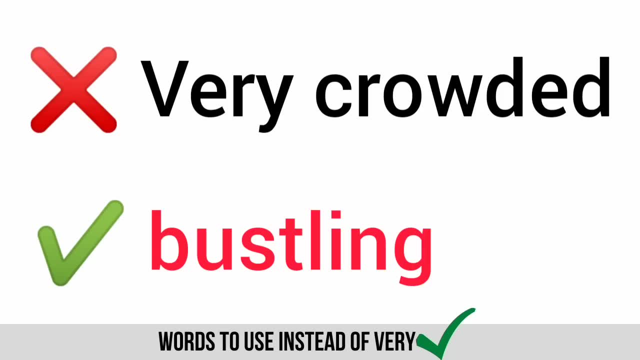 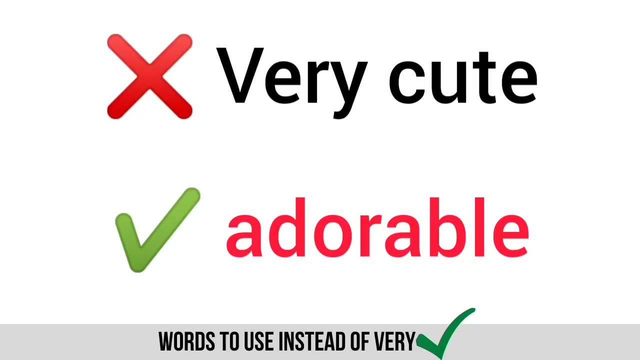 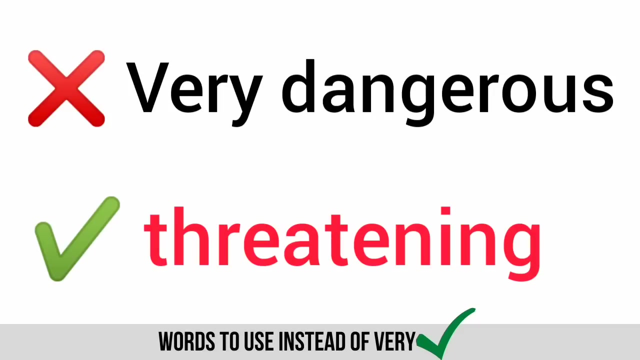 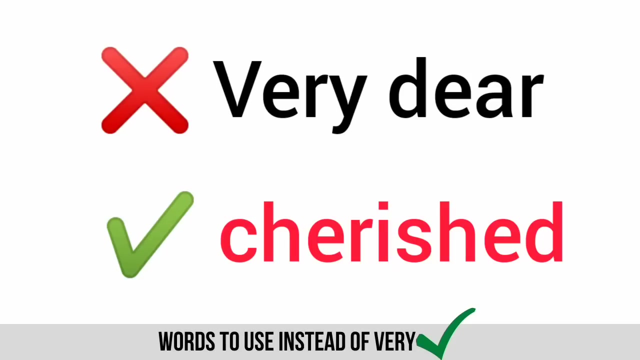 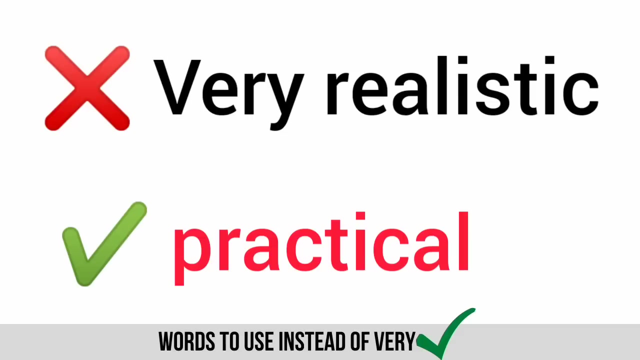 Very creative, innovative, very creative, innovative. very crowded, bustling, very crowded bustling, very cute, adorable, very cute, adorable, Very dangerous, threatening, very dangerous, threatening, very dear, cherished, very dear cherished. very realistic, practical, very realistic practical. 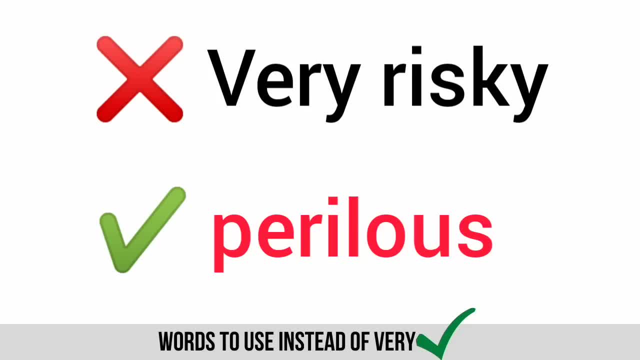 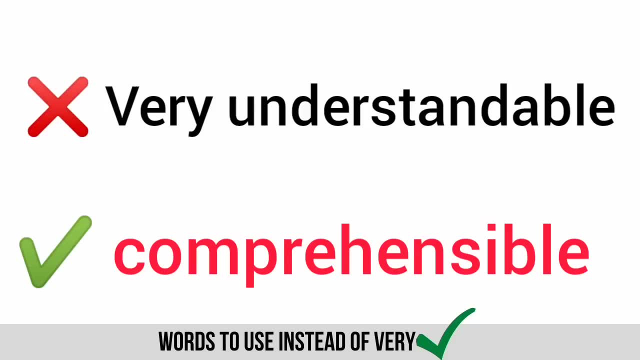 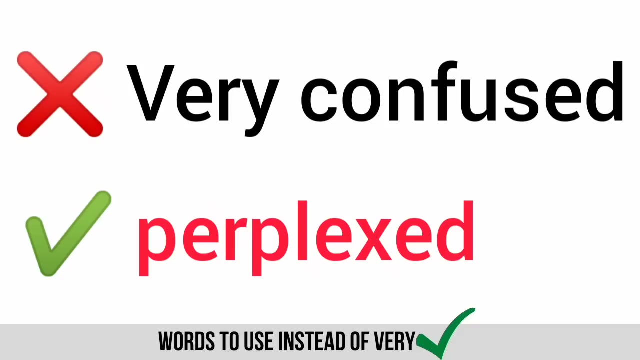 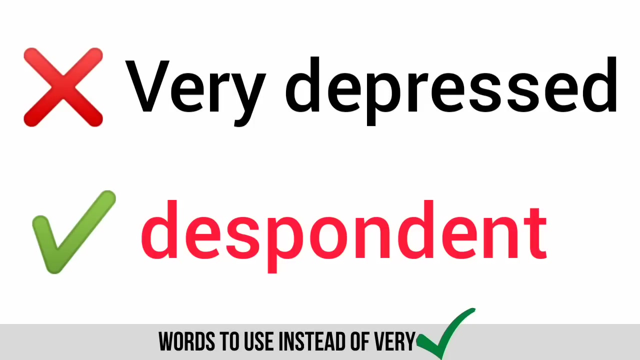 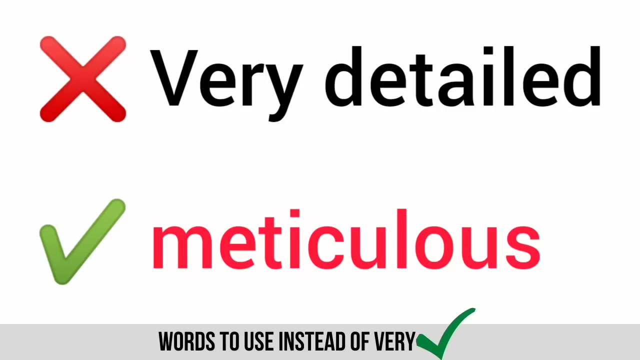 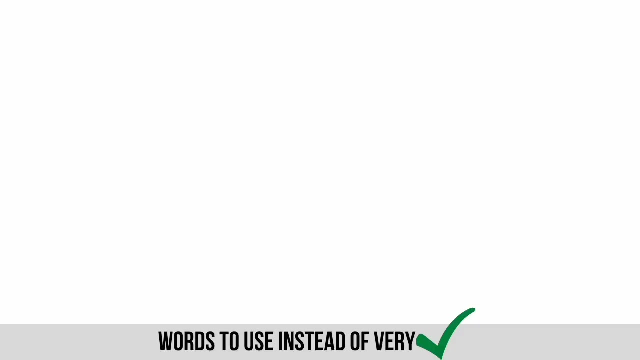 Very real, Very risky, perilous, very risky, perilous. very understandable, comprehensible, very understandable, comprehensible. very confused, perplexed, very confused, perplexed. Very depressed, despondent, very depressed, despondent. very detailed, meticulous, very detailed, meticulous. very big, massive, very big massive. 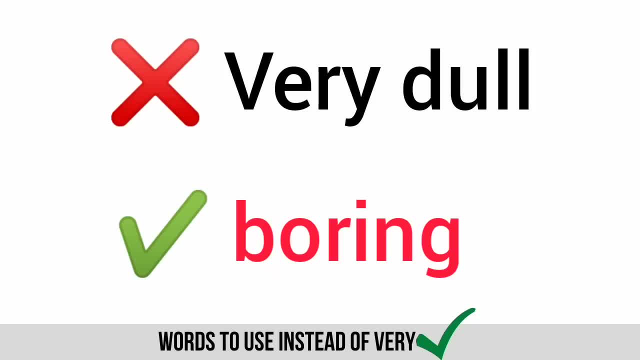 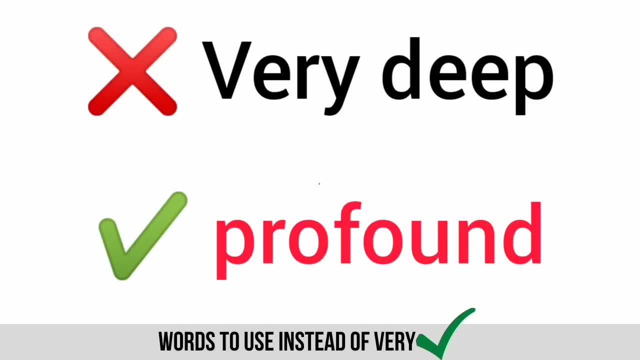 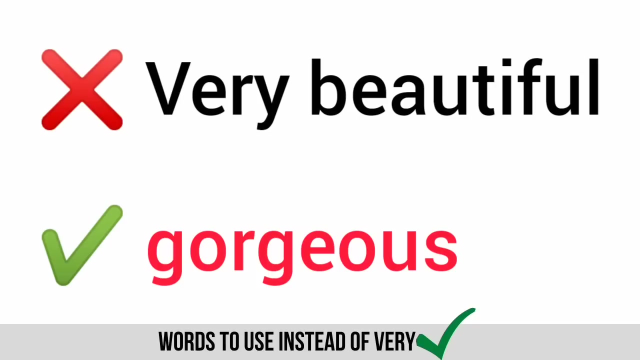 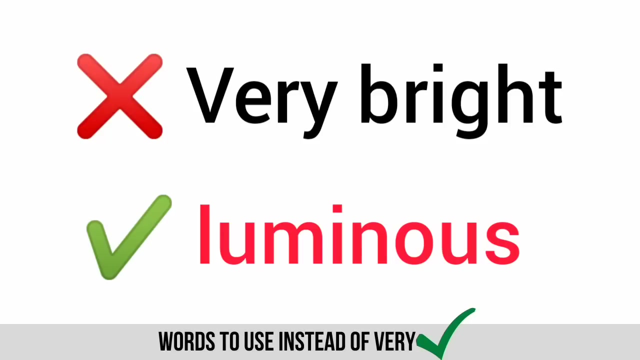 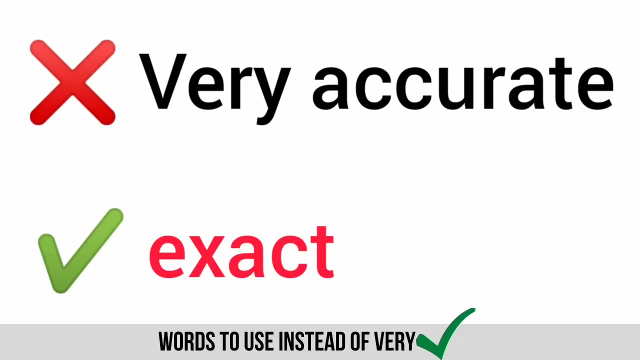 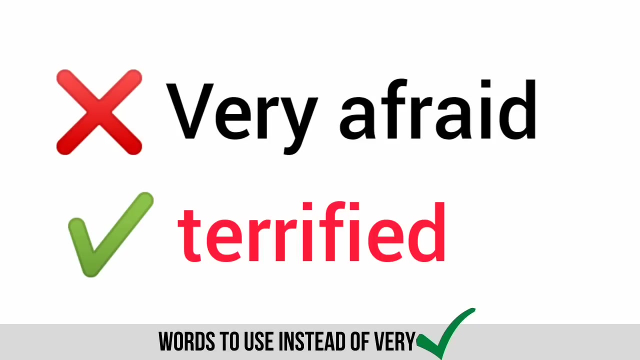 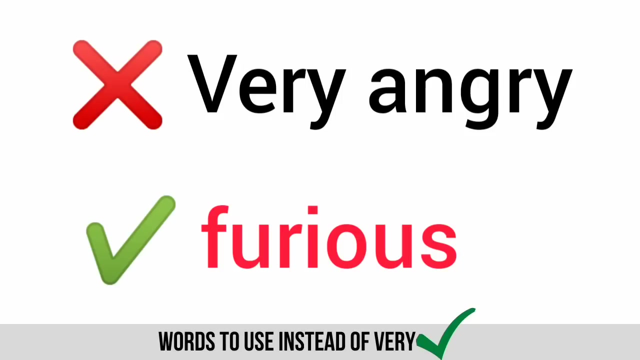 Very dull, boring, very dull, boring, very deep, profound, very deep, profound, very beautiful, gorgeous, very beautiful, gorgeous, very bright, very bright, Very bright, luminous, very bright, luminous, very accurate, exact, very accurate, exact, very afraid, terrified, very afraid, terrified, very angry, very angry, very angry. 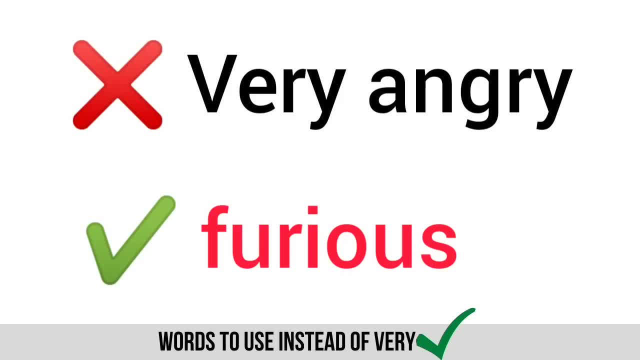 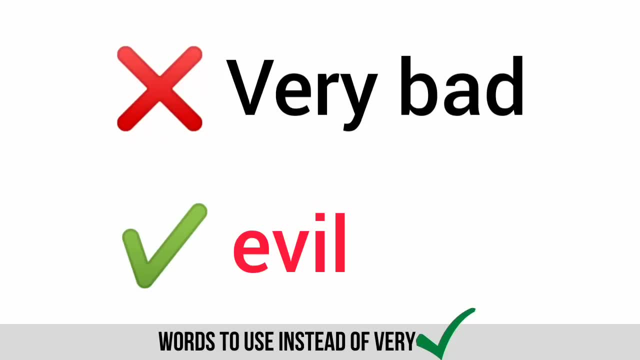 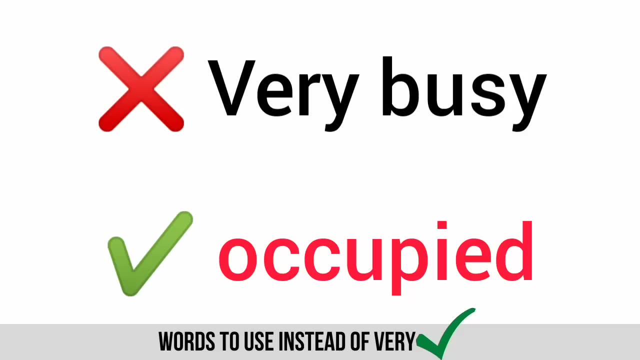 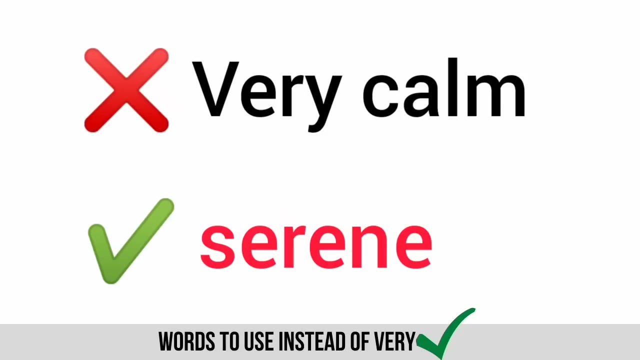 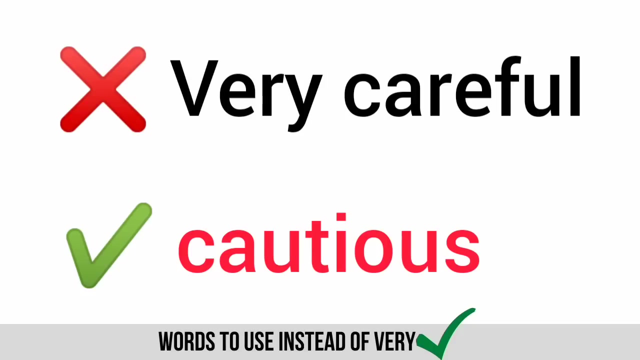 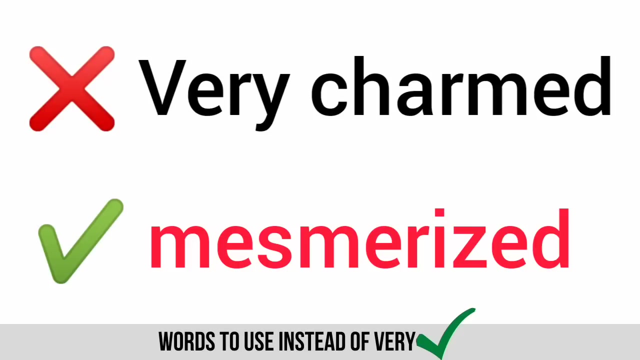 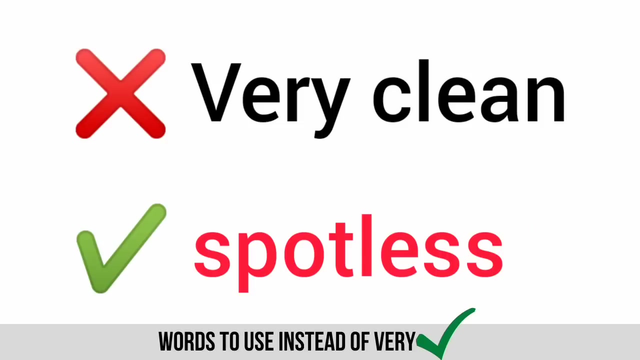 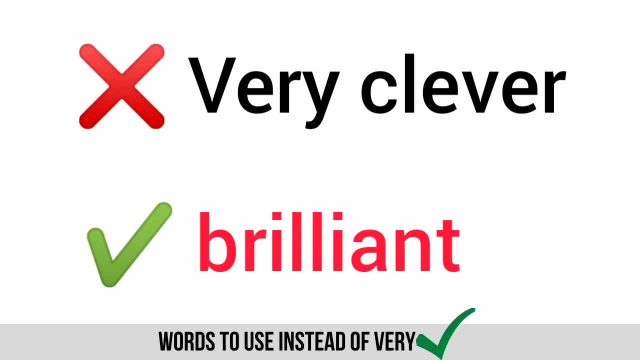 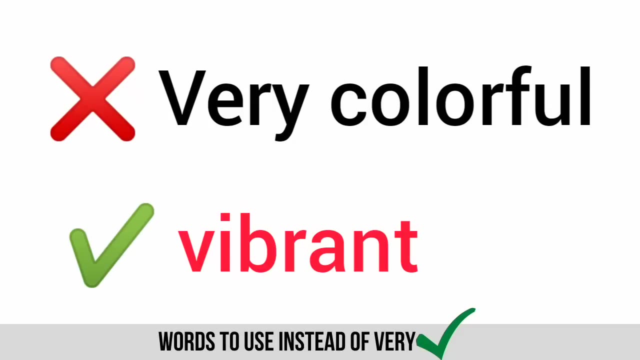 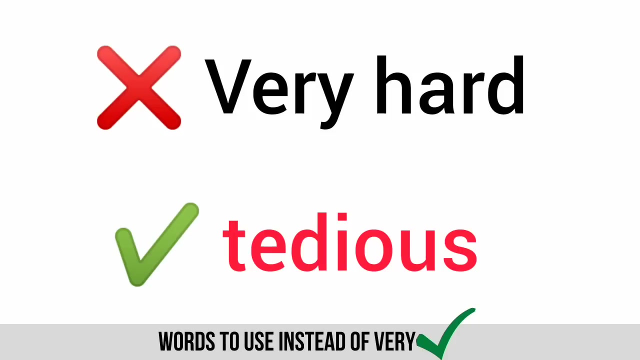 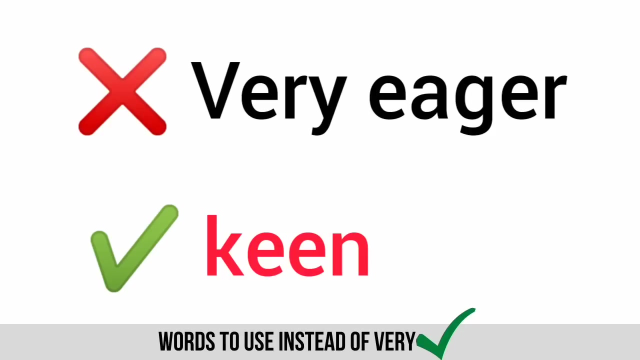 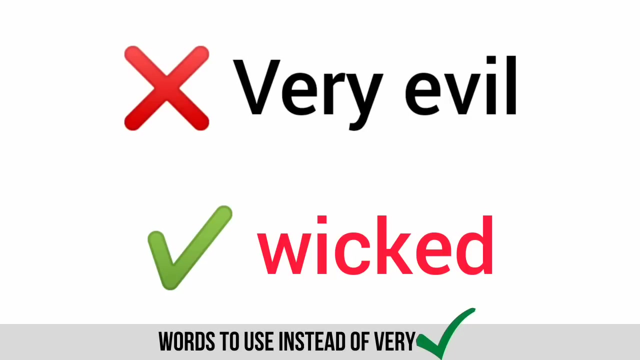 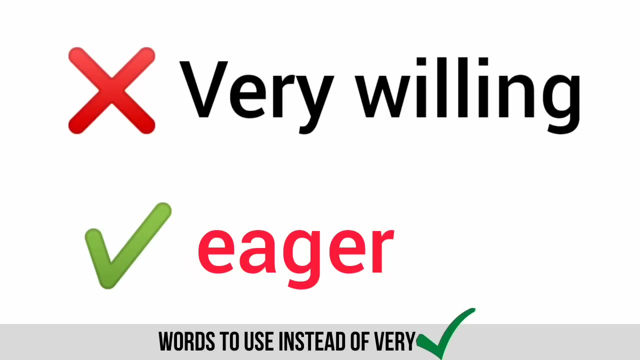 Spotless, very clever, brilliant, very clever, brilliant, very colorful, vibrant, very colorful, vibrant. Very hard, tedious, very hard, tedious, Very eager, keen, very eager, keen, very evil, wicked, very evil, wicked, very willing, eager, very willing, eager. 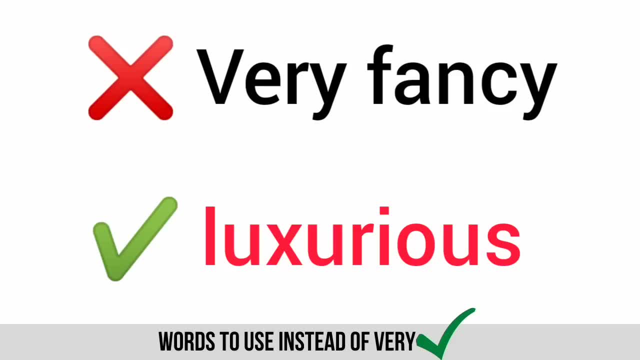 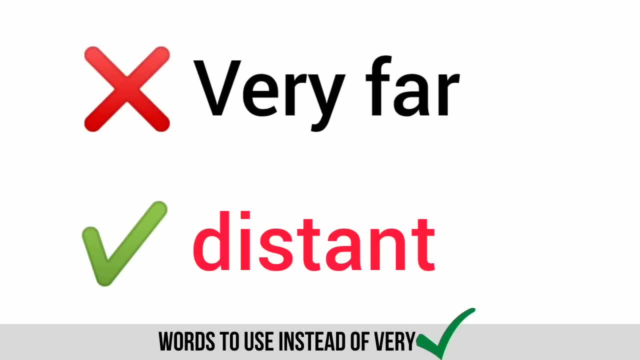 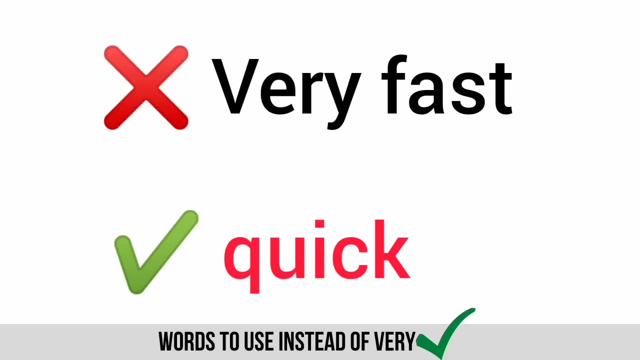 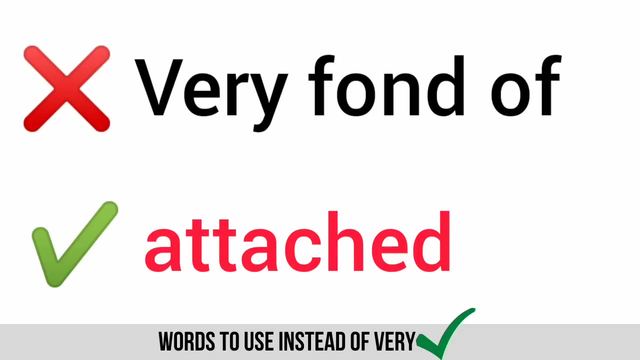 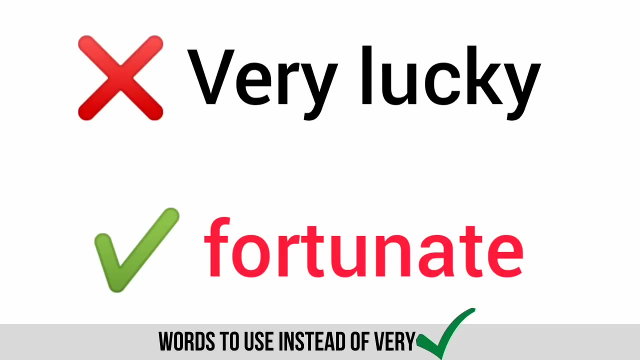 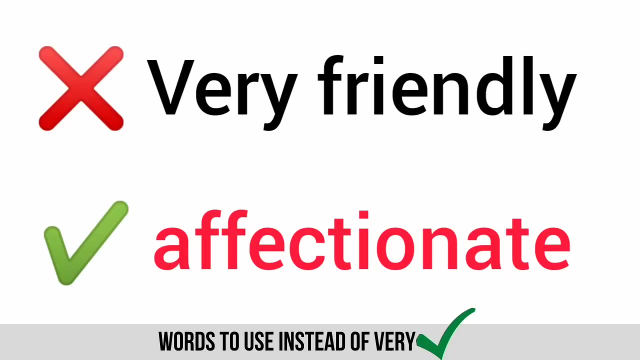 Very fancy, luxurious, Luxurious, very fancy, luxurious, very far distant, very far distant, very fast, quick, very fast, quick, very fond of attached, very fond of Attached. very lucky, fortunate, very lucky, fortunate. very friendly affectionate, very friendly affectionate. 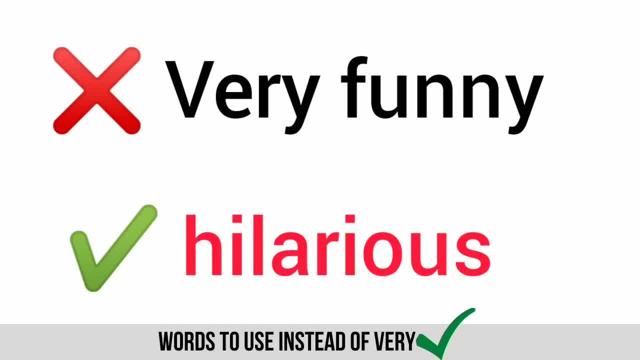 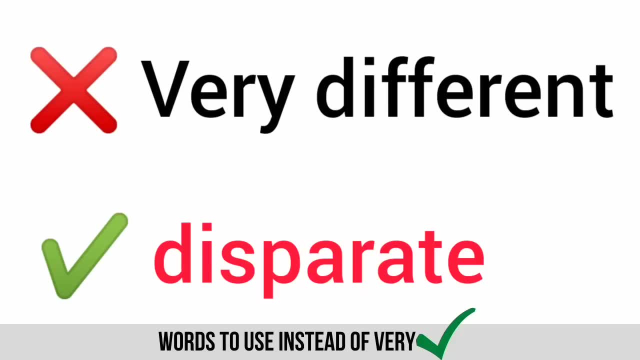 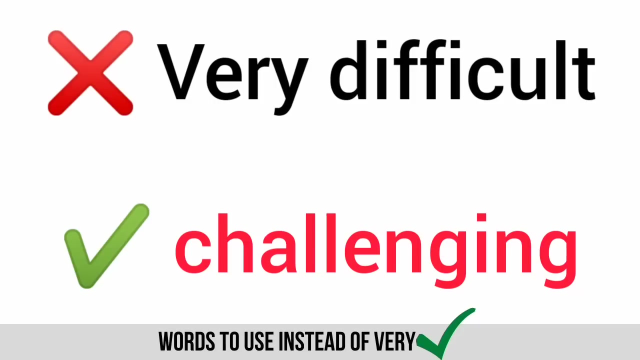 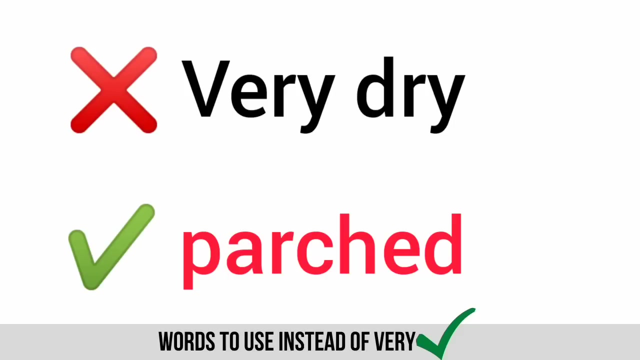 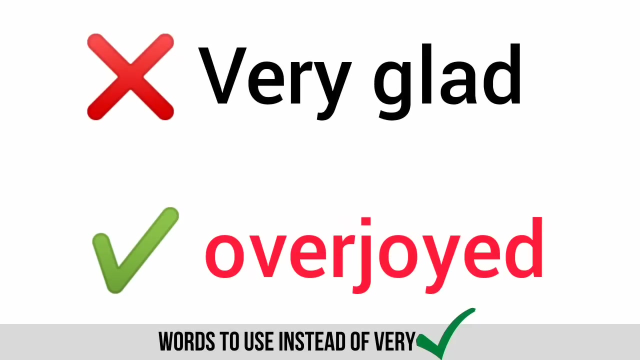 Very funny, hilarious, very funny, hilarious. Very different, disparate, very different, disparate, very difficult, challenging, very difficult, challenging, Very dry parched, very dry parched. very glad, overjoyed, Very glad overjoyed. 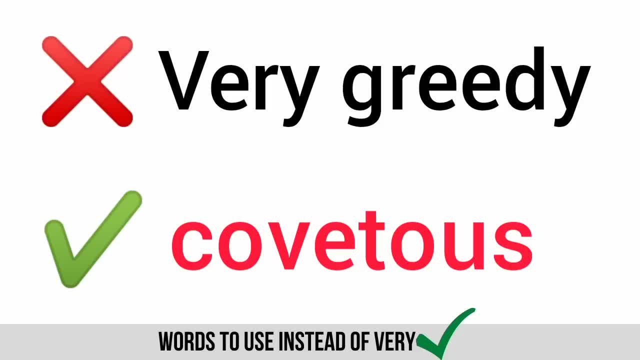 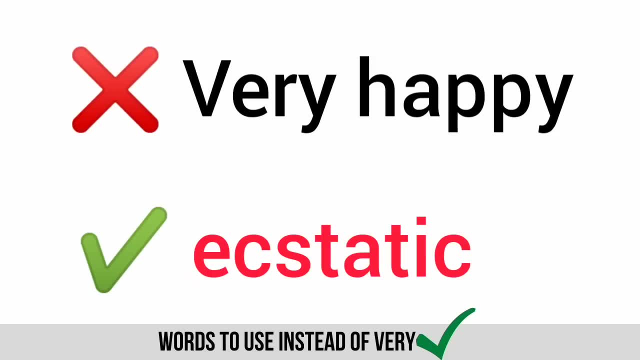 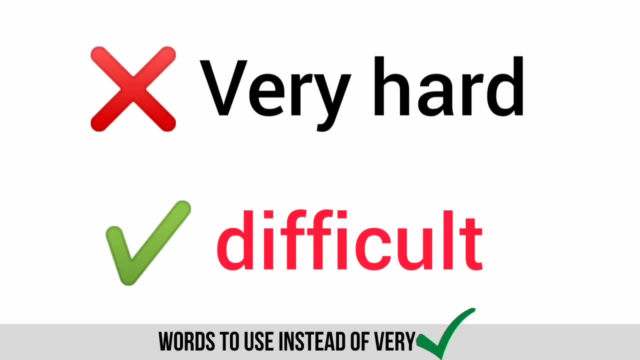 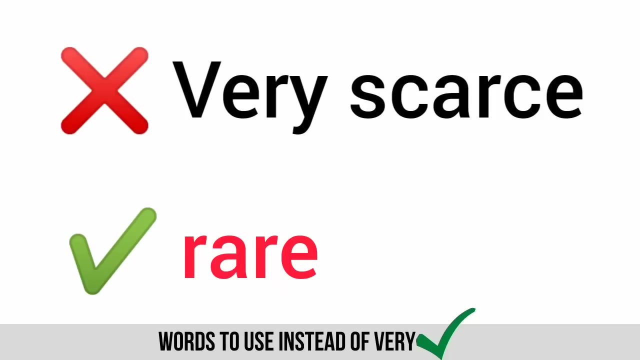 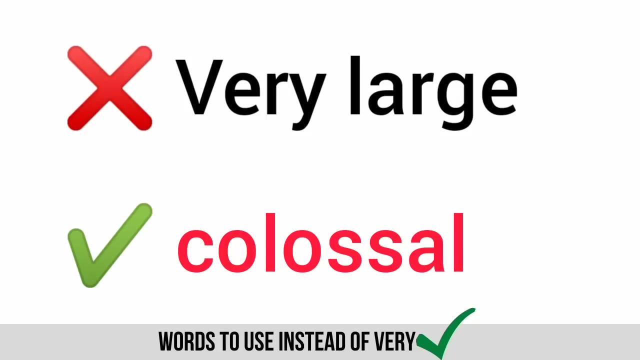 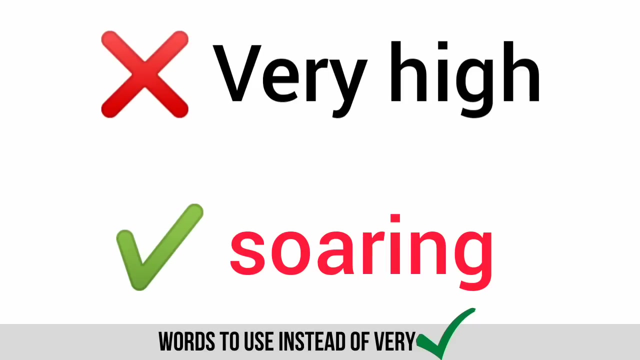 Very greedy covetous, very greedy covetous, Very happy, ecstatic, very happy, ecstatic. Very hard, difficult, very hard, Difficult, very scarce, rare, very large colossal, very high soaring, very high soaring. 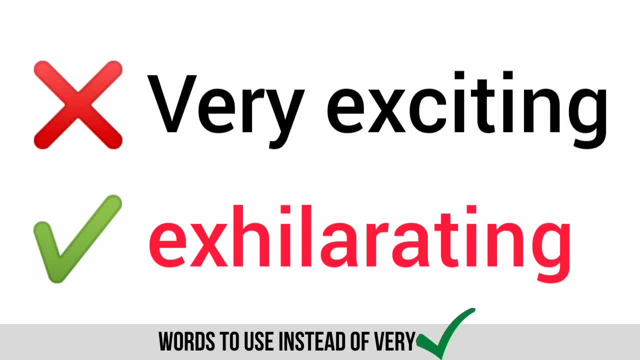 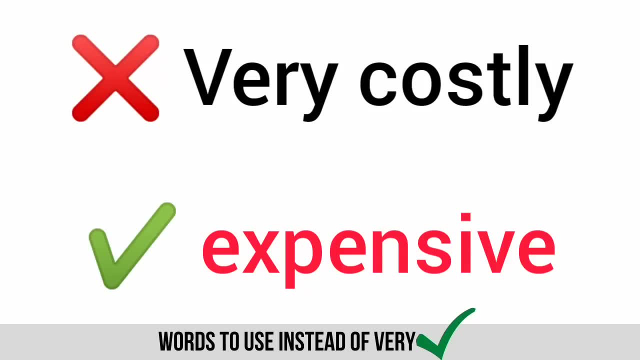 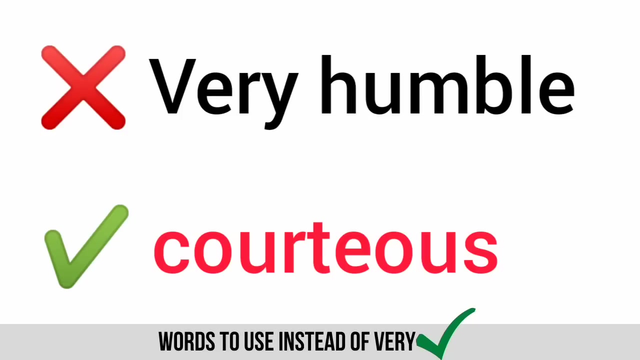 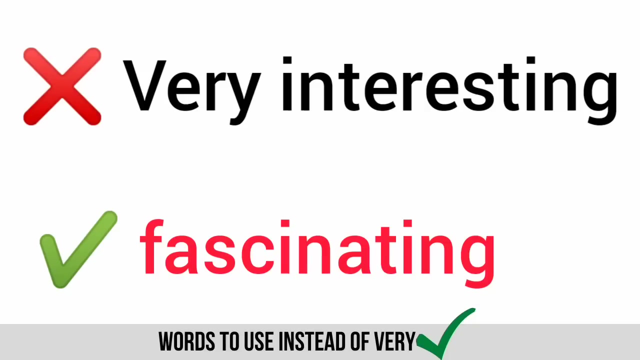 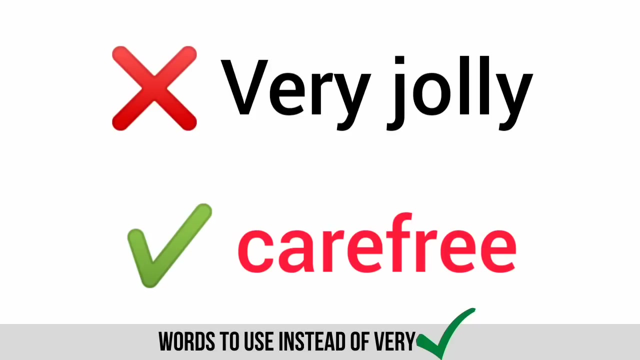 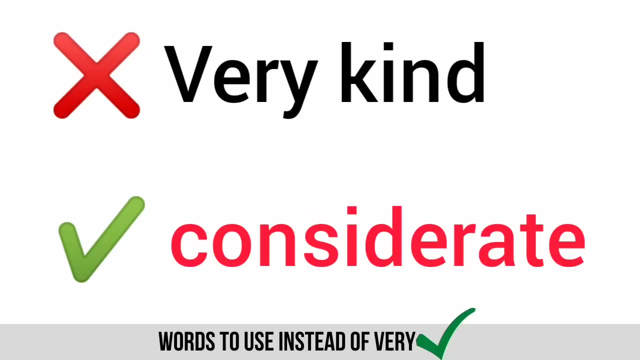 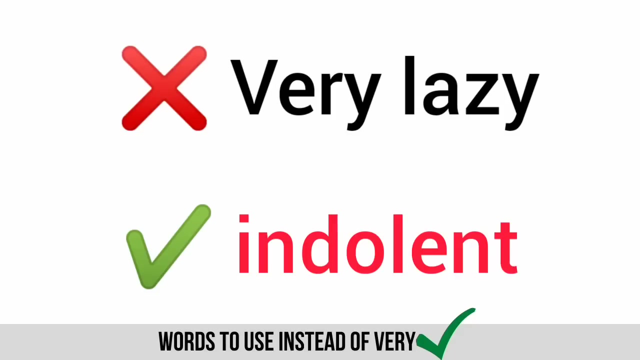 Very exciting, exhilarating, very exciting, exhilarating. very costly, expensive, very costly expensive. very humble, courteous, very humble courteous. very interesting, Fascinating, very interesting, fascinating, very jolly carefree, very jolly carefree. very kind, considerate very kind, considerate very lazy, indolent. 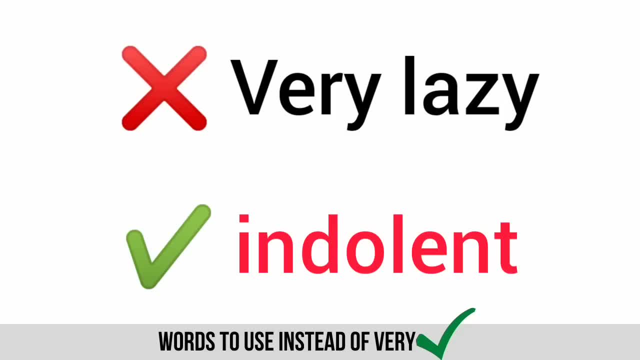 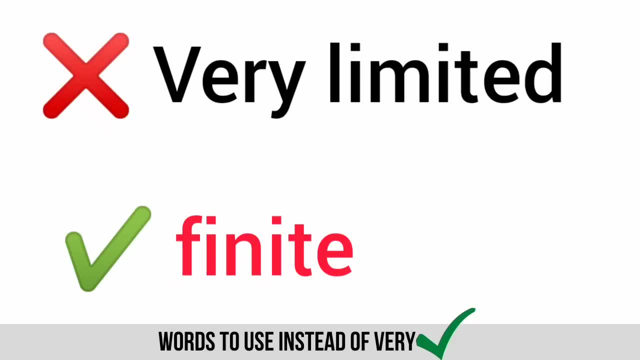 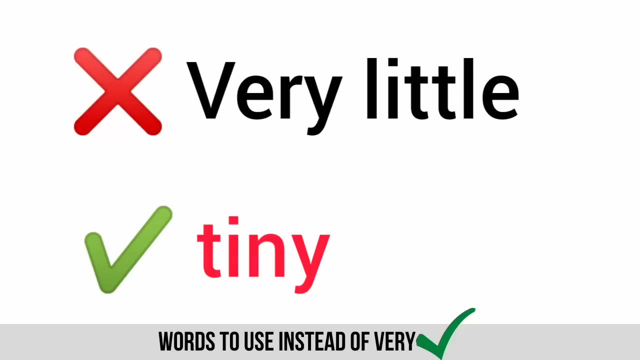 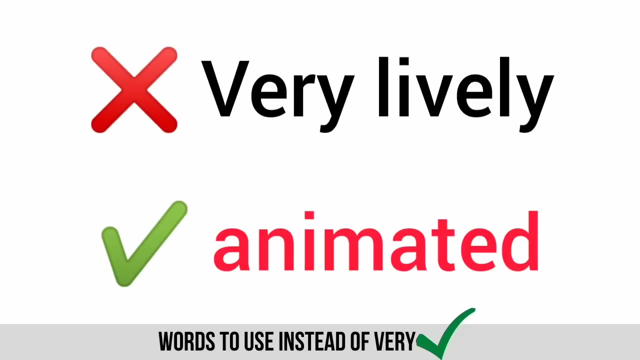 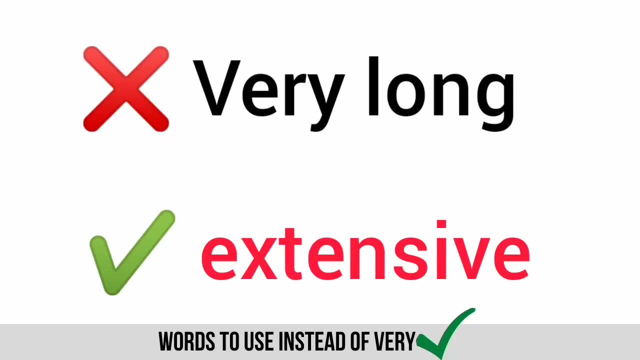 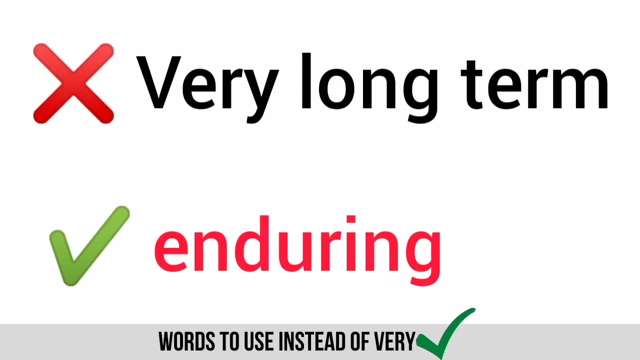 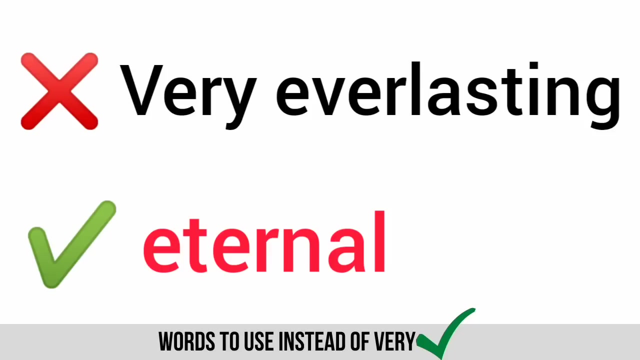 very lazy, indolent, very limited, finite, very limited, finite, very little, tiny, very little tiny, very lively, animated, animated, very lively, Animated. very long, extensive, very long, extensive, very long-term, enduring, very long-term, enduring very everlasting, eternal, very everlasting. 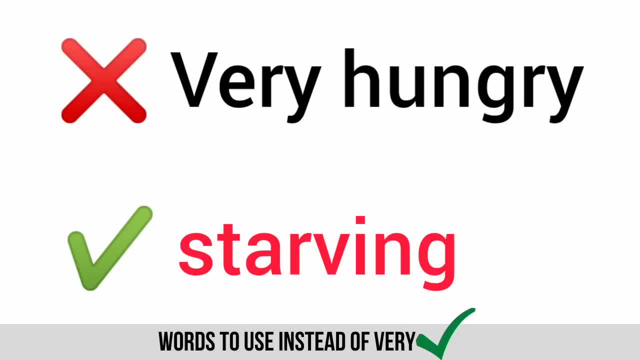 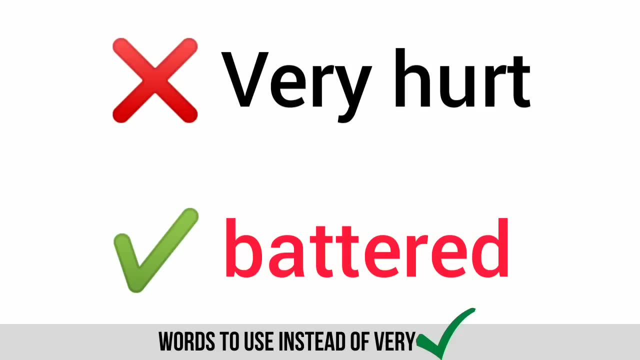 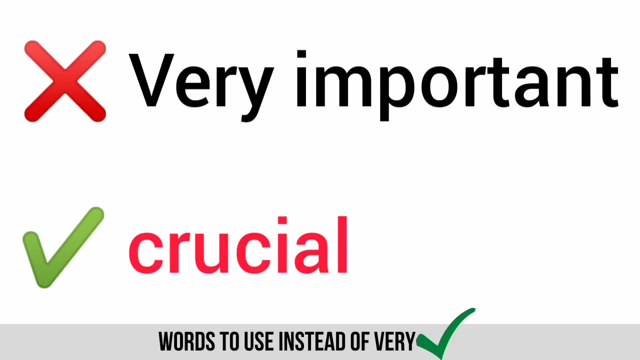 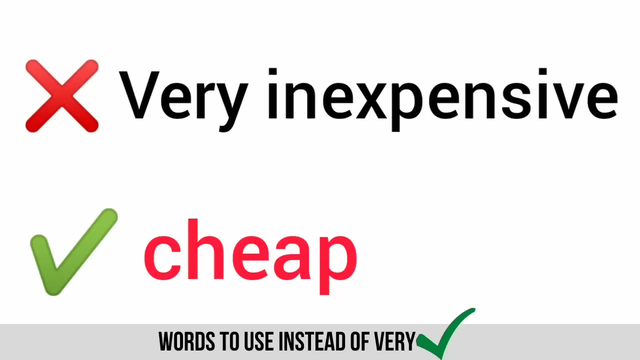 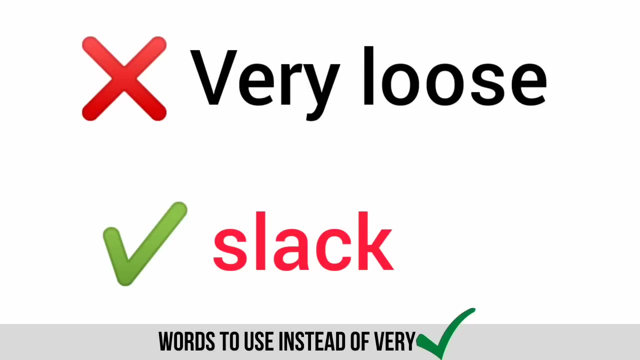 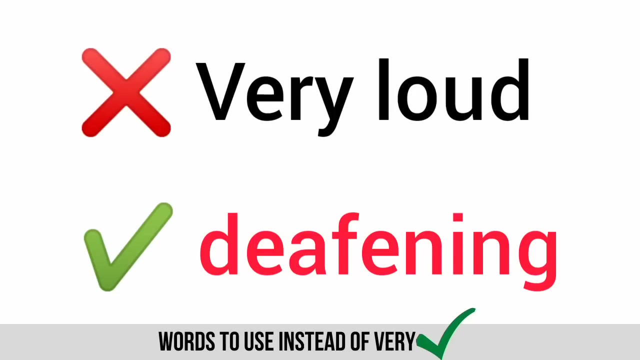 Eternal: very hungry, starving, very hungry, starving, very hot battered, very hot battered. very important, crucial, very important, crucial. Very inexpensive, cheap, very inexpensive, cheap. very loose slack, very loose slack, very loud, deafening, very loud, deafening. 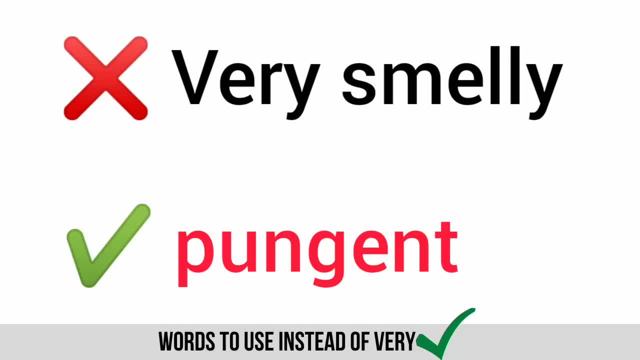 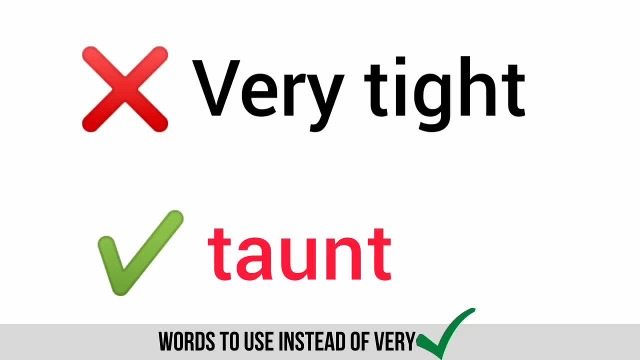 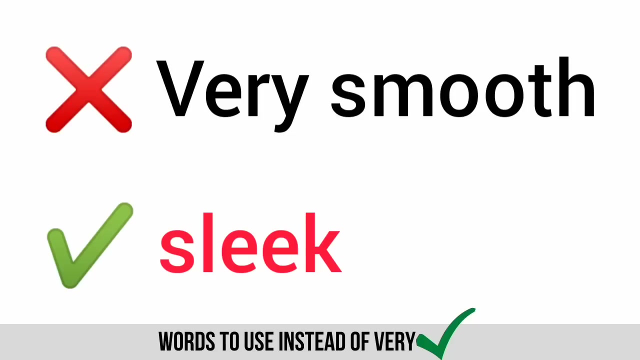 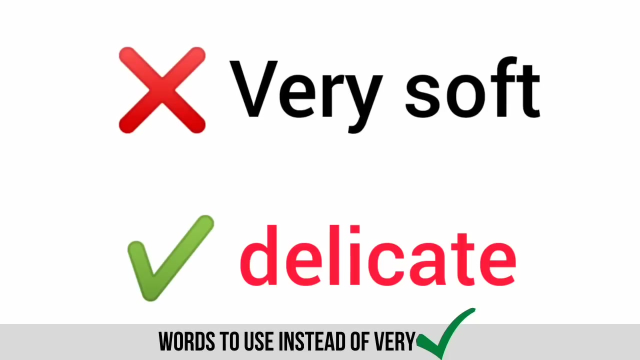 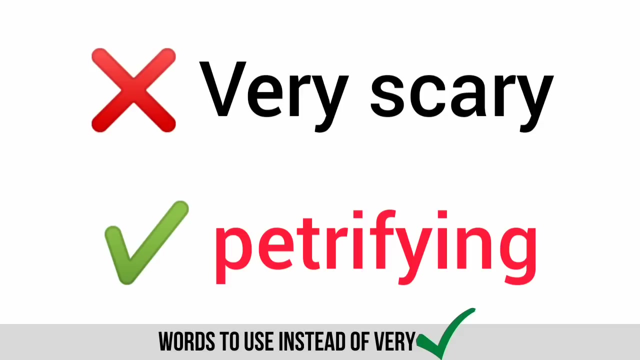 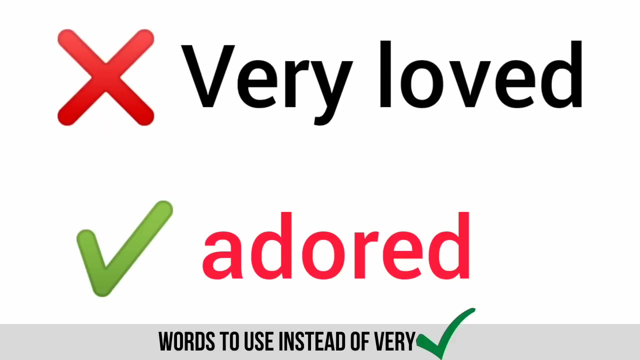 Very smelly pungent, very smelly pungent. very tight taunt, very tight taunt, very smooth, sleek, very smooth, sleek, very soft, Delicate, very soft, delicate, very scary, petrifying, very scary, petrifying. very loved, adored, very loved, adored. 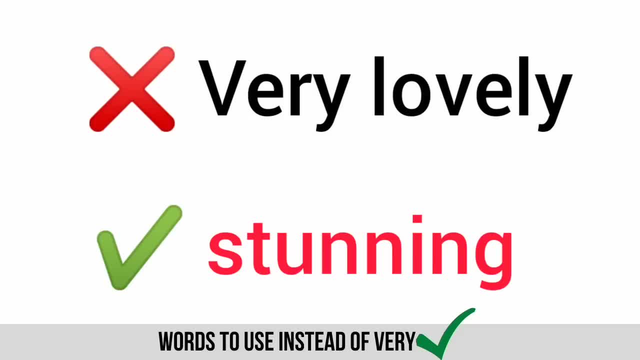 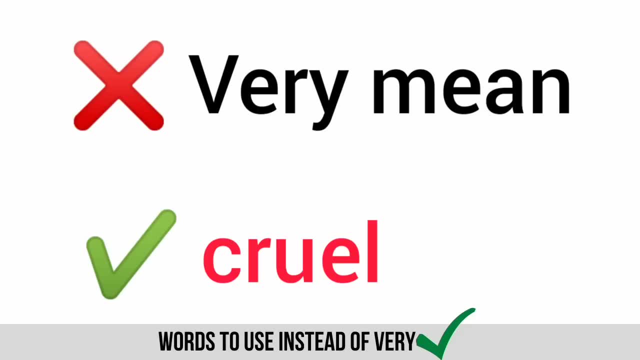 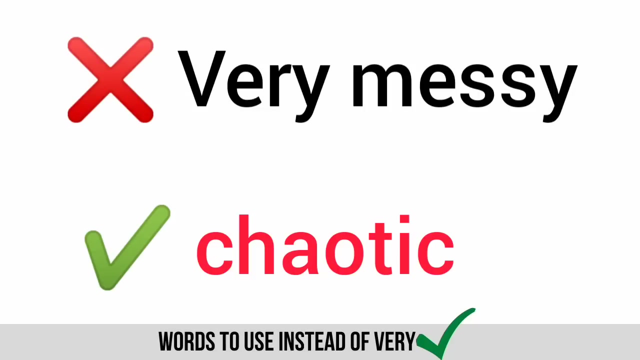 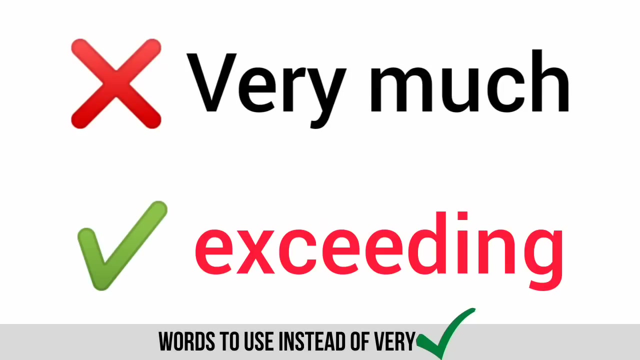 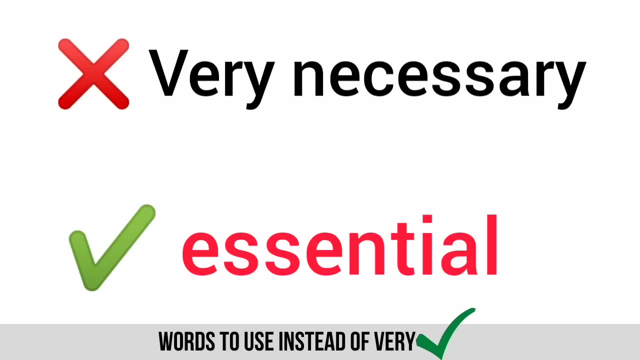 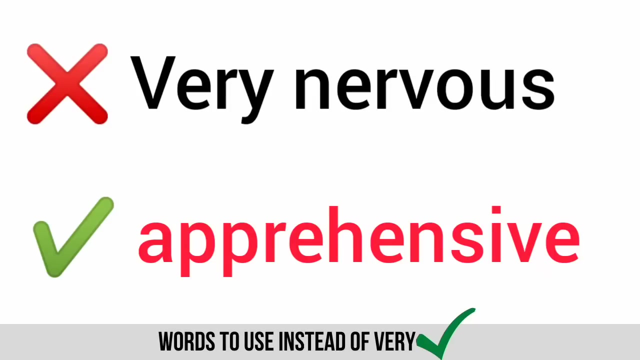 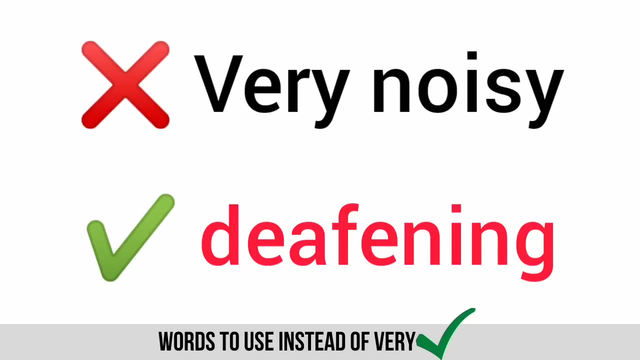 Very lovely, Stunning, very lovely, stunning, very mean, cruel, very mean cruel, Very messy, chaotic, very messy, chaotic, very much exceeding, very much Exceeding, very necessary, essential, very necessary, essential, very nervous, apprehensive, very nervous, apprehensive, very noisy, deafening, very noisy. 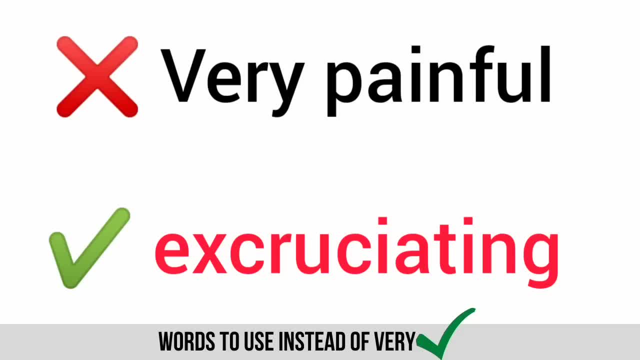 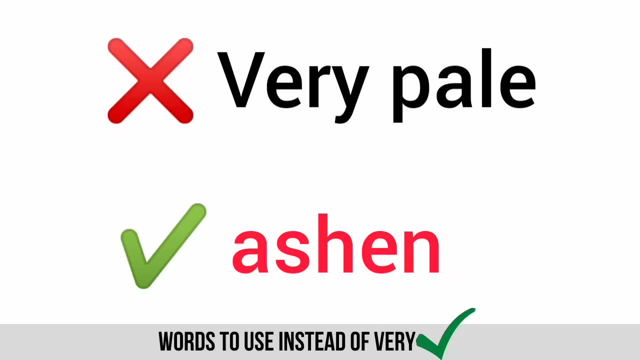 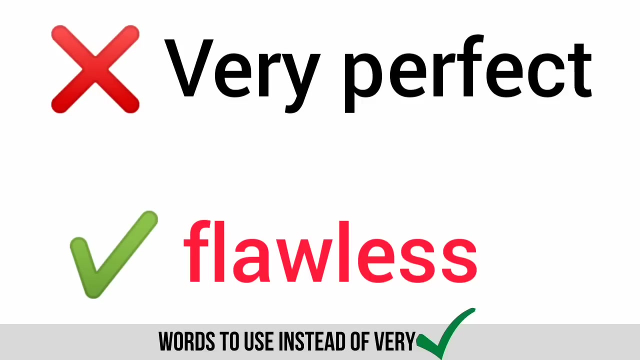 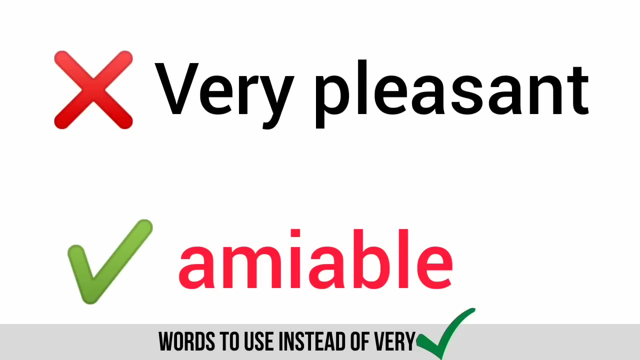 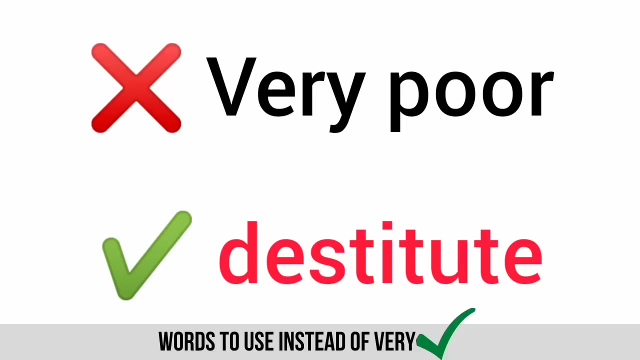 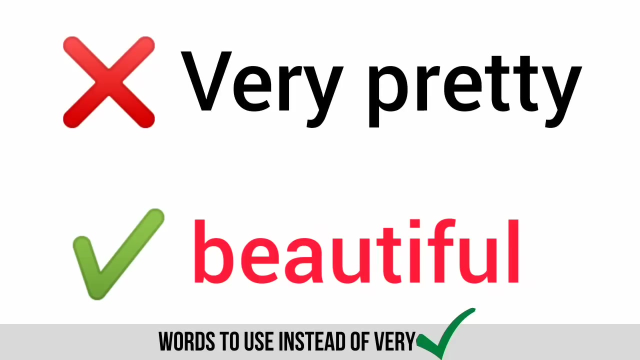 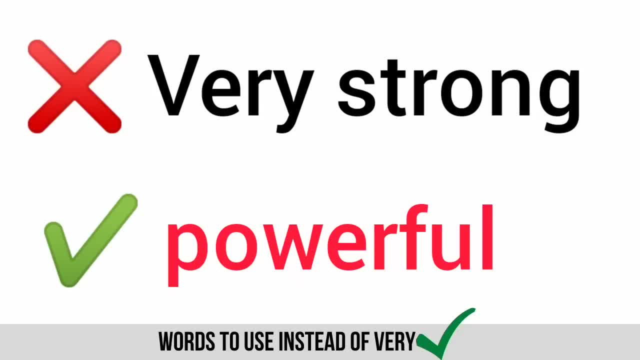 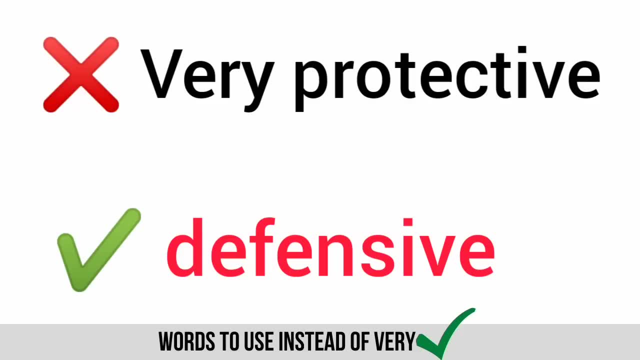 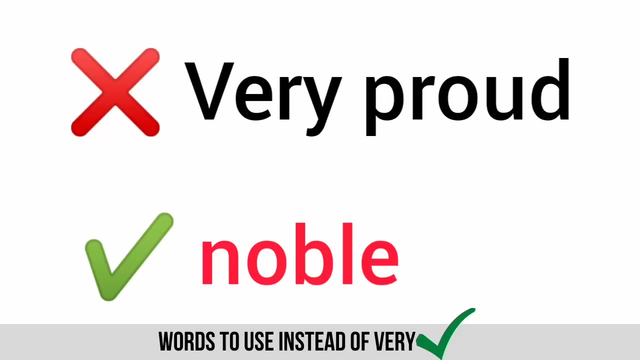 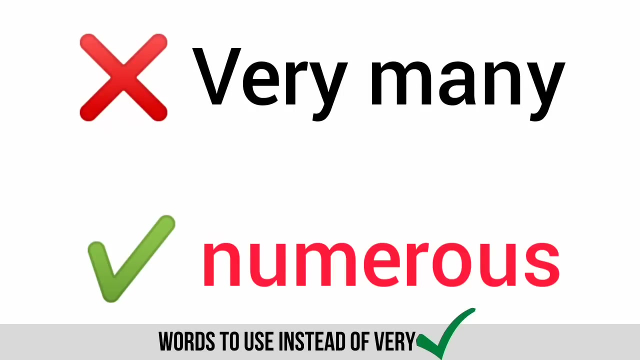 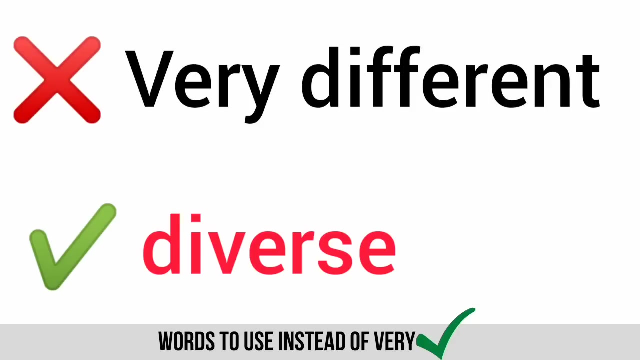 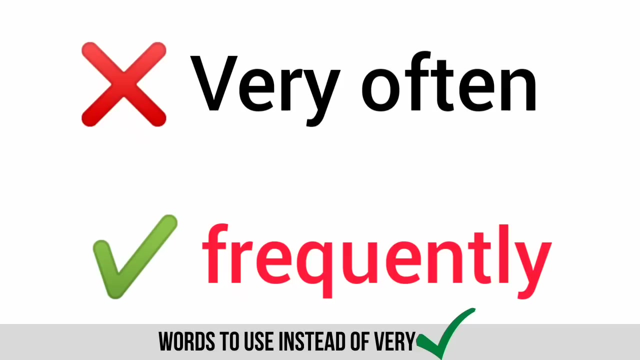 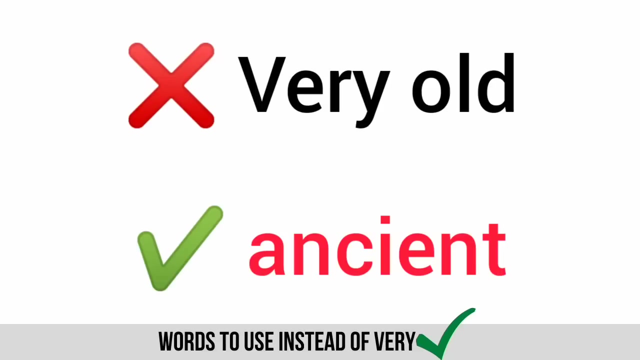 very strong, powerful, very strong, powerful, very protective defensive, very protective defensive, very proud, noble, very proud noble. very many, numerous, very many, numerous, very different, diverse, very different, Diverse. very often, frequently, very often frequently, very old, ancient, very old ancient. 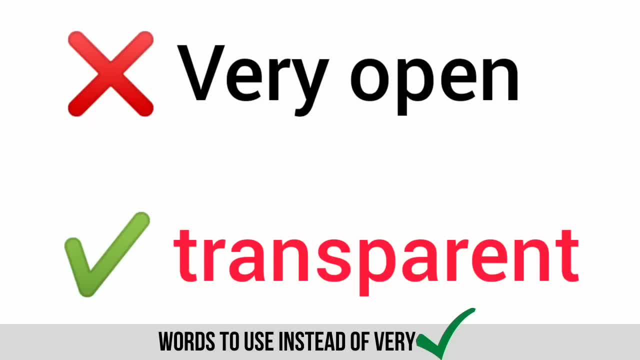 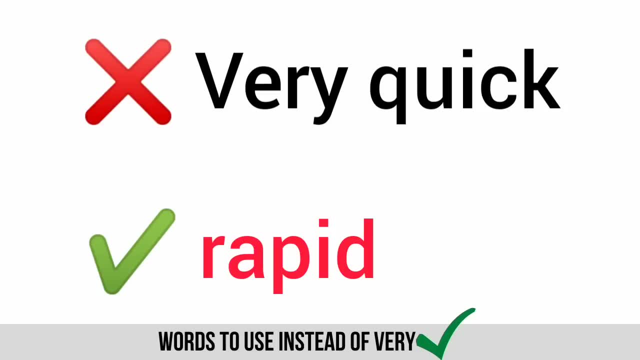 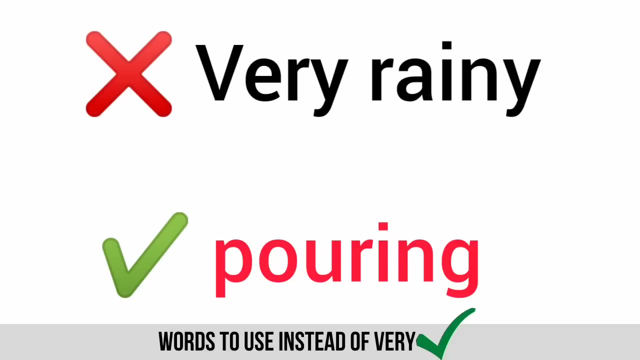 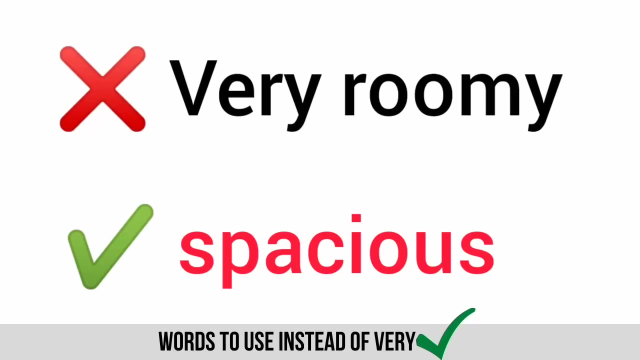 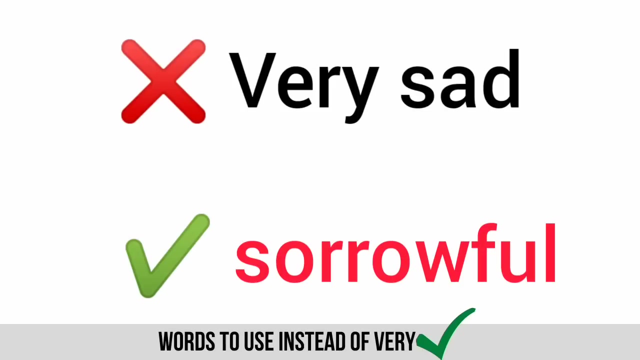 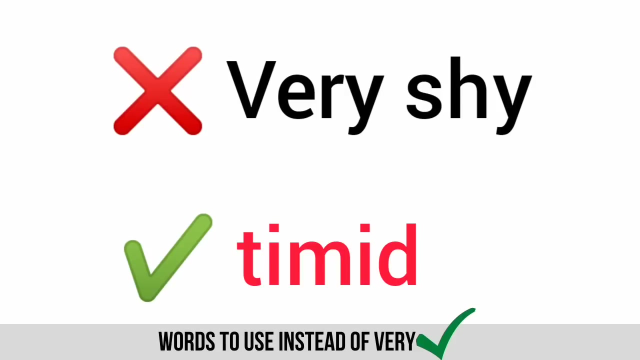 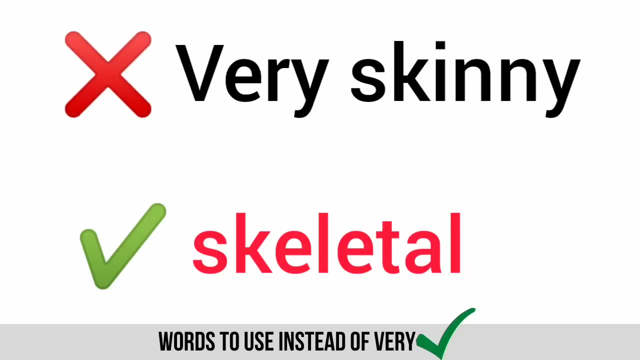 very open, transparent, very open transparent, Very quick, rapid, very quick rapid. very rainy pouring, very rainy pouring. very roomy spacious, very roomy spacious. very sad, Sorrowful, very sad, sorrowful, very shy, timid, very shy, timid. very skinny, skeletal. 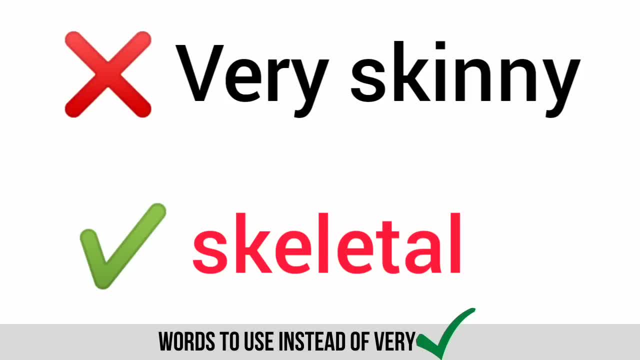 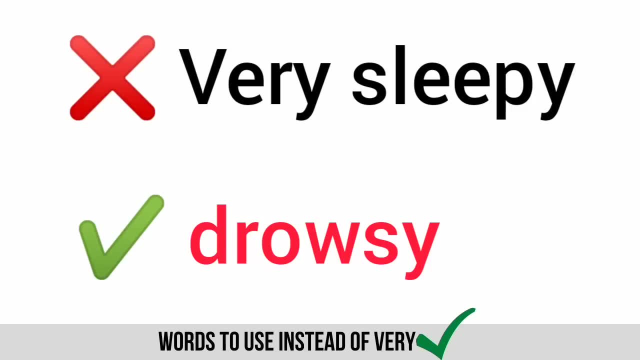 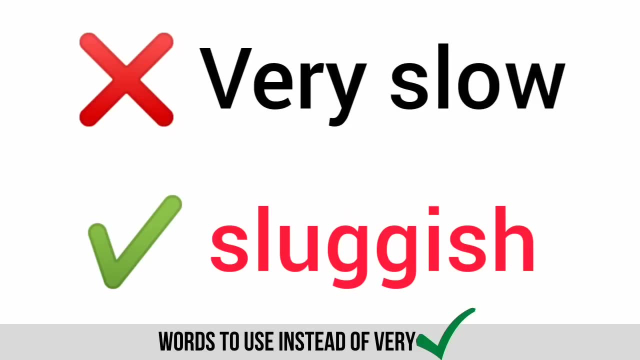 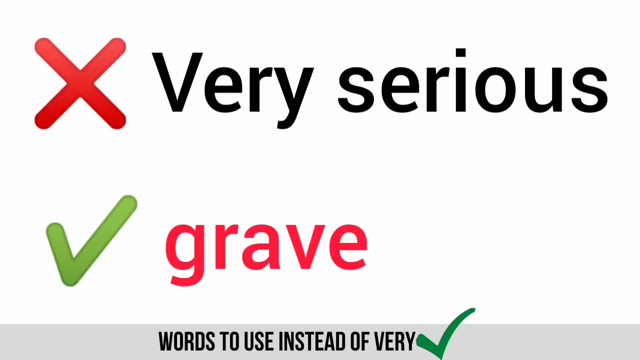 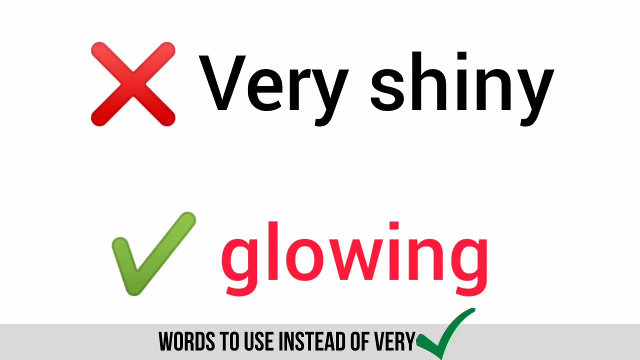 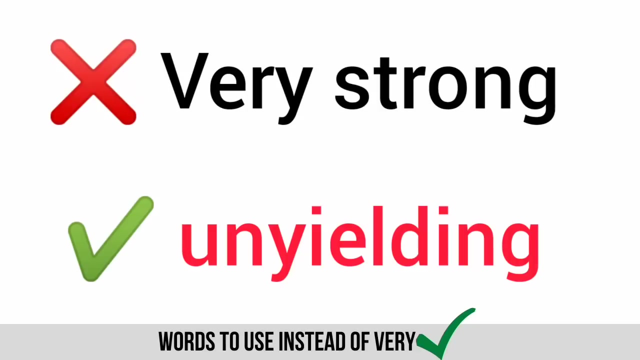 very skinny, skeletal, very sleepy, drowsy, Very slow, sluggish, very slow, sluggish. Very serious grave, very serious grave. Very shiny, glowing, very shiny, Very strong, unyielding, Very strong, unyielding. 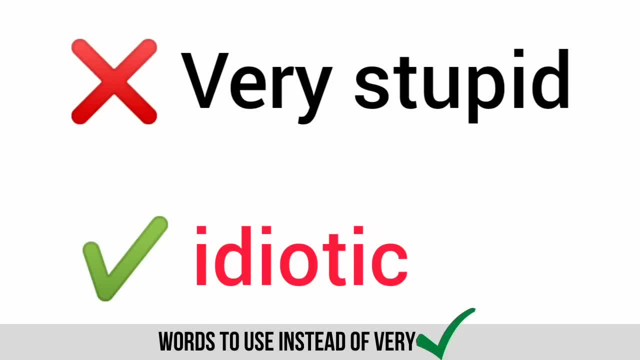 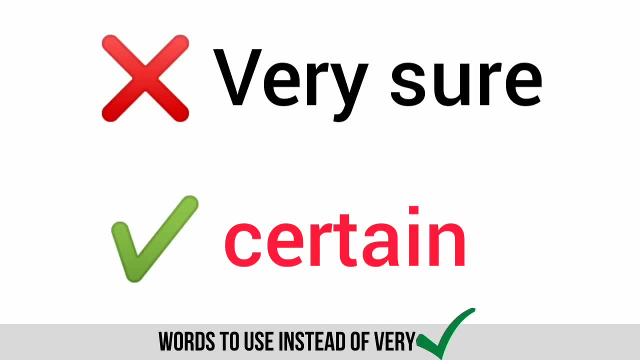 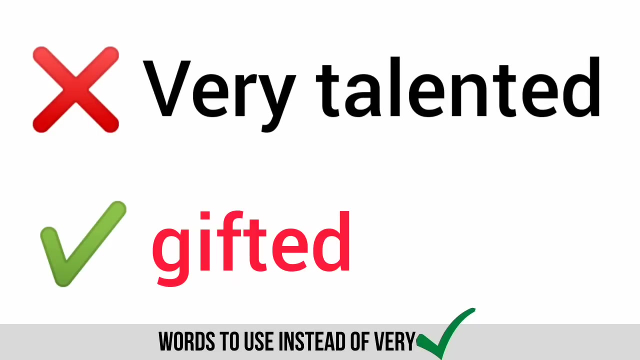 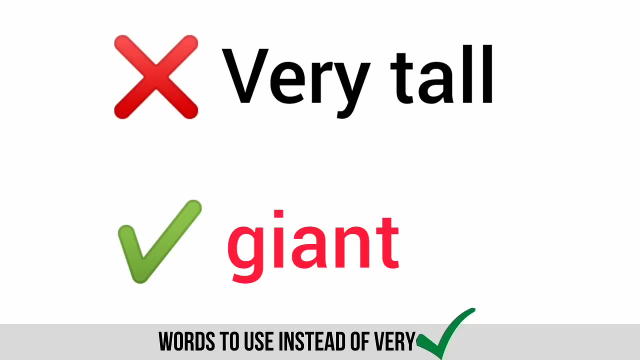 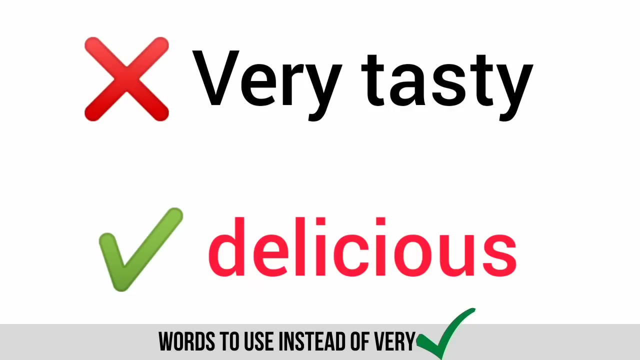 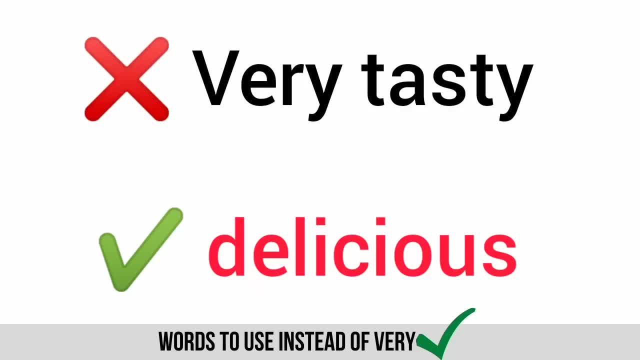 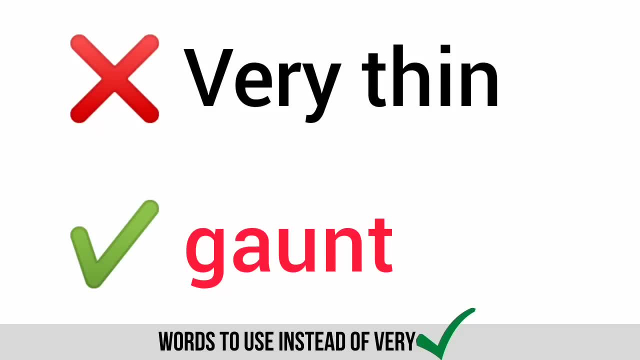 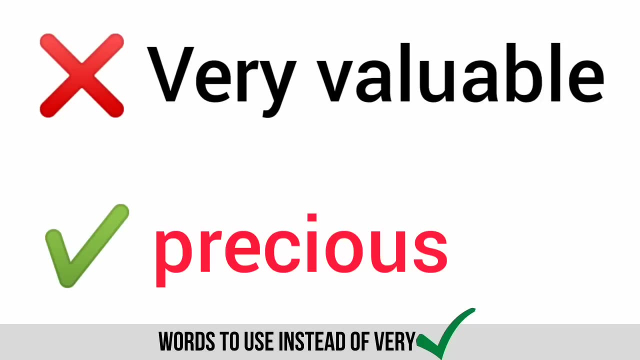 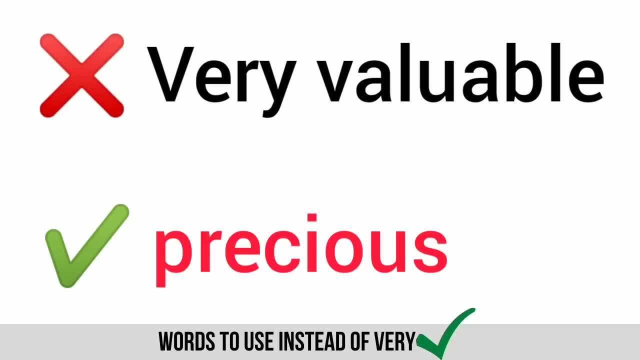 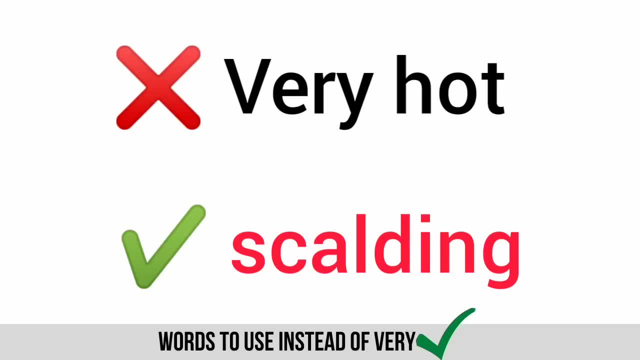 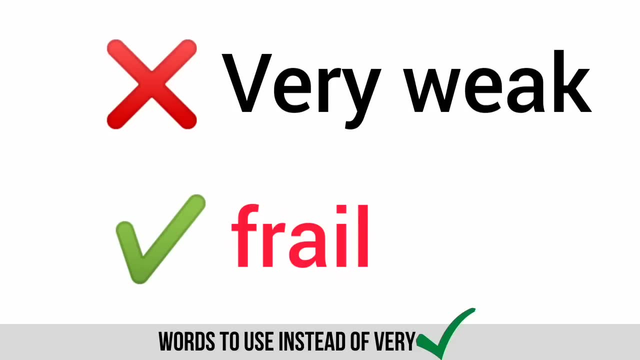 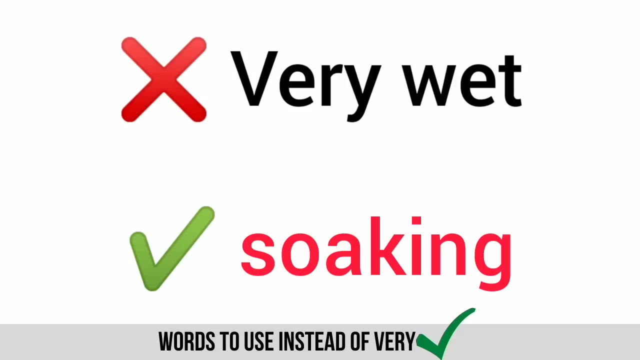 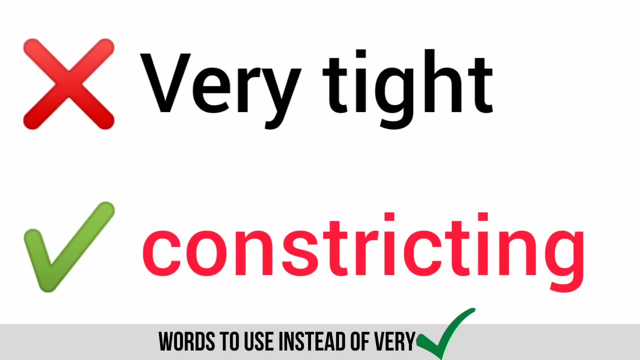 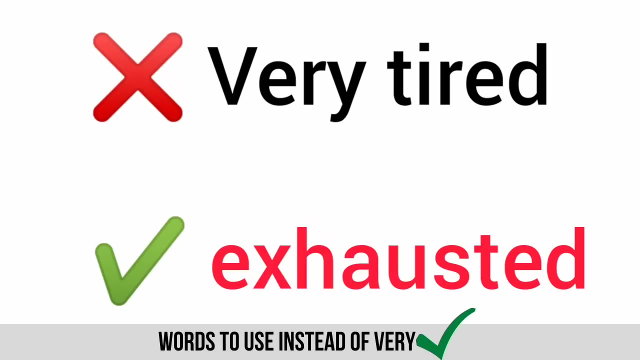 very valuable, precious, very hot scalding, very hot scalding very weak frail, very weak frail, very wet, soaking, very wet, Soaking, very tight constricting, very tight constricting, very tired, exhausted, very. 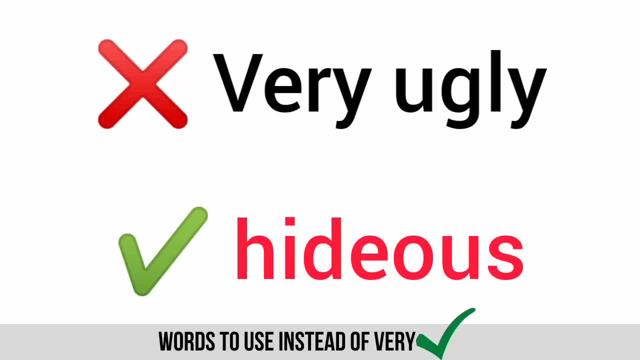 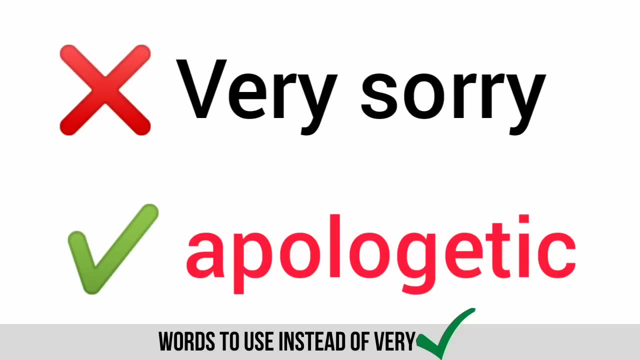 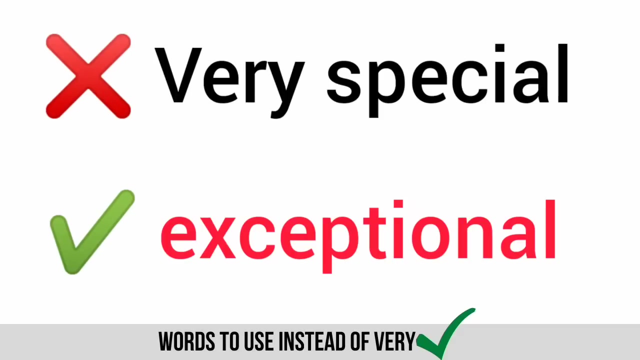 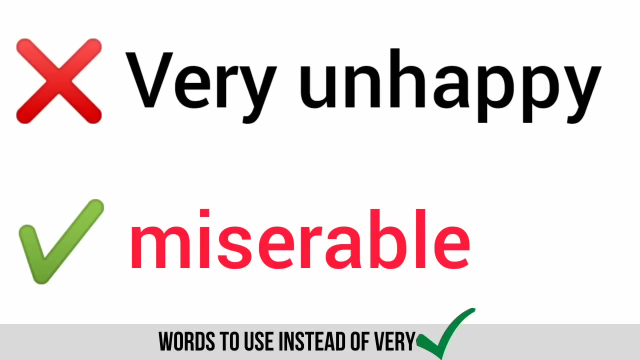 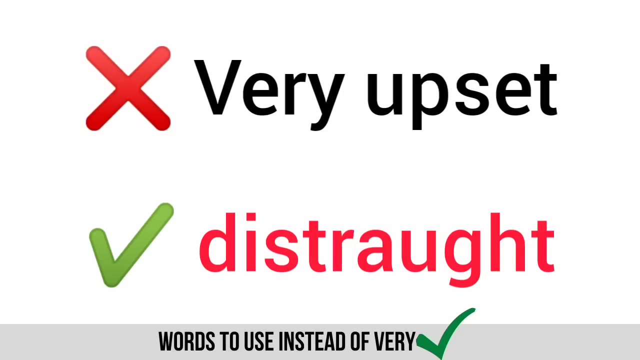 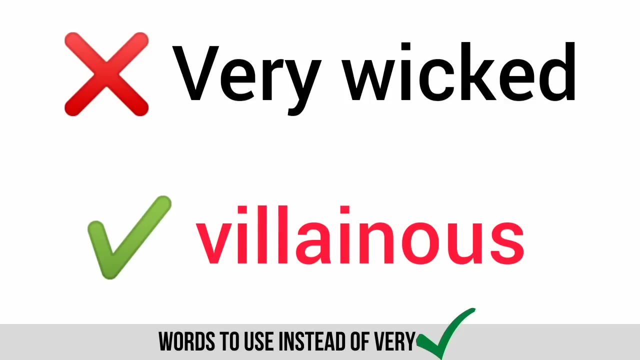 tired, exhausted, very ugly, hideous, very ugly, Hideous, very sorry, apologetic, very sorry, apologetic. very special, exceptional, very special, exceptional, very unhappy, miserable, very unhappy, Miserable, very upset, distraught, very upset, distraught. very wicked, villainous, very. 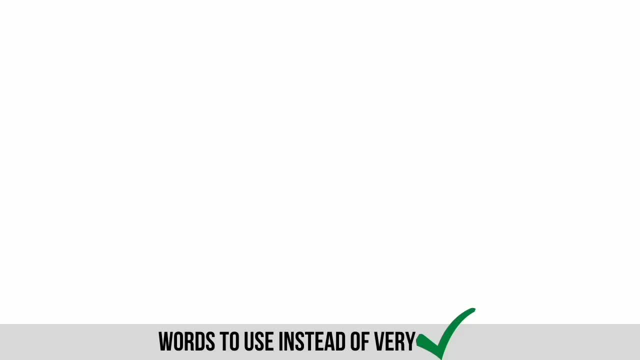 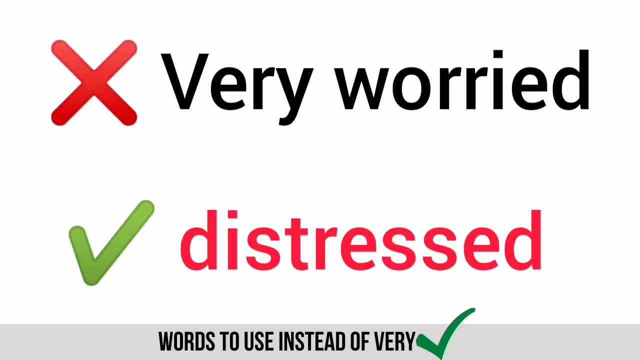 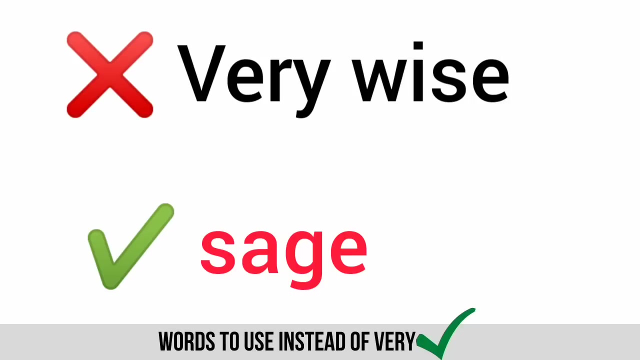 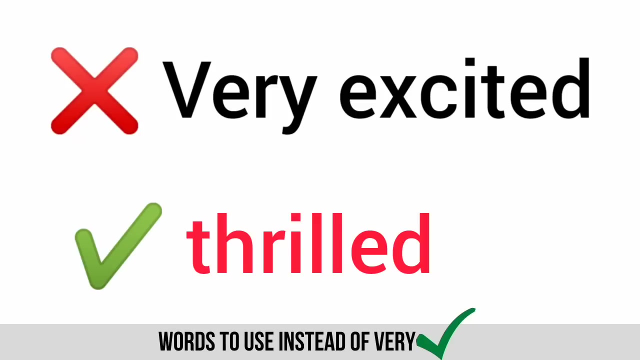 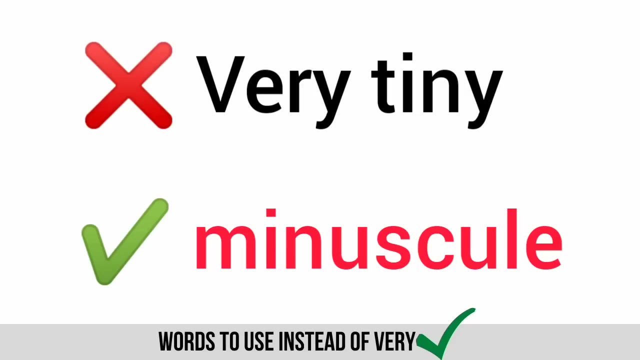 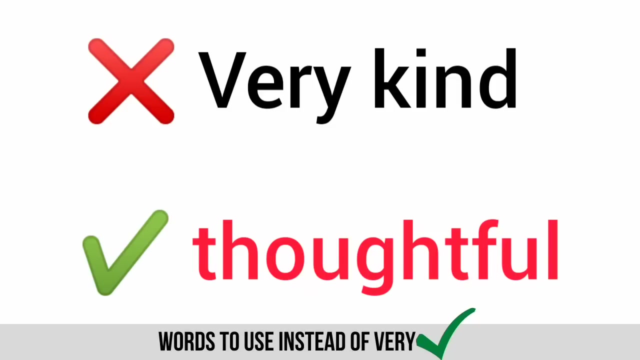 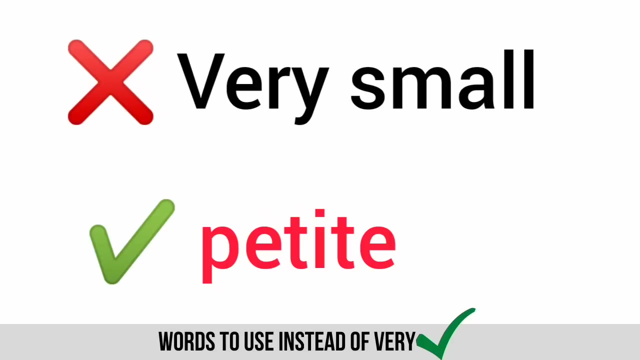 wicked, villainous, very worried, distressed, very worried, Distressed. very wise sage, very wise sage, very excited, thrilled, very excited, thrilled. very tiny miniscule, very tiny Miniscule, very kind, thoughtful, very kind, thoughtful. very small, petite, very small. petite, very scary, chilling, very scary, chilling, very quiet, Hushed, very quiet, hushed, very great, terrific, very great terrific. very fat, obese, very fat obese, very difficult, arduous. 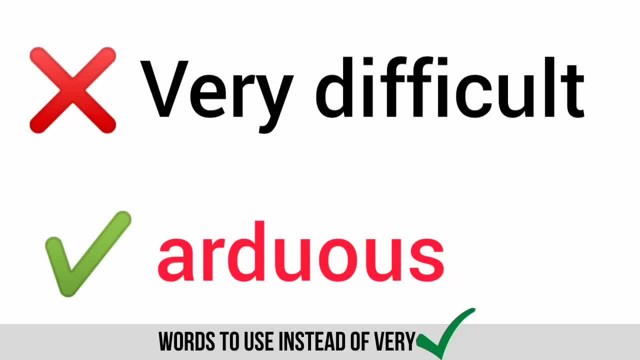 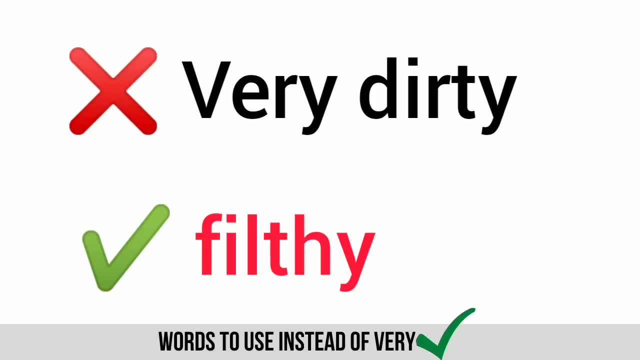 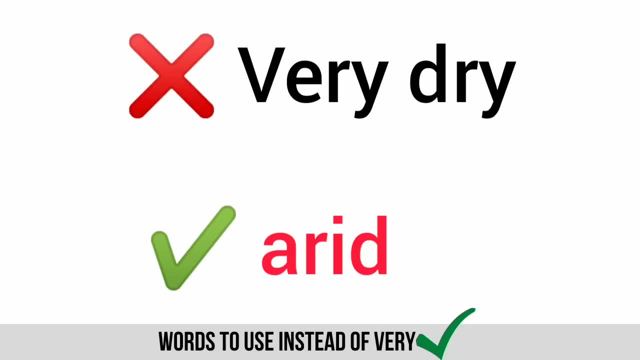 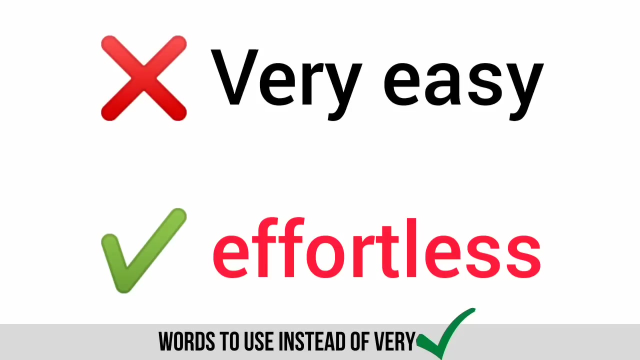 Hushed, very sweet, beautiful, very sweet, beautiful, very, very tutte. Very dirty, Filthy, Very dirty Filthy, Very dry, Arid, Very dry, Arid, Very easy, Effortless, Very weak. 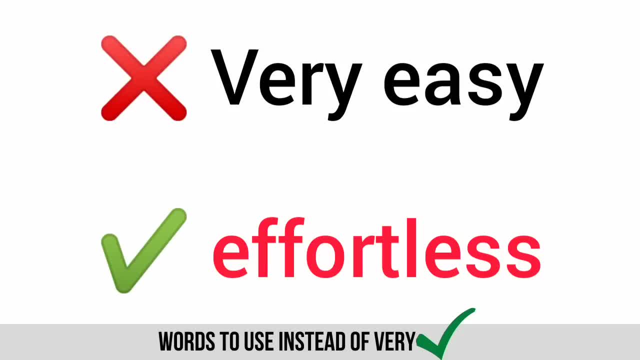 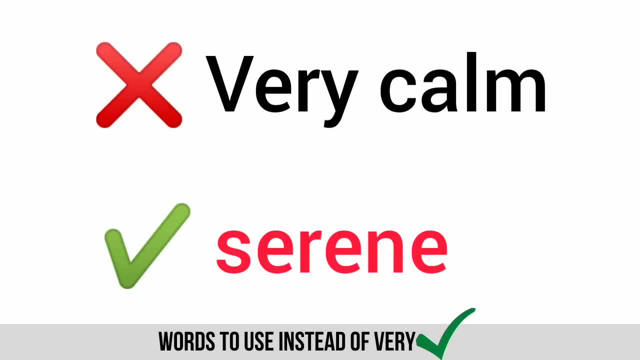 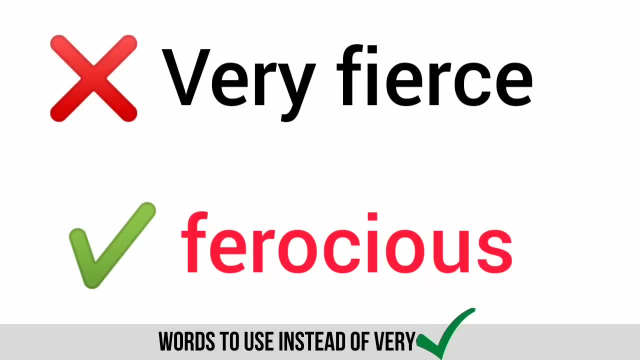 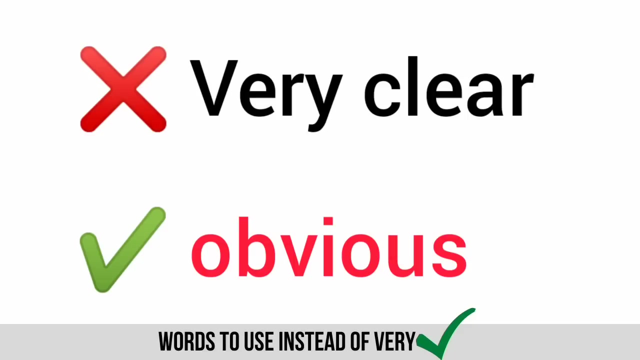 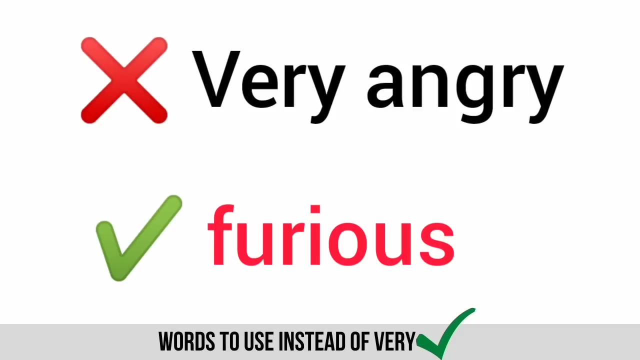 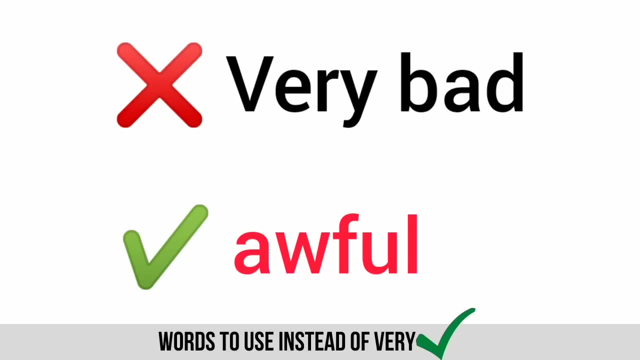 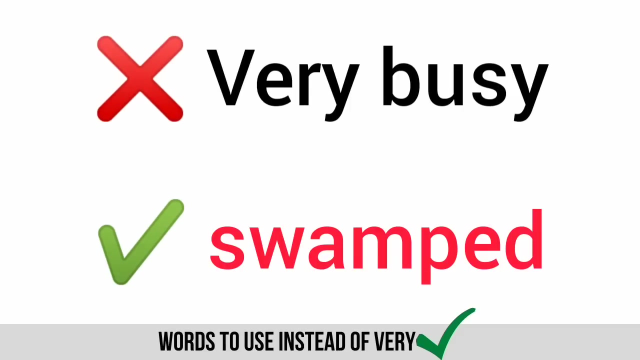 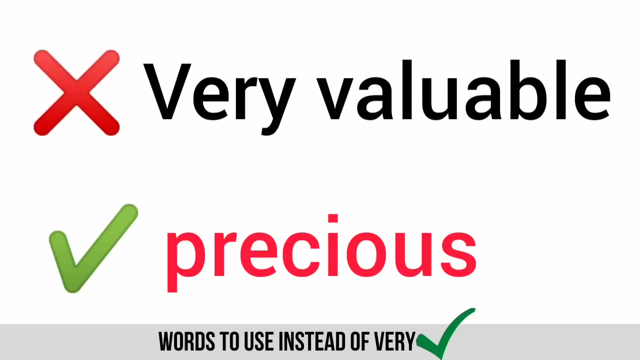 very easy, effortless, very calm, serene, very calm, serene, very fierce, ferocious, very fierce, ferocious. very clear, obvious, very clear, obvious. very angry, furious, very angry, furious, very bad, Awful, very bad, awful, very busy, swamped, very busy swamped. very valuable, precious 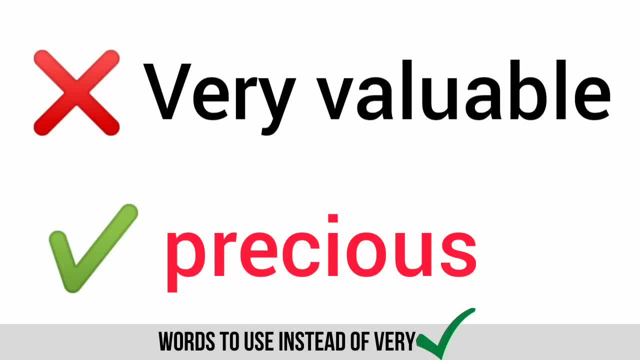 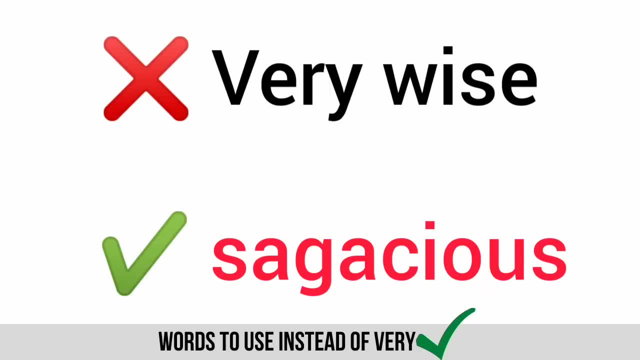 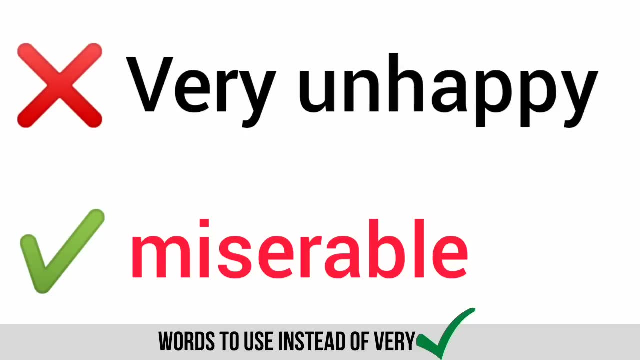 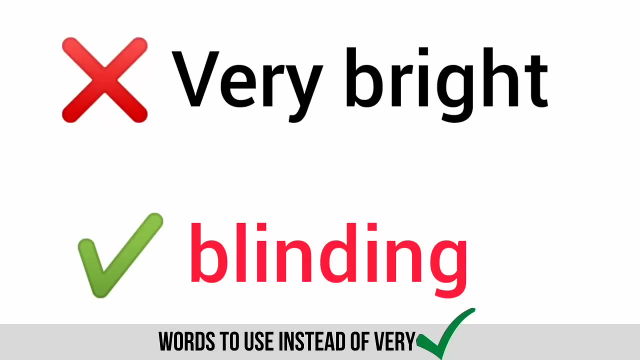 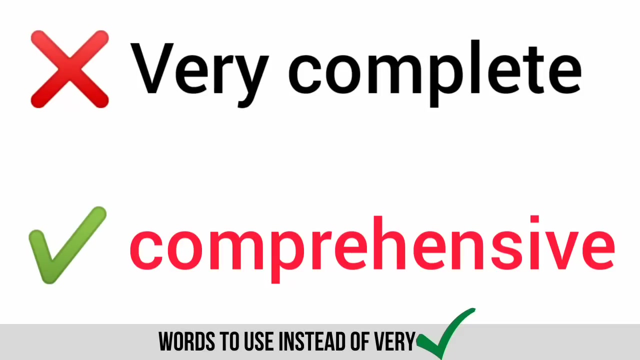 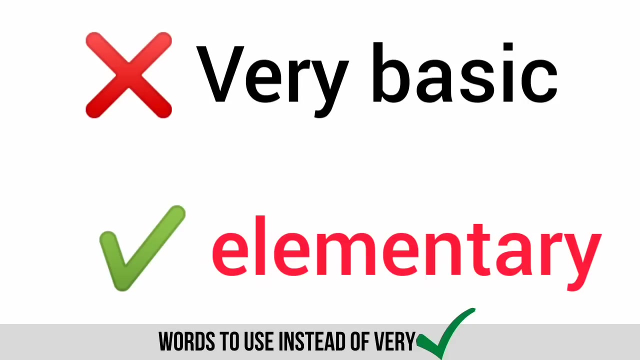 very valuable, precious, very wise, Sagacious, very wise, sagacious, very unhappy, miserable, very unhappy, miserable, very bright, blinding, very bright, blinding. very complete, Comprehensive, very complete, comprehensive, very basic, elementary, very basic elementary. 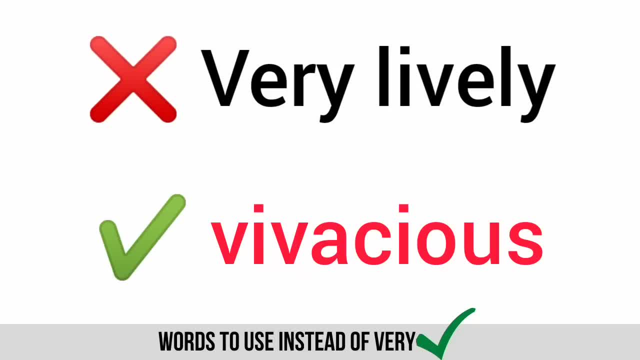 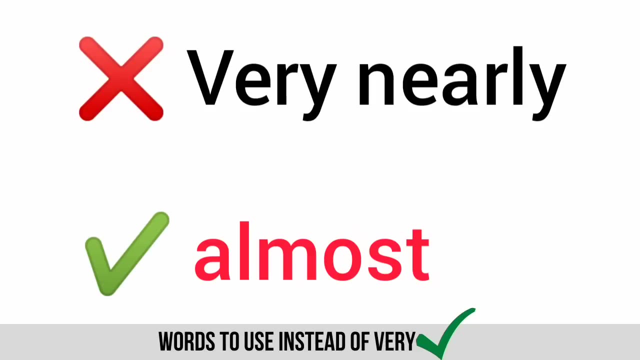 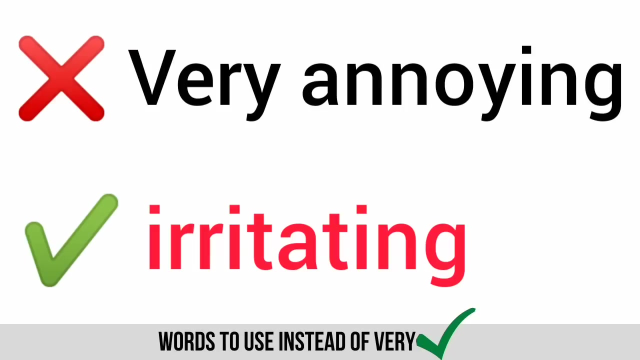 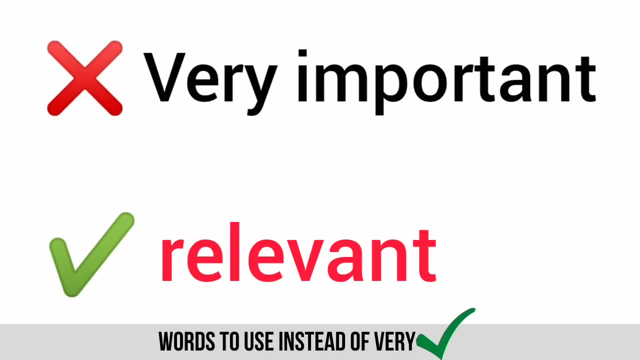 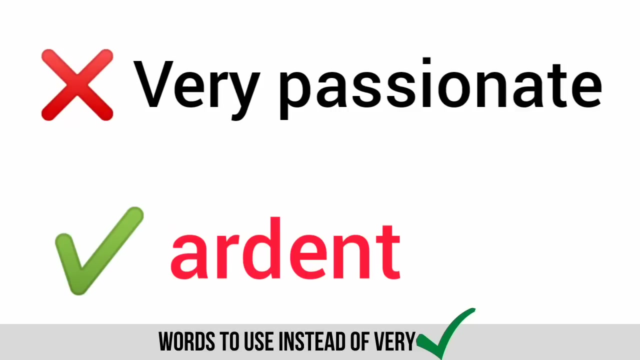 very lively, vivacious, very lively, vivacious. Very nearly almost, very nearly, almost, very annoying, irritating, very annoying, irritating. very important, relevant, very important, relevant, Very passionate, ardent, very passionate, ardent. 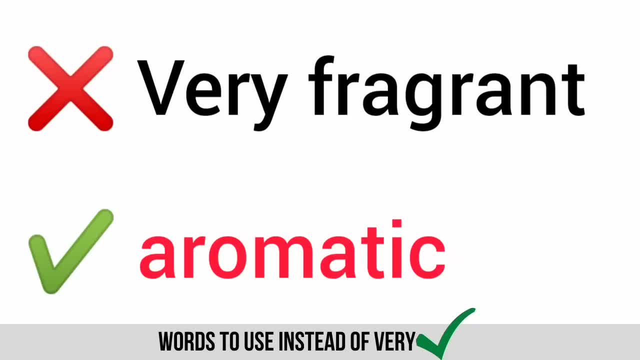 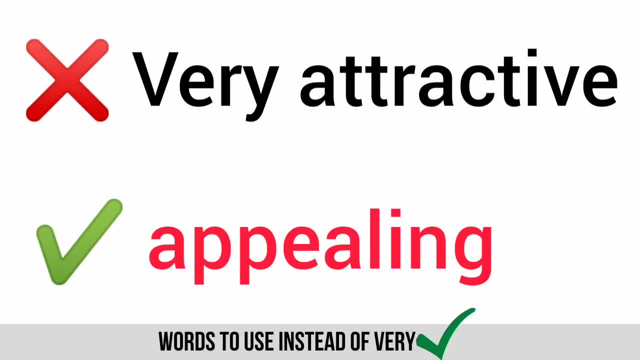 Very fragrant, aromatic, very fragrant aromatic, very attractive, appealing, very attractive, very attractive, appealing, very attractive, appealing, very attractive. You probably didn't notice something interesting, I think we Belin, we Belin. Exactly, I think we Belin helps Alola stand out and our Americanna can always be like Bra Din, or yeah, she is a very, very brilliant Poet Pho And she, she seems to be very, very, very innovative indeed. 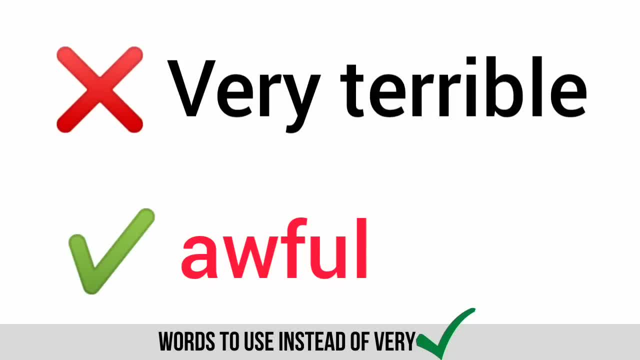 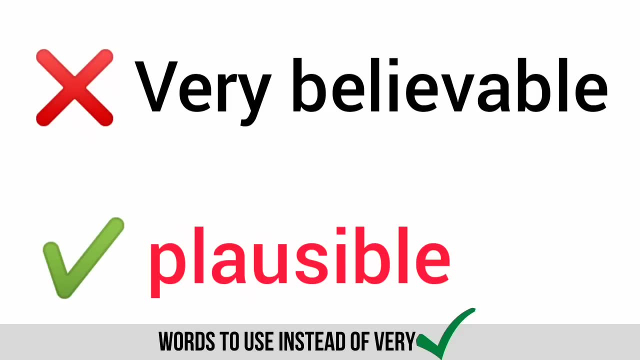 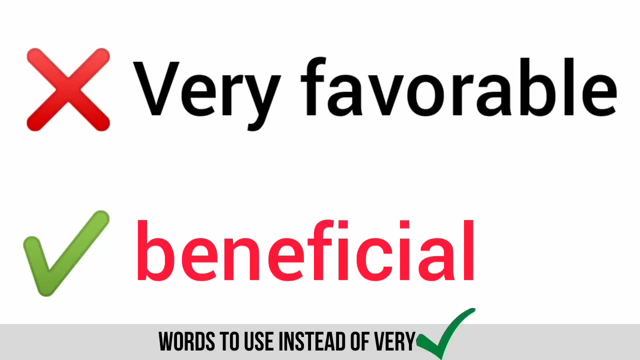 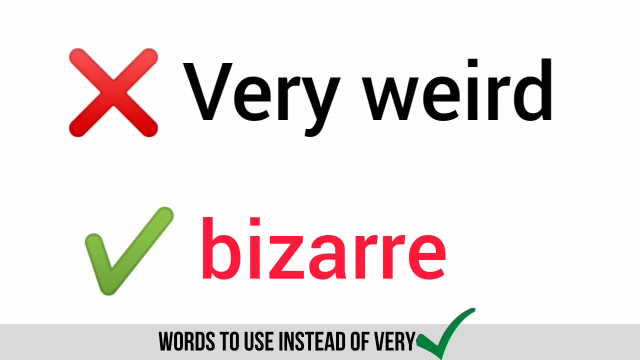 She seems to be very, very obras, very, very good and very active, but still I think she's appealing very terrible, awful, very terrible awful, very believable, plausible, very believable, plausible, very favorable, beneficial, very favorable, beneficial. very weird, bizarre, very weird bizarre. 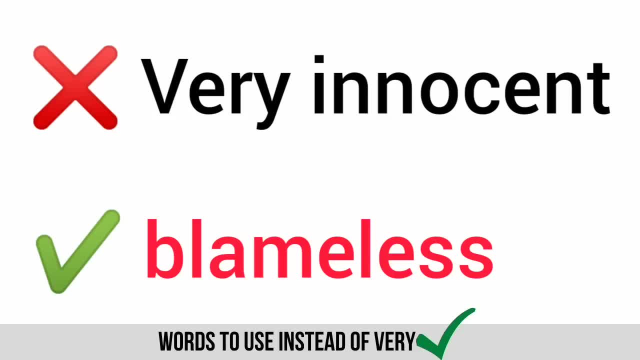 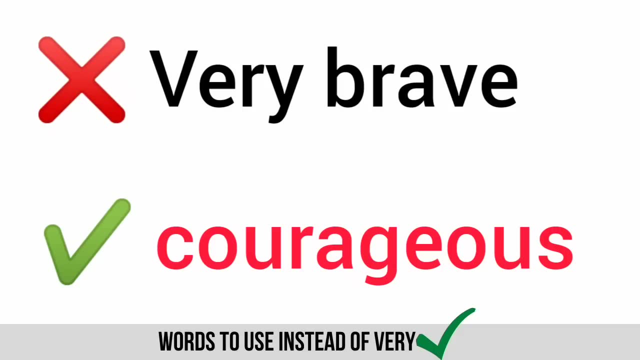 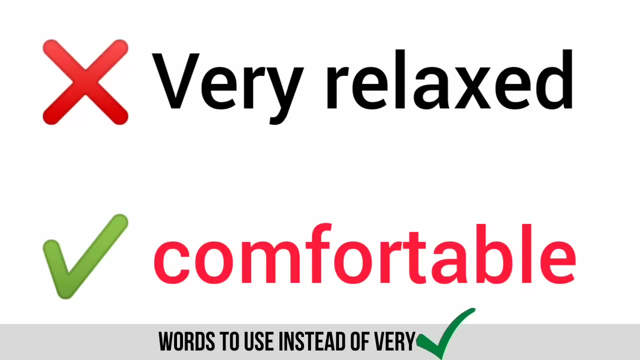 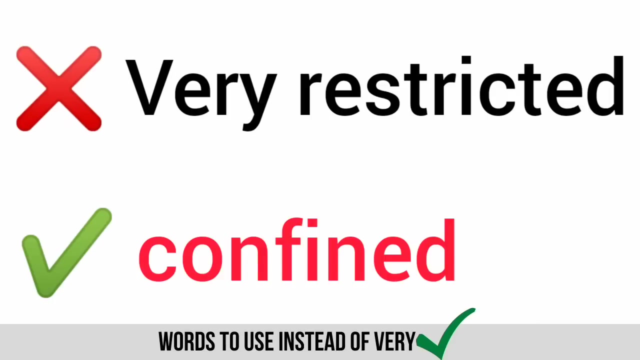 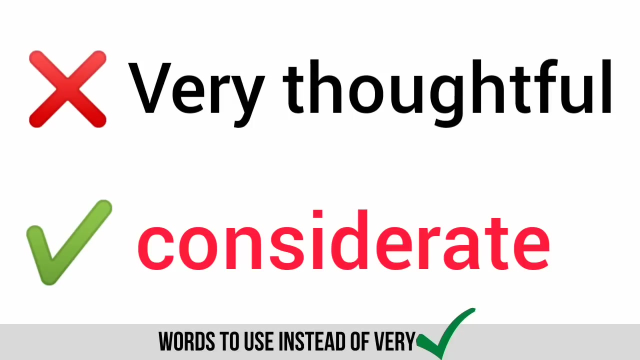 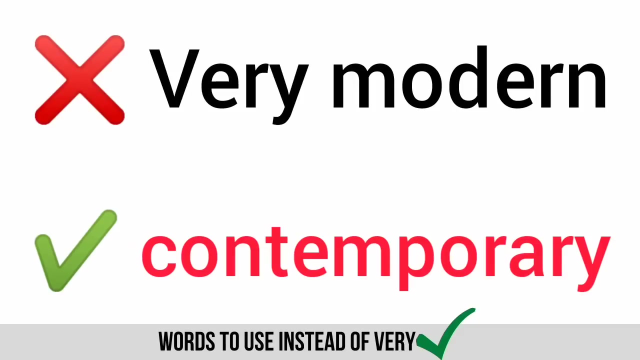 very innocent, blameless, very innocent, blameless, very brave, courageous, very brave, courageous. very relaxed, comfortable, very relaxed, comfortable, very restricted, confined, very restricted, confined, very thoughtful, considerate, very thoughtful, considerate very modern, contemporary, very modern, contemporary, very opposite. 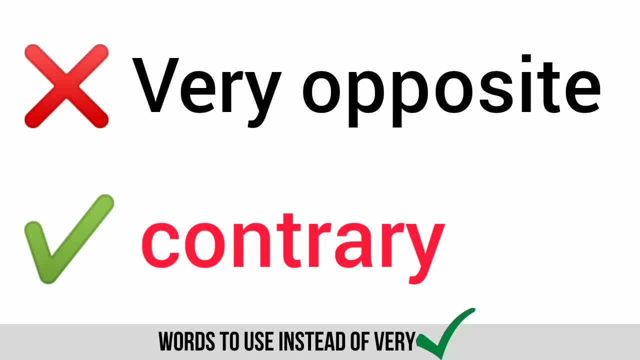 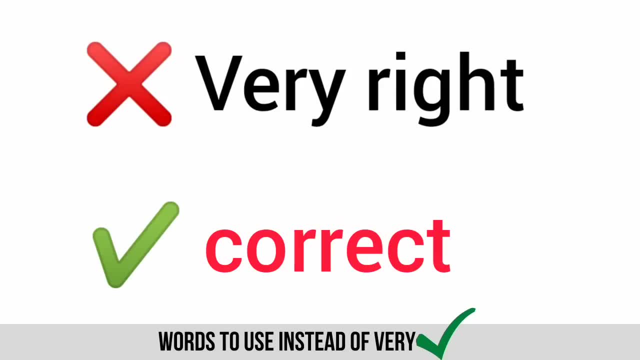 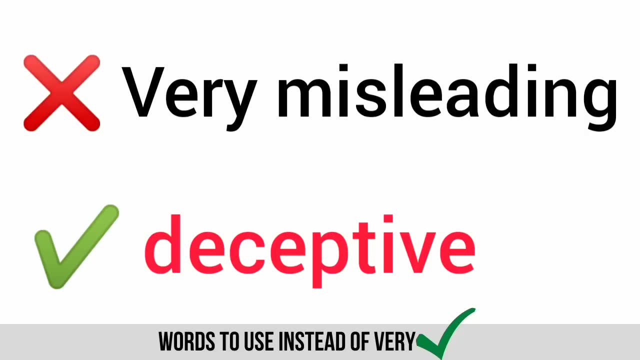 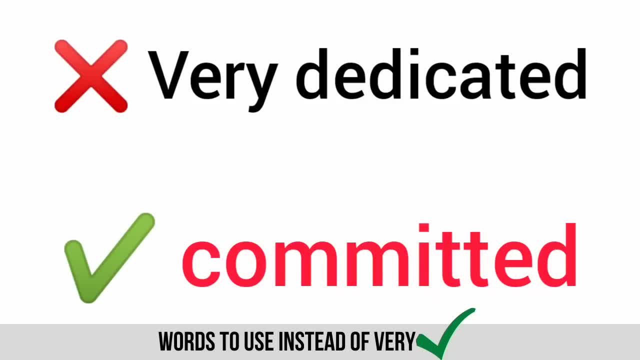 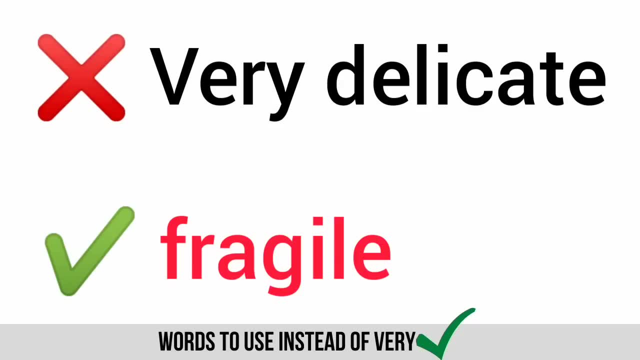 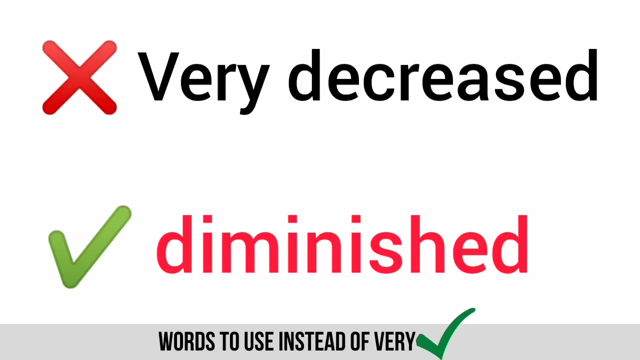 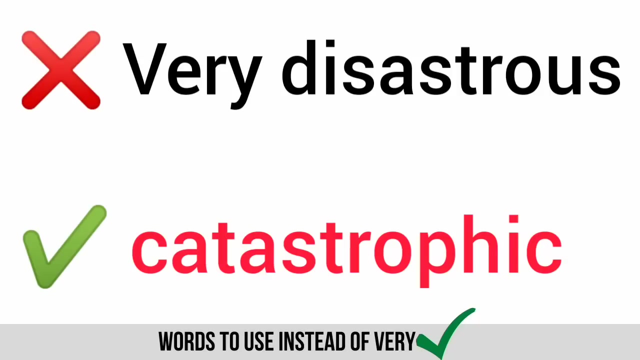 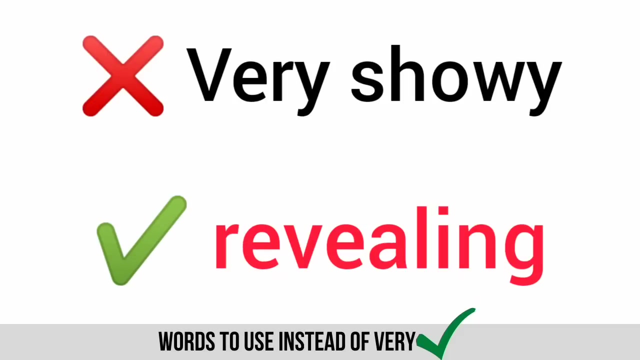 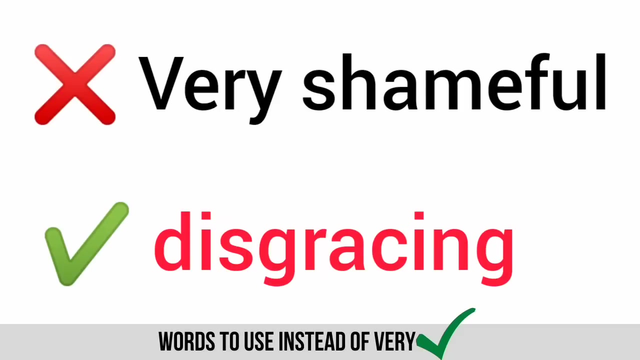 committed, very dedicated, committed, very delicate, fragile, very delicate, fragile, very decreased, diminished, very decreased, diminished, very disastrous, catastrophic, very disastrous, catastrophic, very showy, revealing, very showy, revealing, very shameful, disgracing, very shameful, disgracing, very selfish, egocentric. 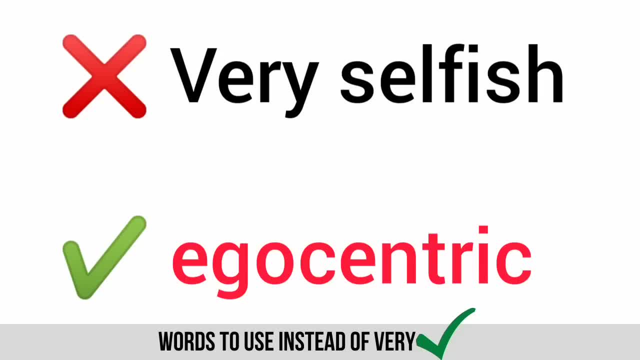 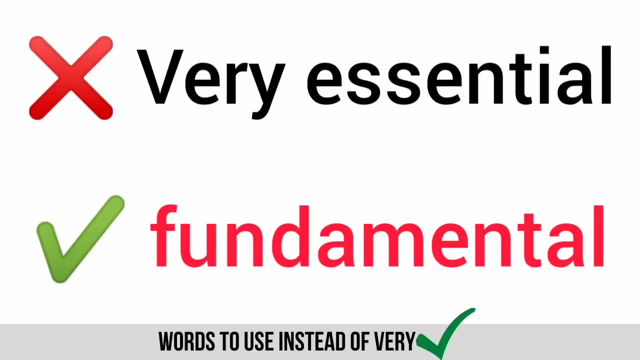 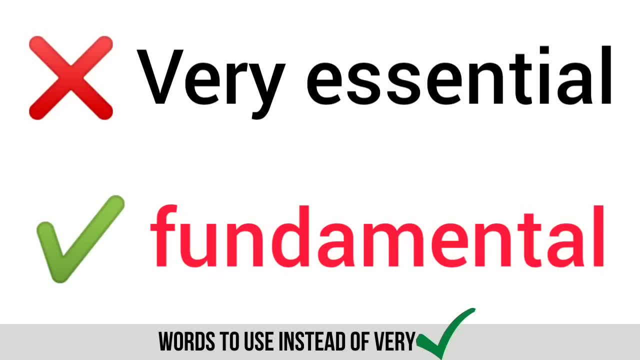 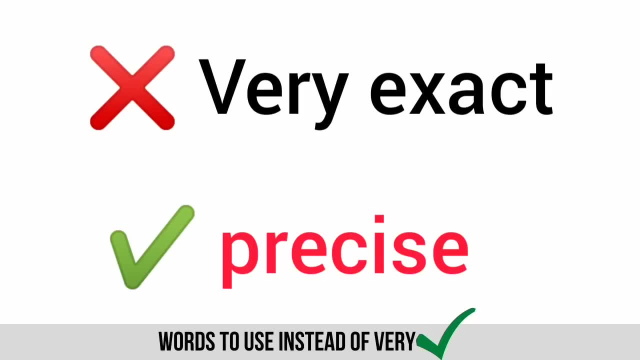 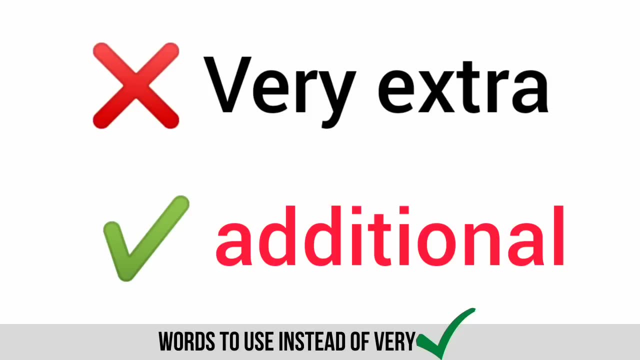 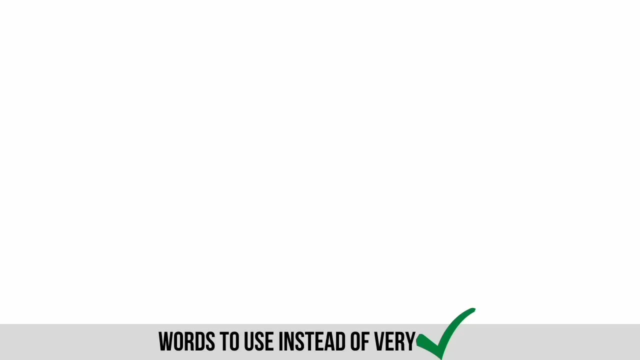 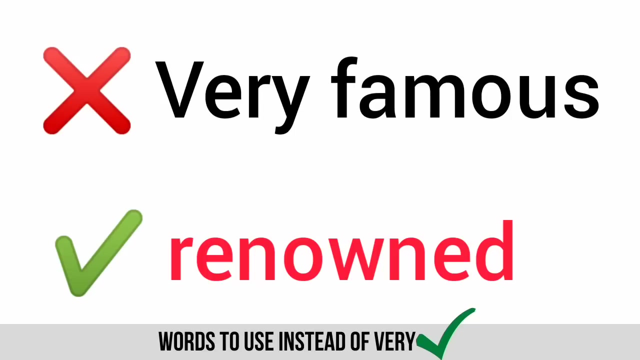 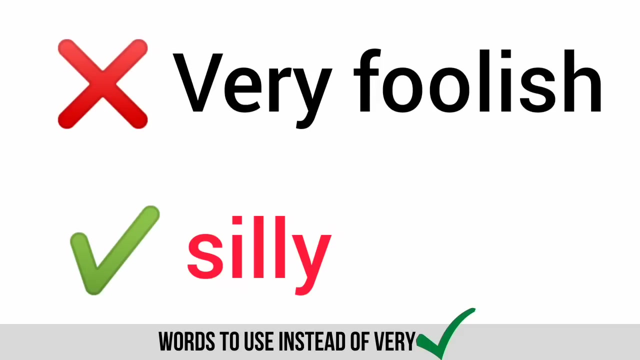 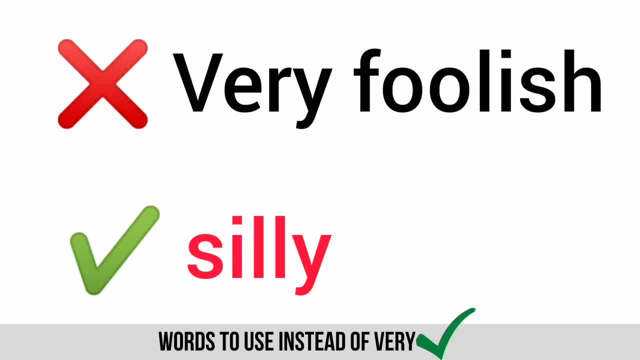 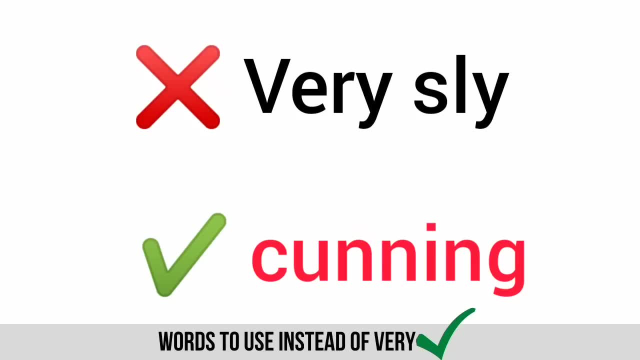 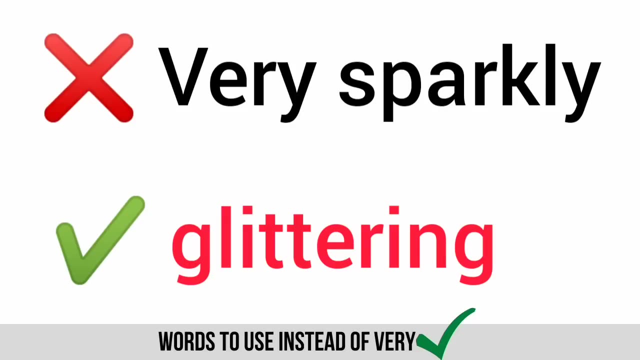 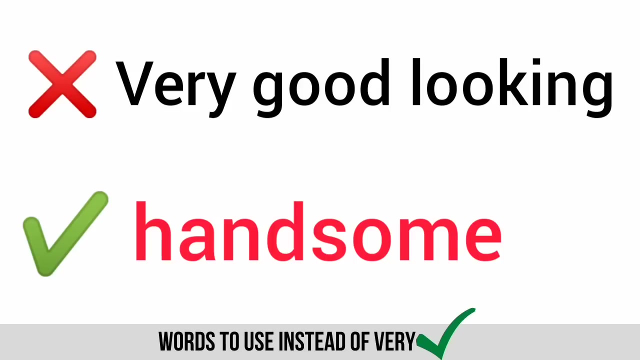 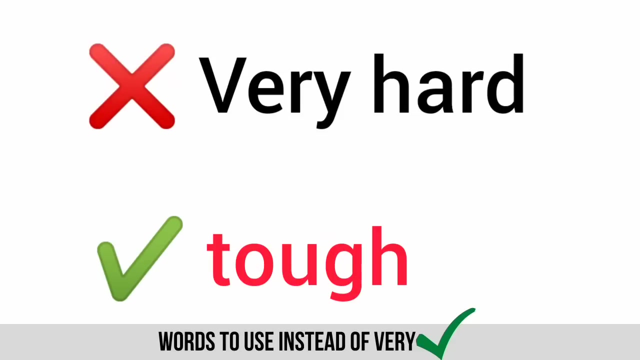 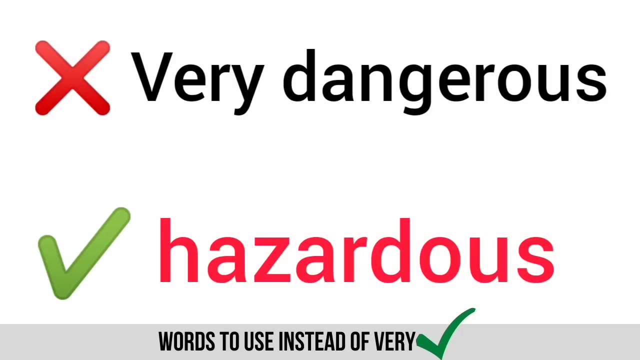 very foolish, silly, very sly Cunning, very sly cunning, very sparkly, glittering, very sparkling, glittering, very good-looking handsome, very good-looking handsome. very hard, Tough, very hard, tough, very dangerous, hazardous, very dangerous, hazardous, very. 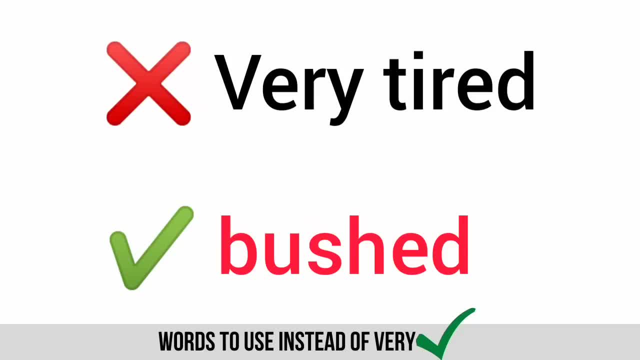 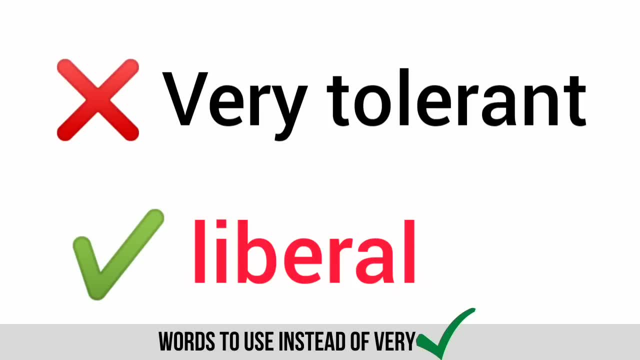 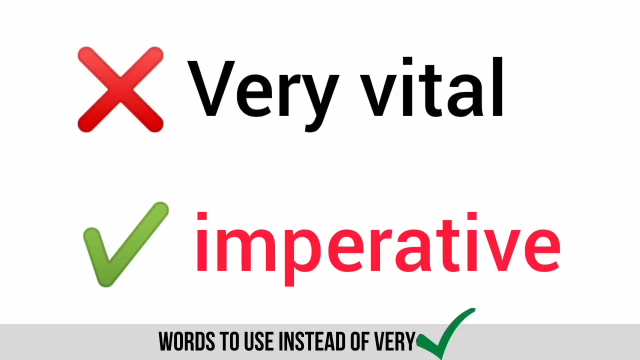 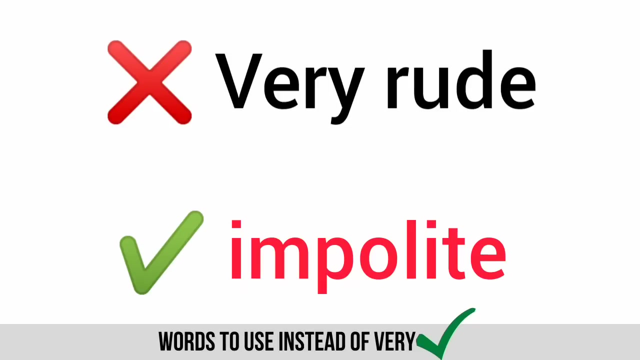 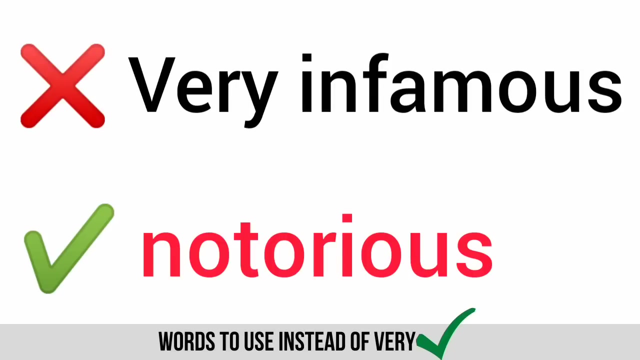 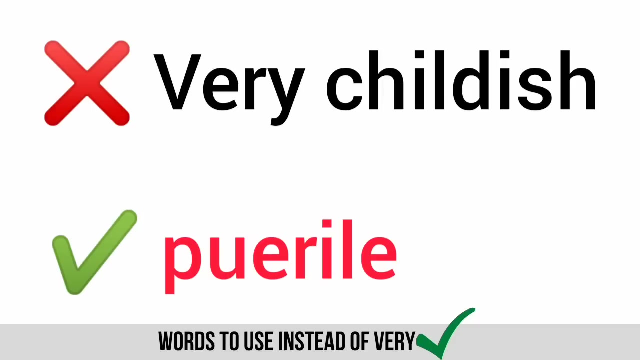 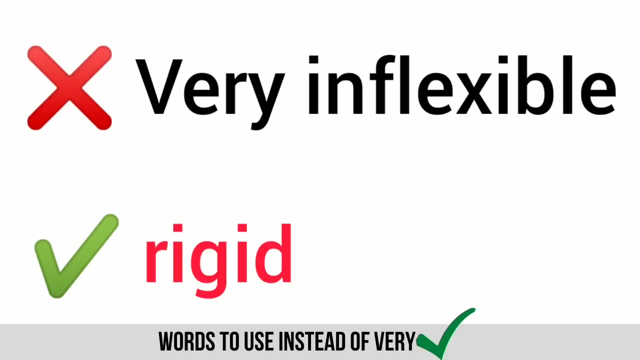 tired, pushed, very tired, pushed. very tolerant, liberal, Very vital imperative, very vital imperative. very rude, impolite, very rude, impolite, very infamous, notorious, Very infamous, notorious, very childish, puerile, very childish puerile, very inflexible. 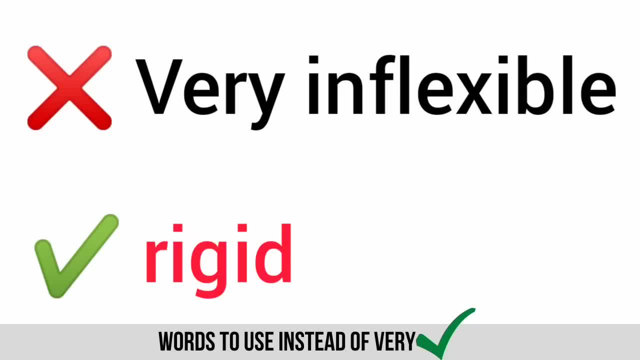 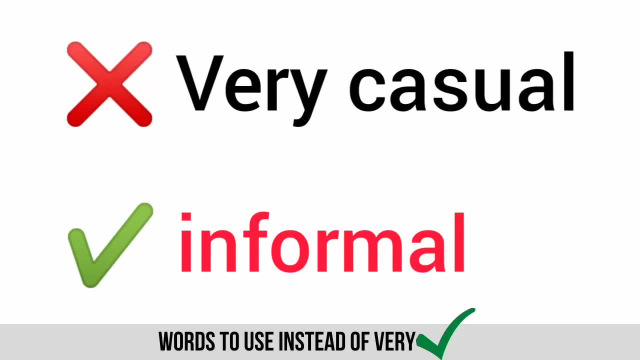 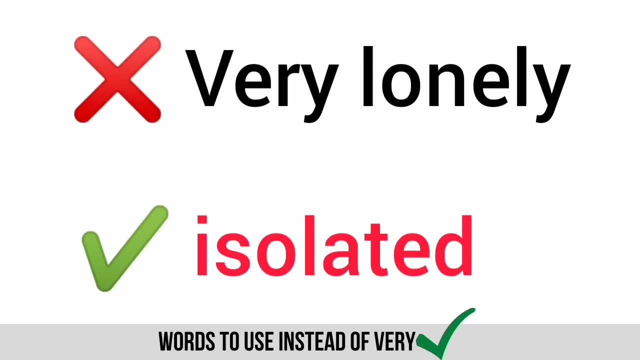 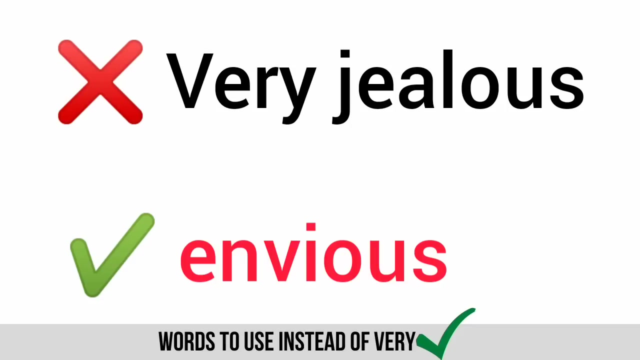 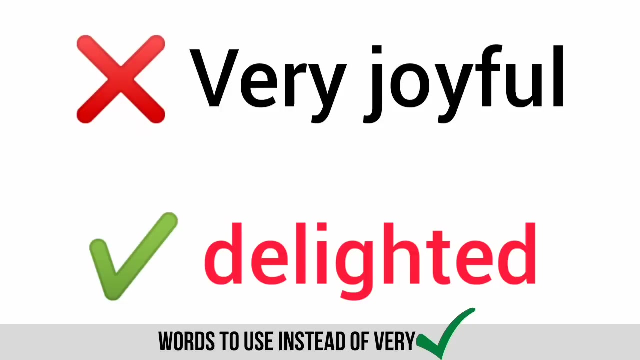 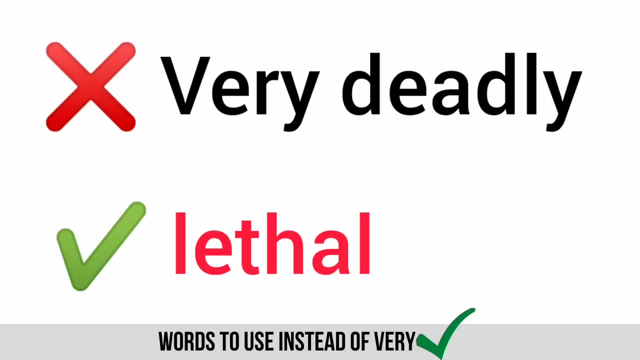 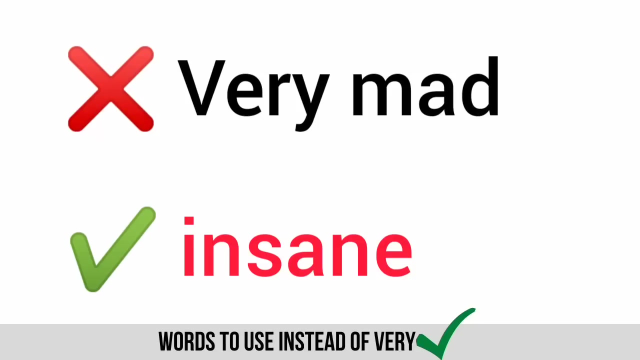 rigid, very inflexible, rigid, very casual, informal, Very lonely, isolated, very lonely, isolated, very jealous, envious, very jealous, envious, very joyful, delighted, delighted, Innocent, Very joyful, delighted, very deadly, lethal, very deadly lethal, very mad, insane very. 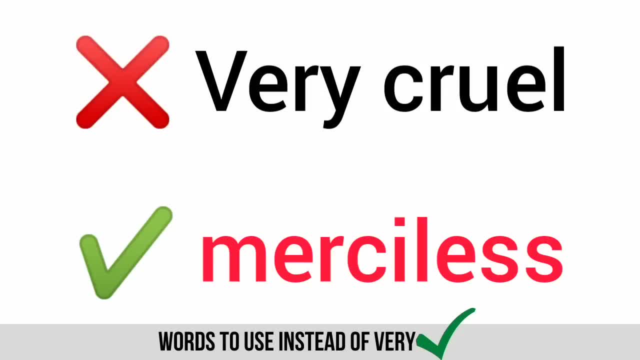 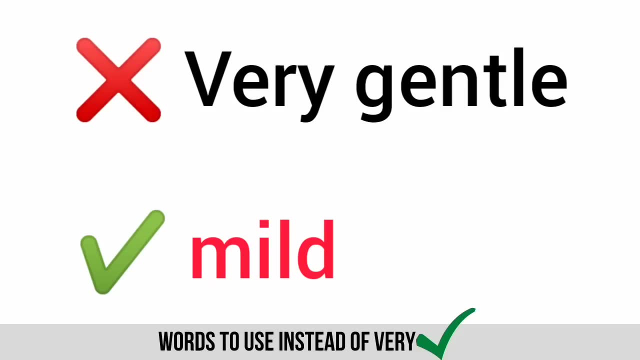 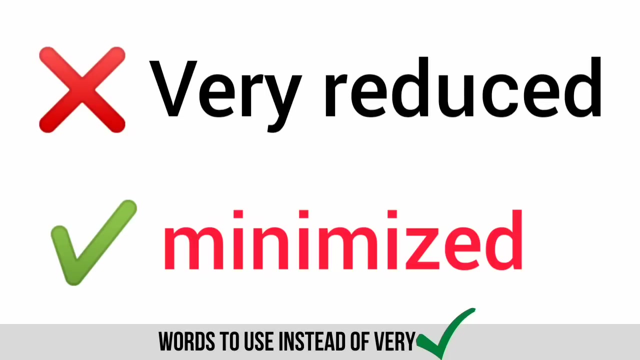 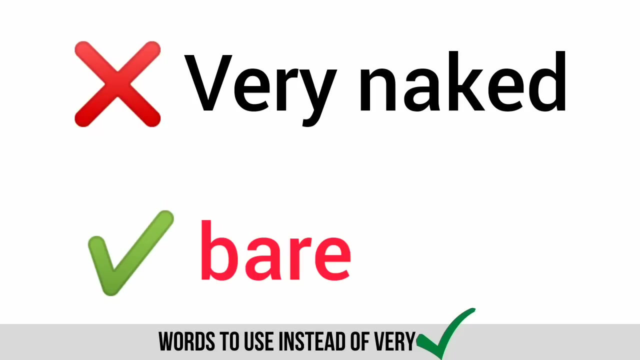 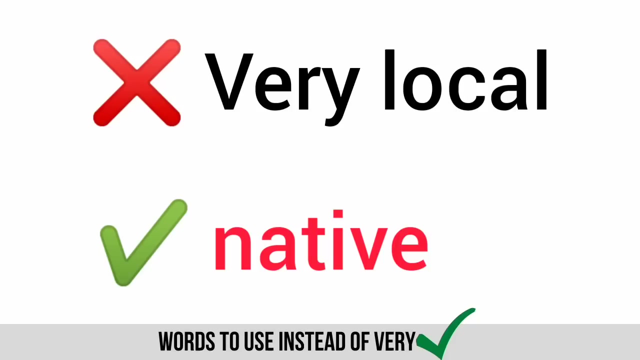 mad, insane, very cruel, merciless, very cruel, merciless, very gentle, mild, very gentle, mild, very reduced, minimized, very reduced, Very reduced, minimized. very naked, bare, very naked bare, very local, native, very. 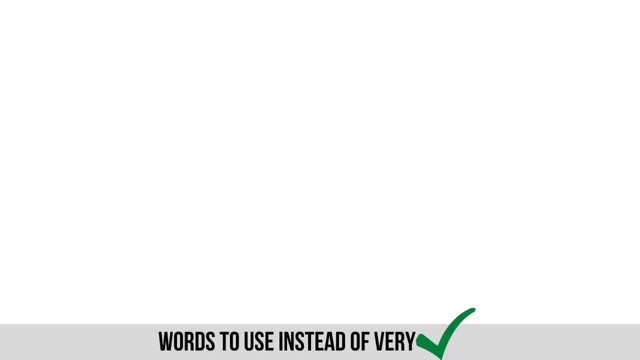 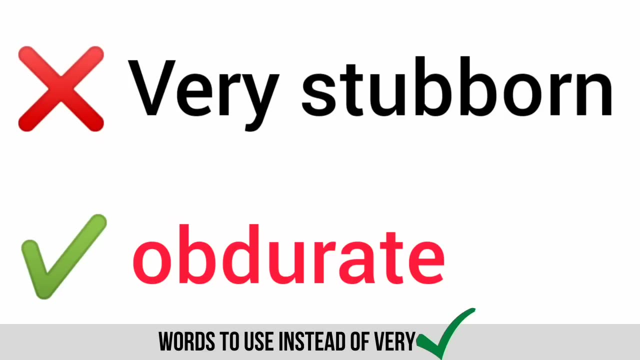 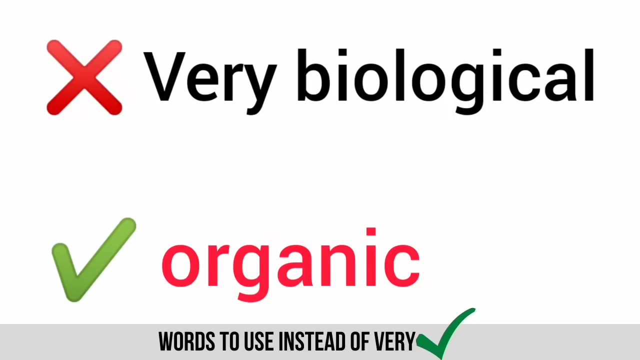 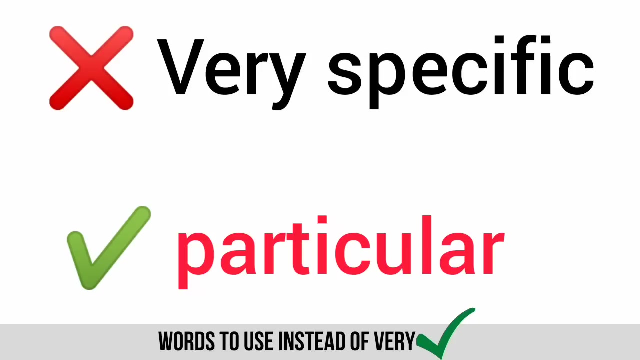 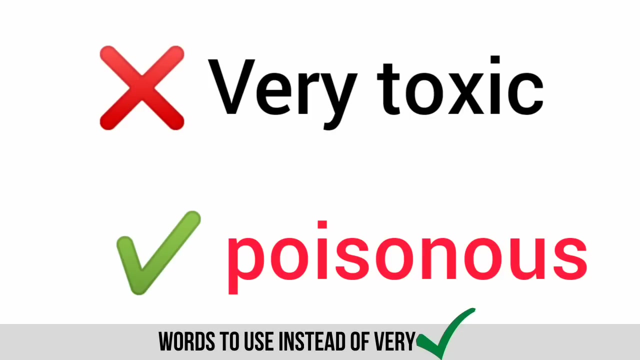 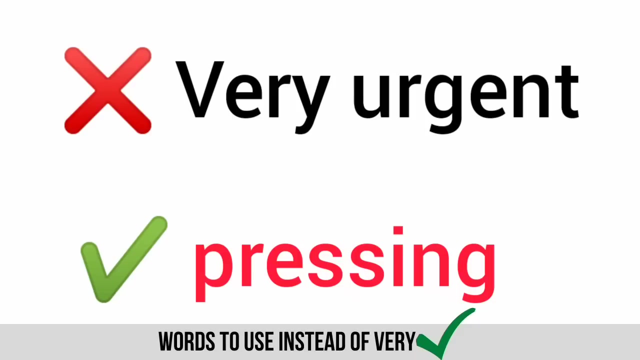 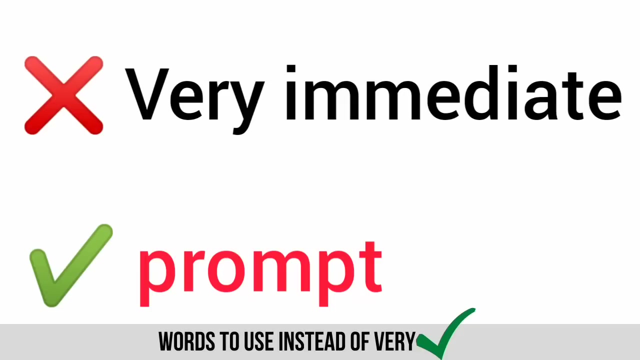 local, native, very stubborn, obdurate, very stubborn, Obdurate, very biological, organic, very biological, organic, very specific, particular, very specific, particular, very toxic, poisonous, Very toxic, poisonous, very urgent, pressing, very urgent, pressing, very immediate, prompt. 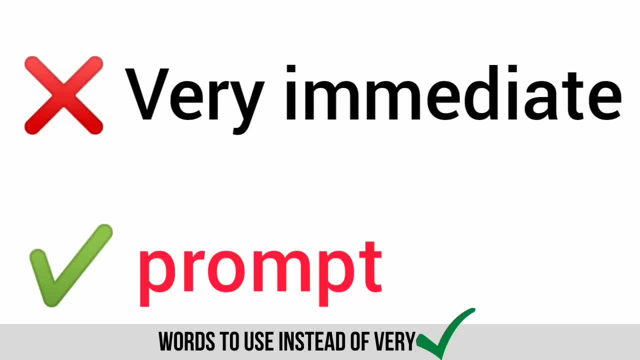 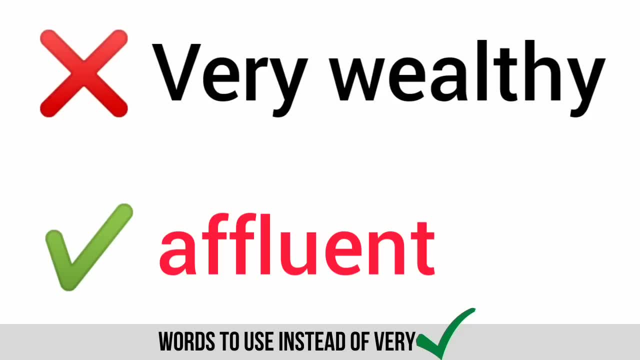 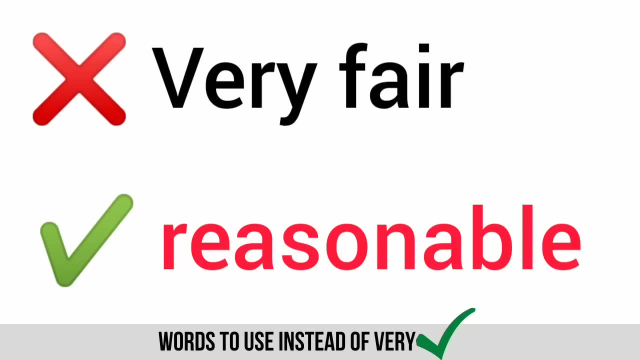 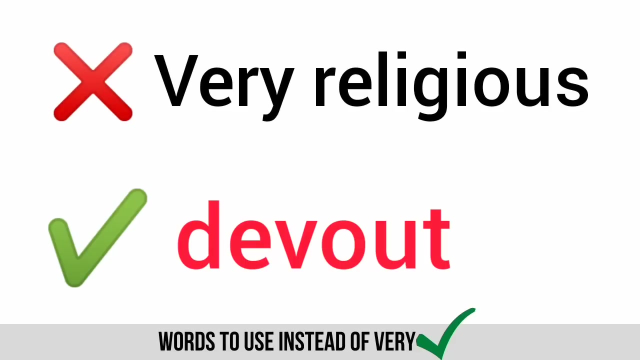 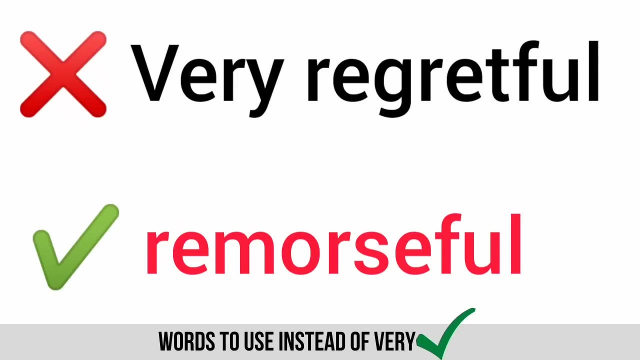 very immediate, prompt. very wealthy affluent, Very wealthy affluent, very fair, reasonable, very fair reasonable, Very religious devout, very religious devout. Very regretful, regretful, Remorseful, very regretful, remorseful. 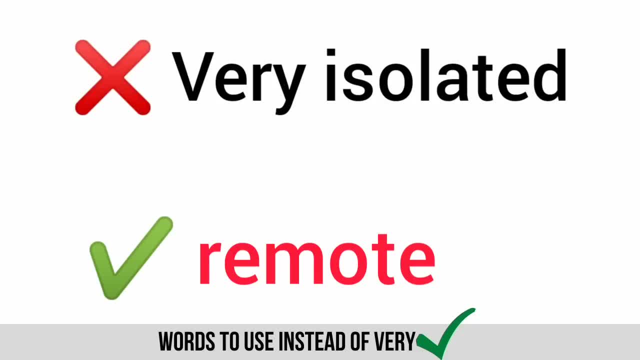 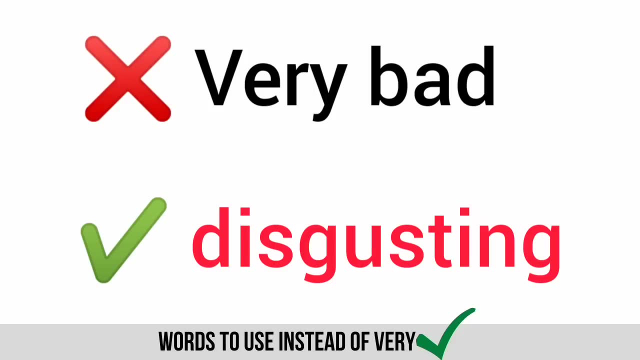 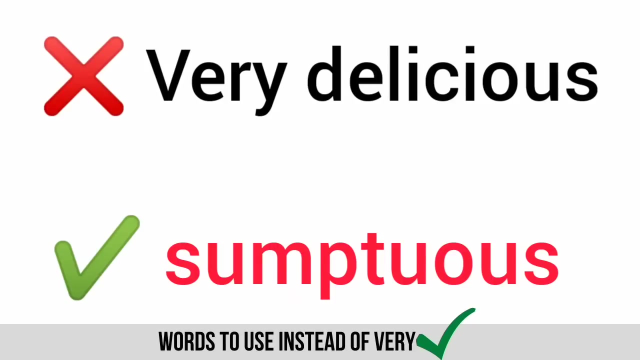 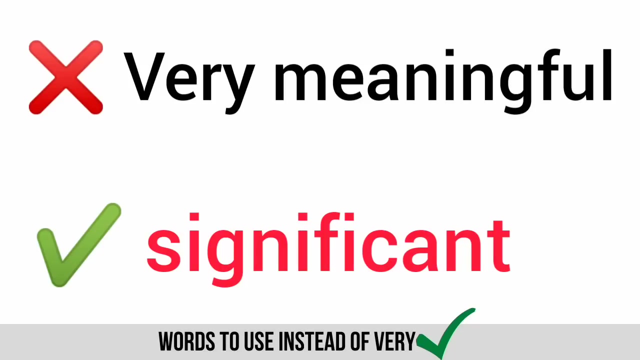 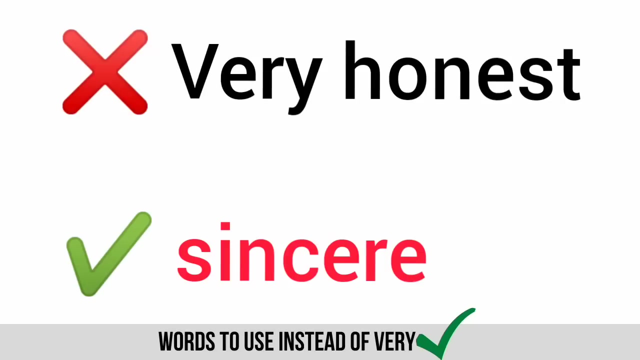 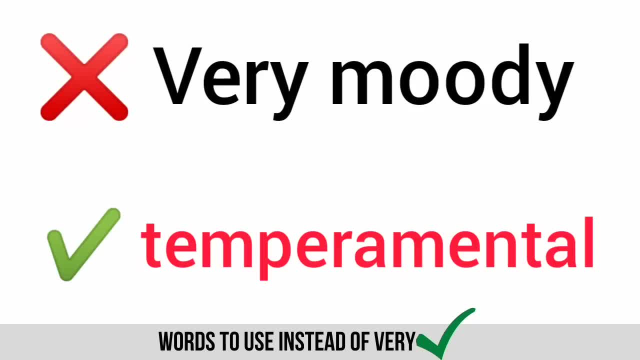 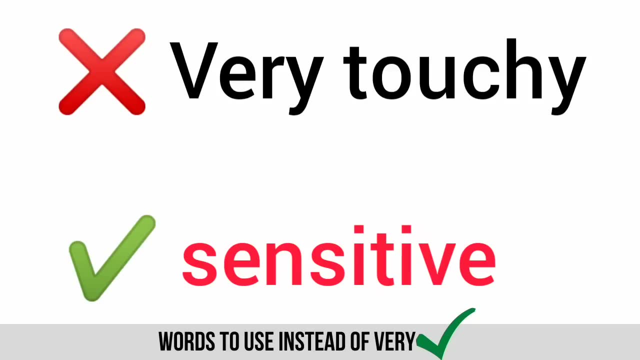 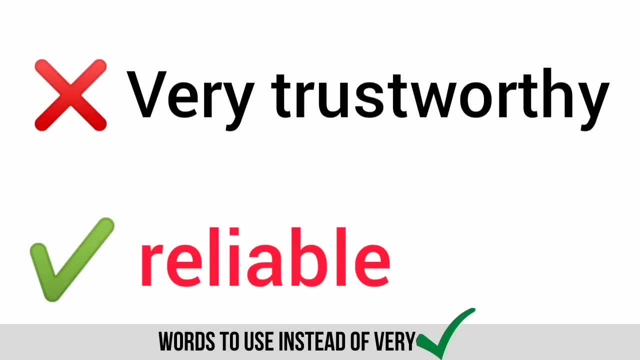 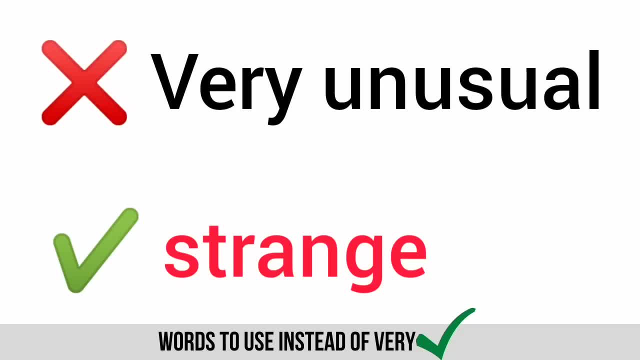 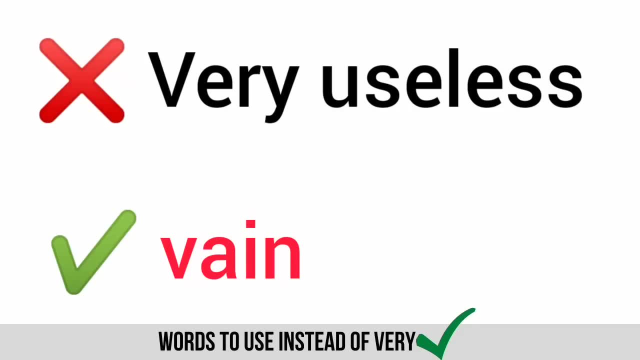 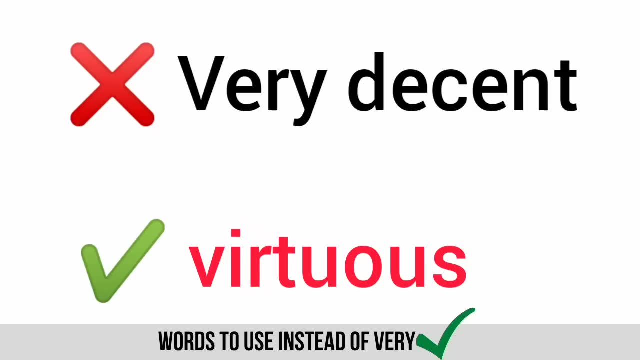 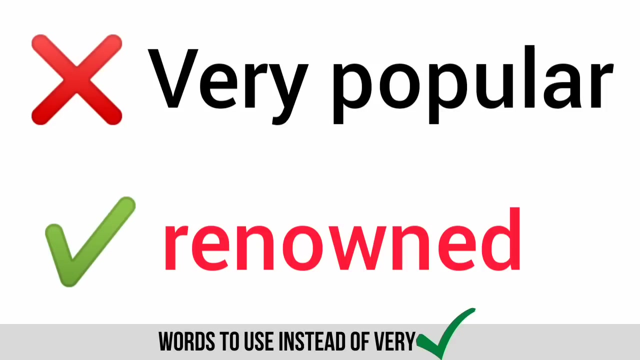 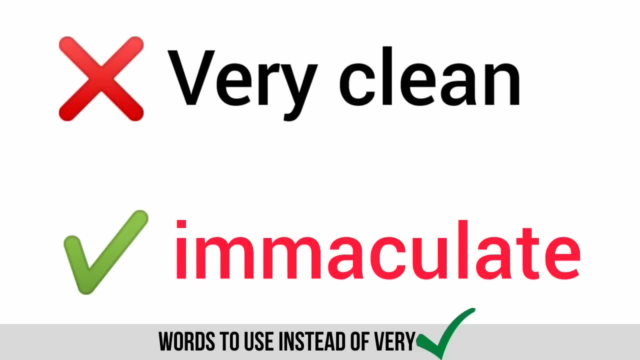 Strange, Very unusual, Strange, Very useless Vain, Very useless Vain Very decent, Virtuous, Very decent, Virtuous, Very popular. Renowned, Very popular. Renowned Very clean, Immaculate, Very clean. 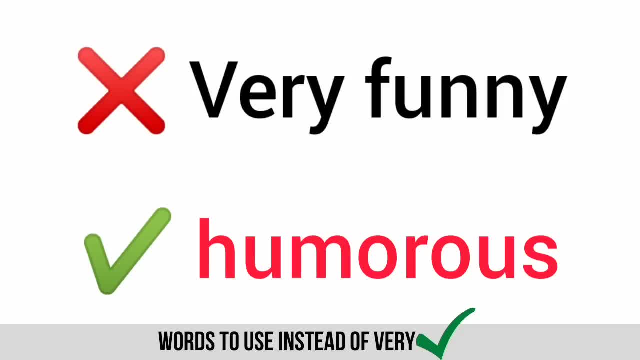 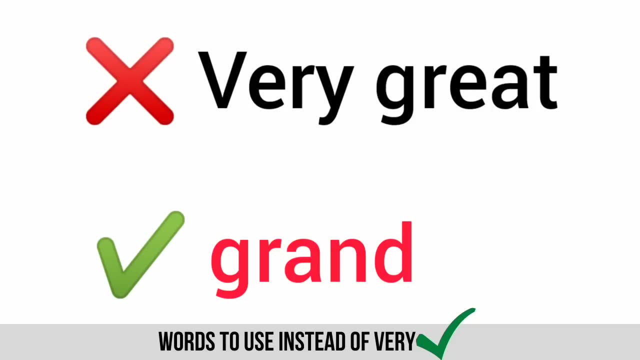 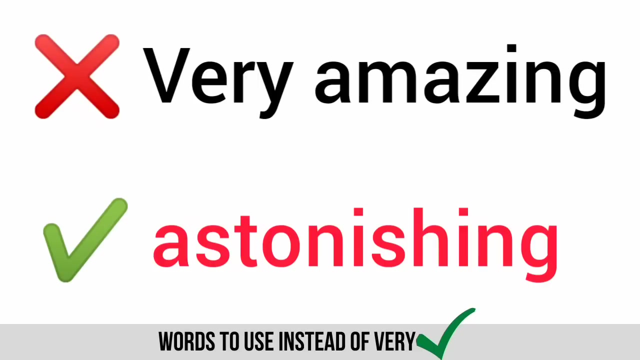 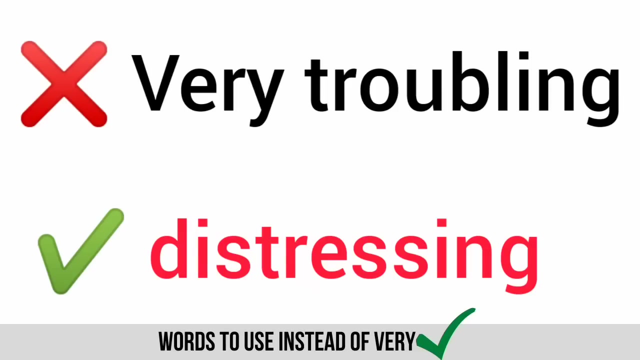 Immaculate, Very funny, Humorous, Very funny, Humorous, Very great Grand, Very great Grand, Very amazing, Astonishing, Very amazing, Astonishing, Very troubling, Distracting kids. Very hundred Est sid charged. 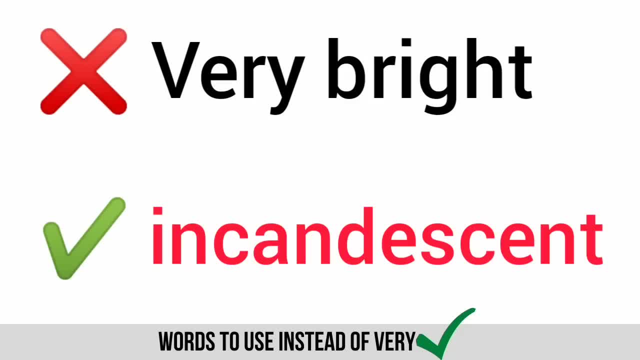 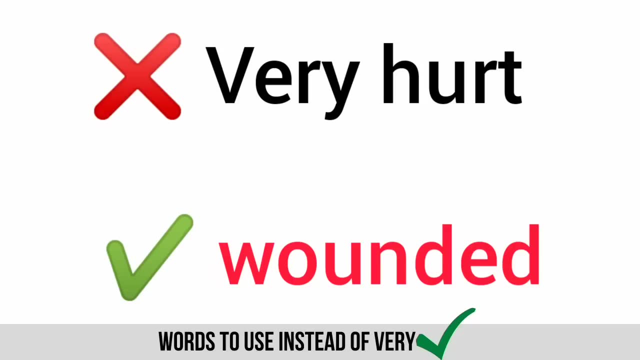 Very great: Distracting, Distracting Very Pirates. It's quite interesting. It's not Very bright, describing Very bright, Incandescent, Very bright, Incandescent, Very bright. It's so great, Very awful. 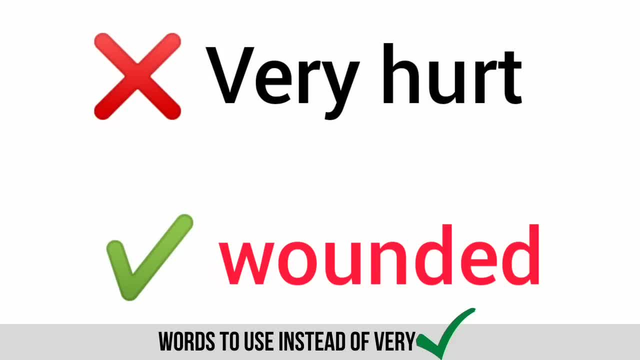 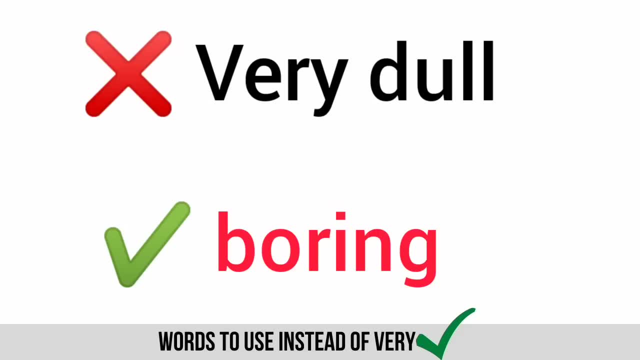 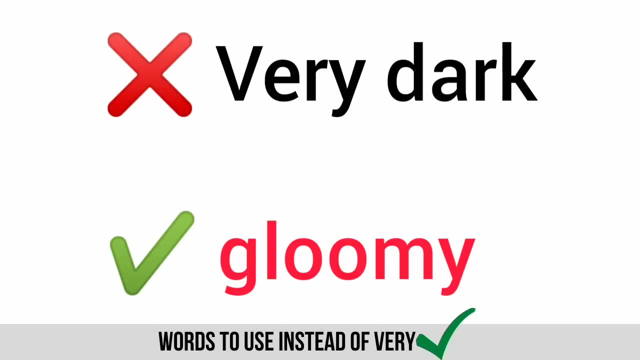 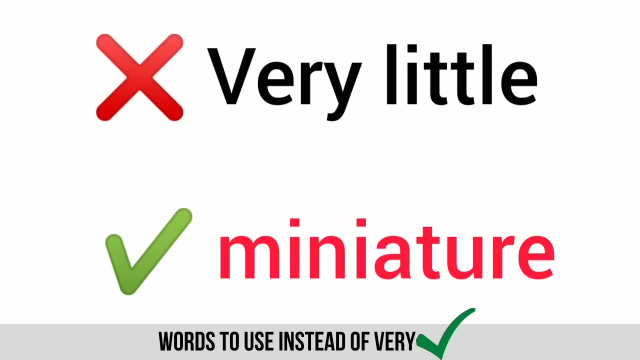 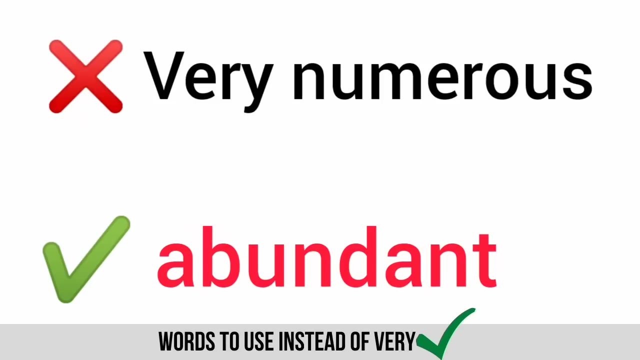 Very harsh, Very warm, Very hurt. Sixえ, Very hot, Wounded, Very dull, communal, retained, boring, very dull, boring, very dark, gloomy, very dark, gloomy. very little miniature, very little miniature. very numerous, abundant, very numerous, abundant, very active, energetic. 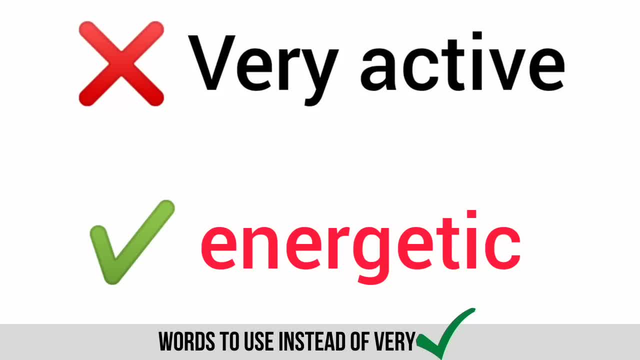 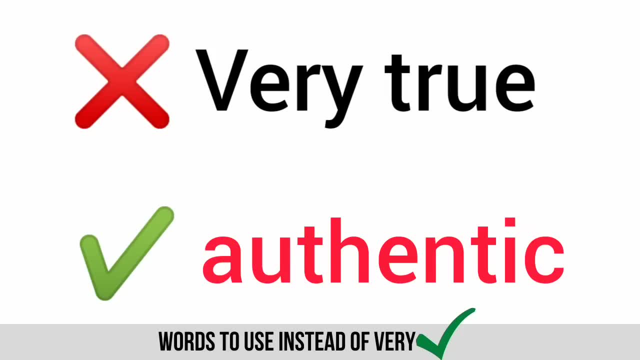 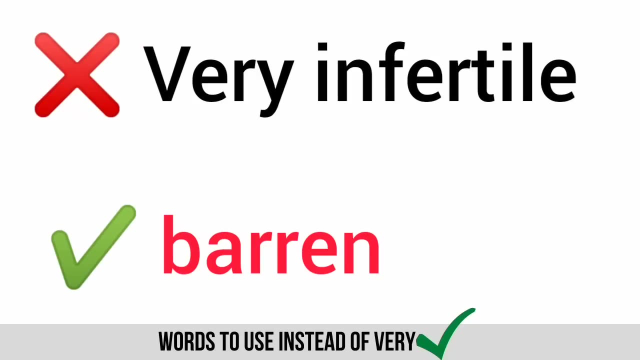 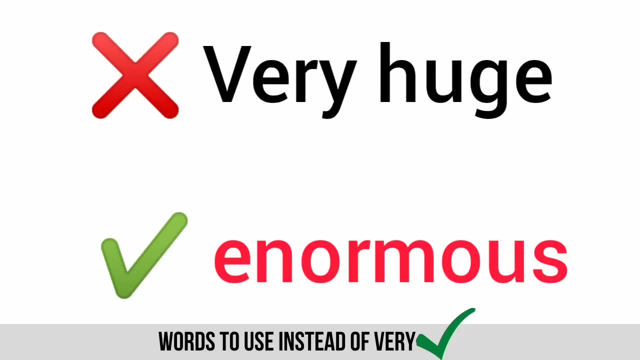 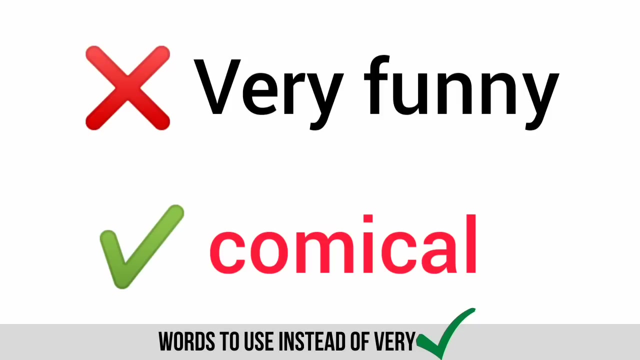 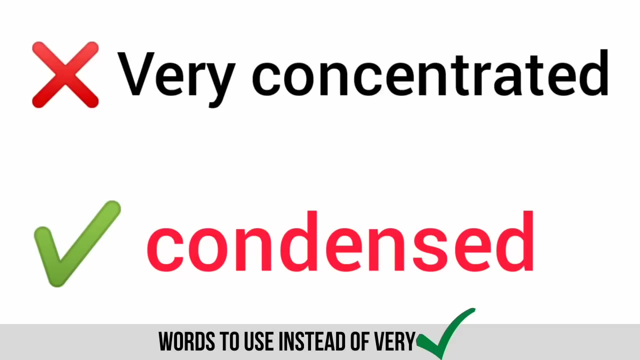 very active, energetic, very true, Authentic, very true, authentic. very infertile, barren, very infertile, barren. very huge, enormous, very huge, enormous, very funny, Comical, very funny, comical. very concentrated, condensed, very concentrated, condensed. 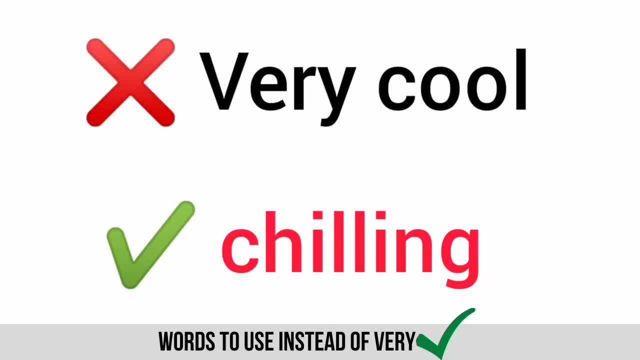 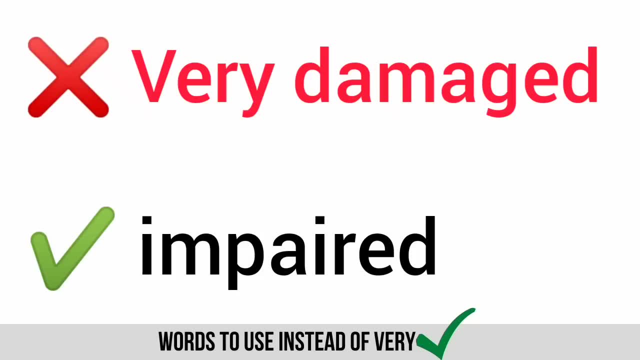 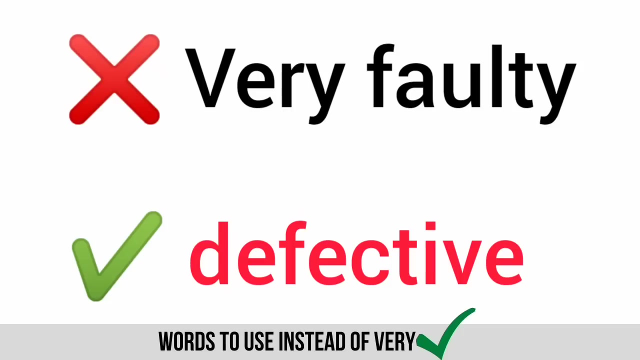 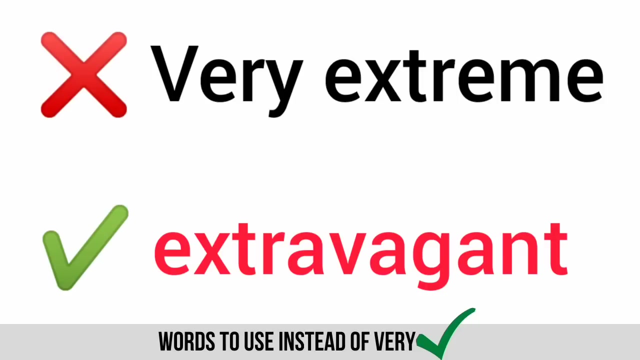 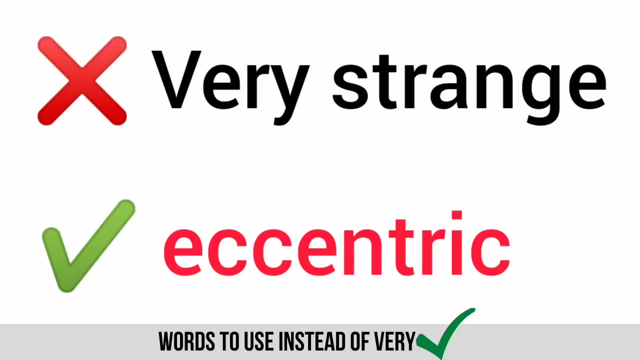 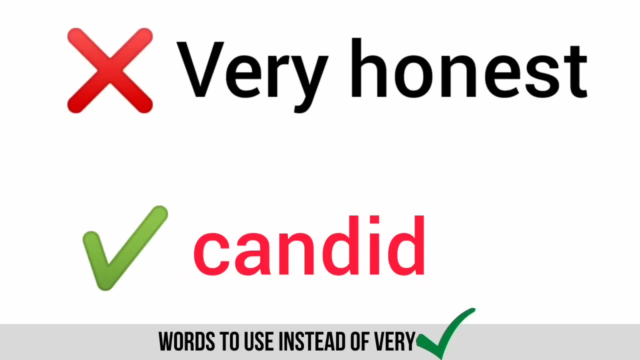 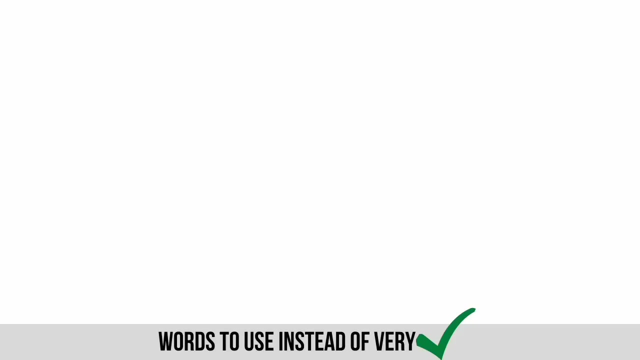 very cool, chilling, very cool, chilling, very cool, chilling. very damaged, impaired, very damaged, impaired, very faulty defective, very faulty defective, very extreme, extravagant, very extreme, extravagant, very strange, eccentric, very strange eccentric, very honest, candid, very honest, candid. 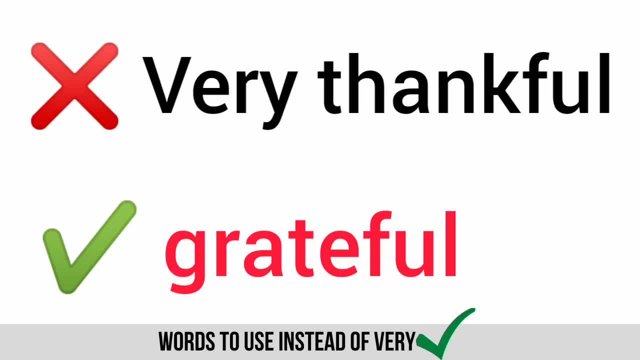 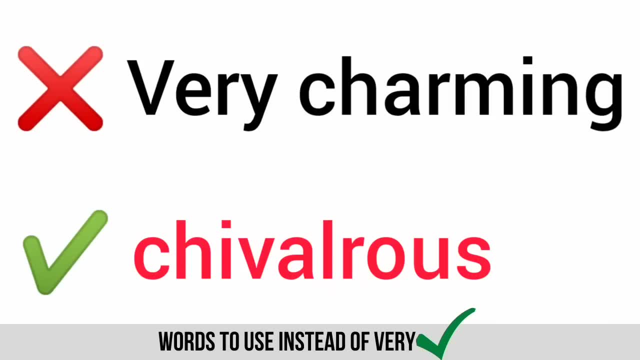 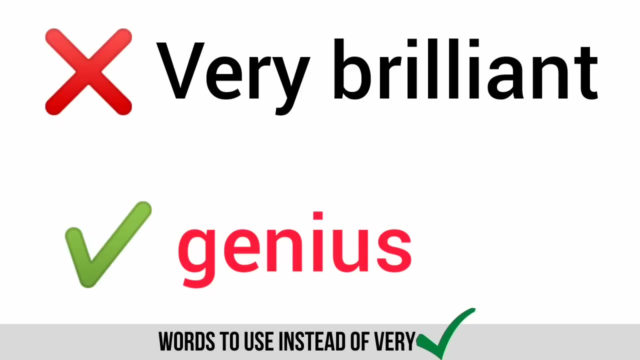 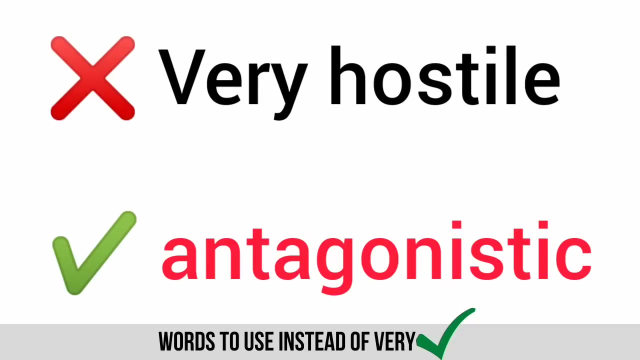 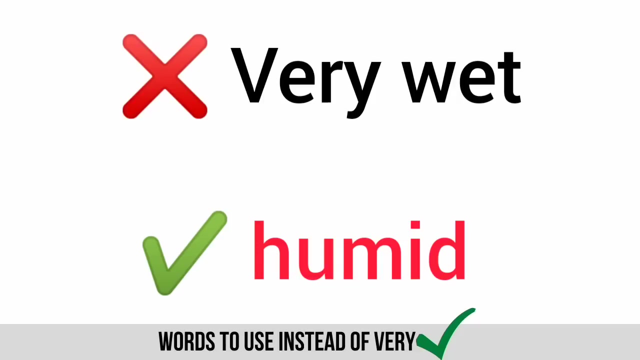 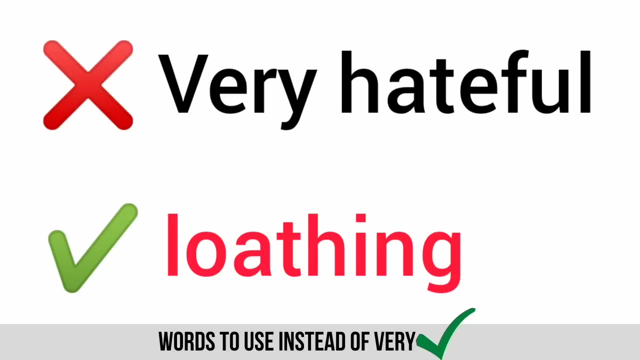 very thankful, grateful, very thankful, grateful. very charming chivalrous, very charming chivalrous, very brilliant genius, very brilliant genius. very hostile, antagonistic, very hostile, antagonistic, very wet, humid, very wet, humid. very hateful loathing, very hateful. 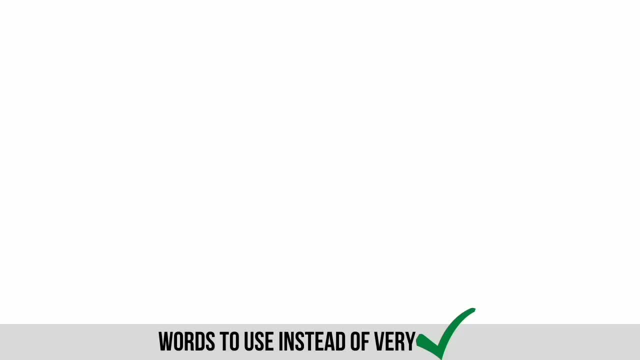 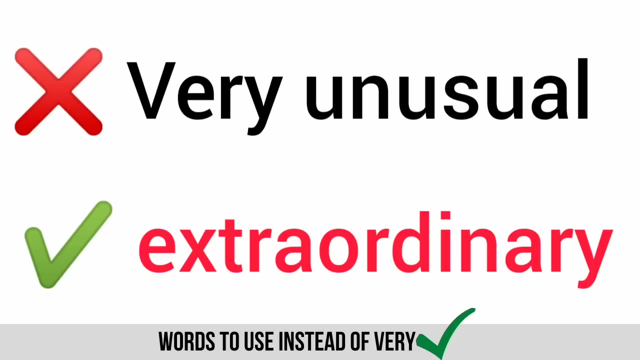 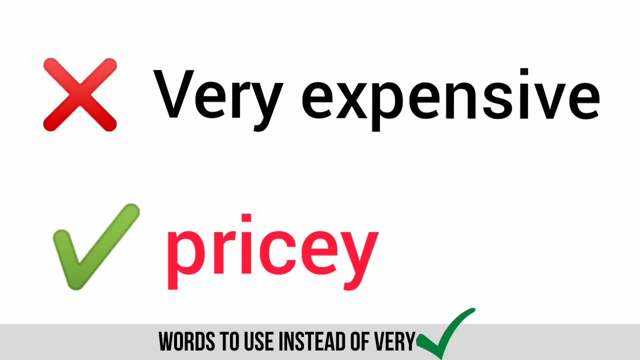 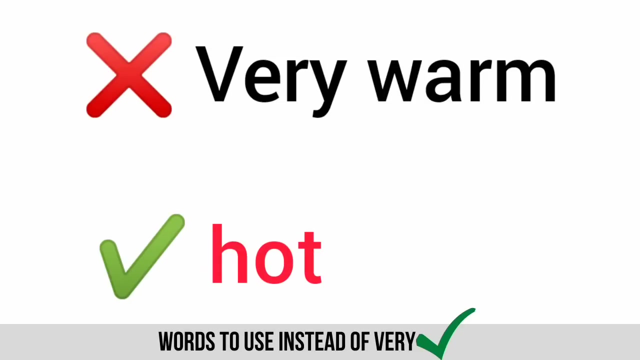 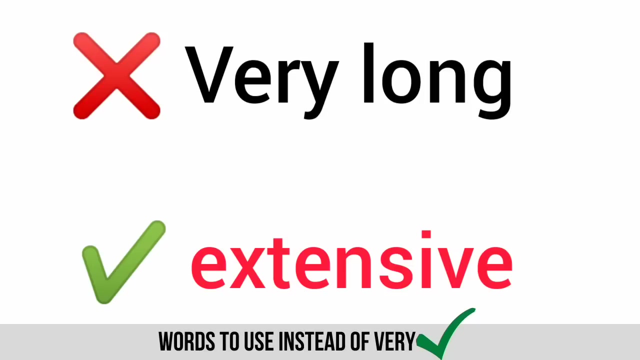 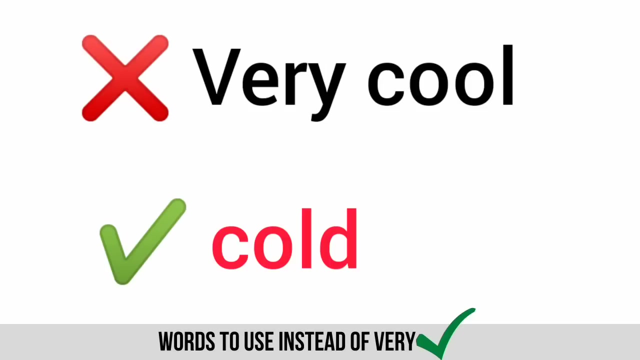 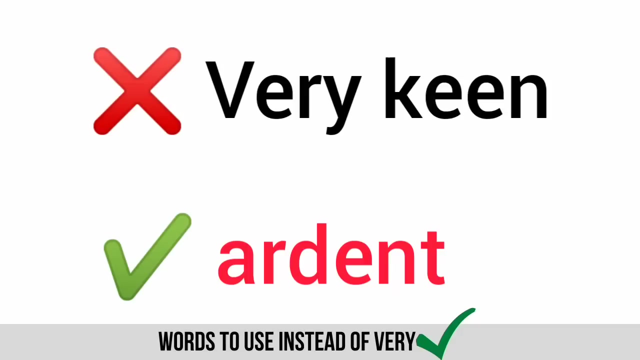 very hateful, very hateful loathing, very dirty filthy, very dirty filthy. very unusual, extraordinary, very unusual, extraordinary, very expensive, pricey, very expensive, expensive, pricey. very warm, hot, very warm hot, very long, extensive, very long extensive. very cool, cold, very cool cold. very keen, ardent, very keen ardent, very impressive. 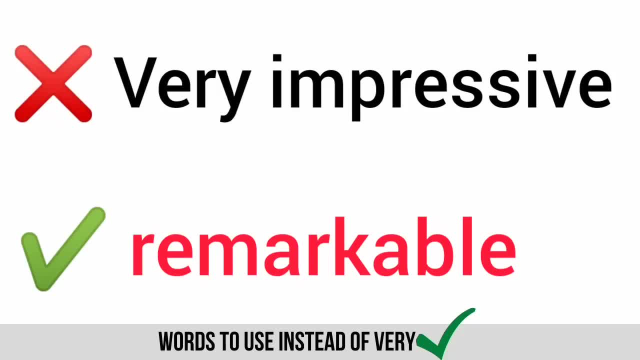 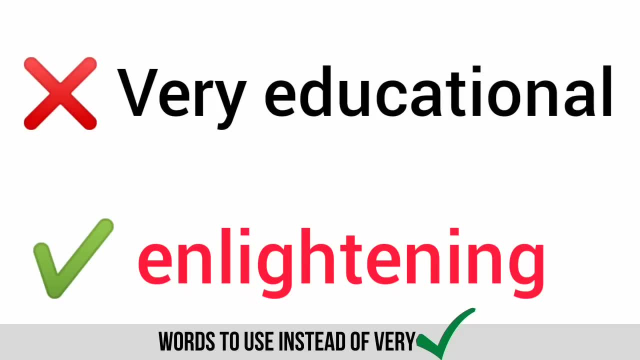 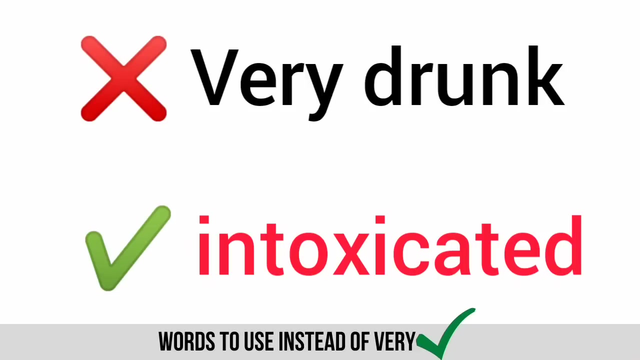 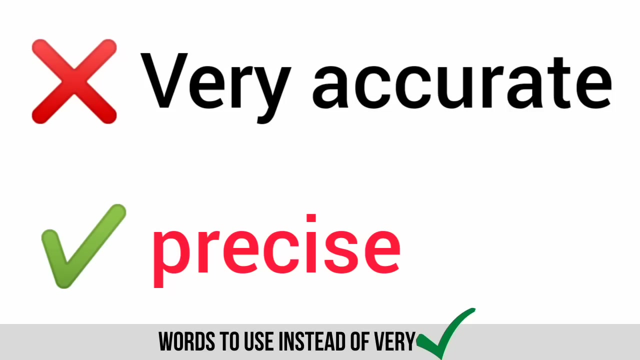 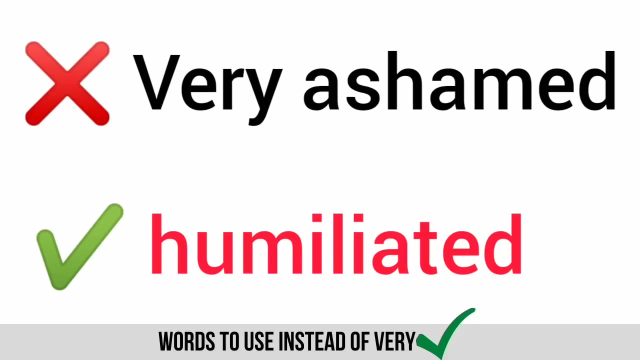 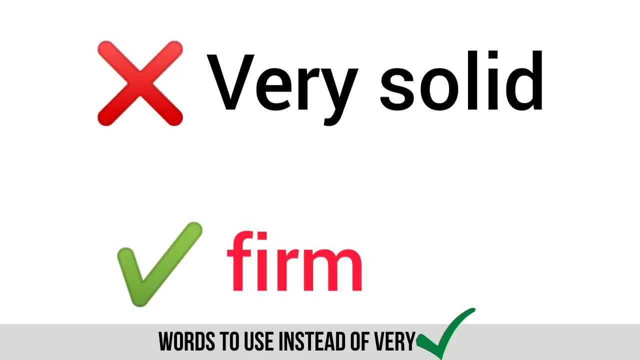 remarkable, very impressive, Remarkable, very educational, enlightening, very educational, enlightening. very drunk, intoxicated, very drunk intoxicated. very accurate, precise, Very ashamed, humiliated, very ashamed, humiliated. very solid firm, very solid firm, very forceful. 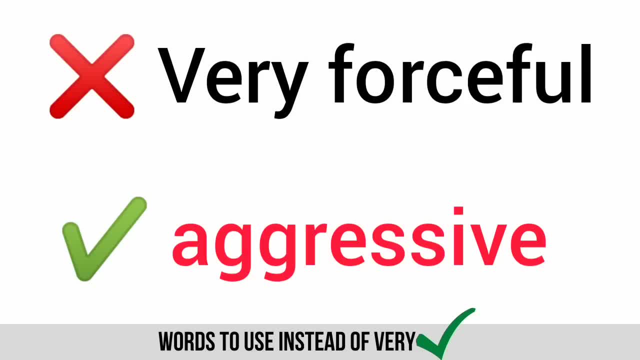 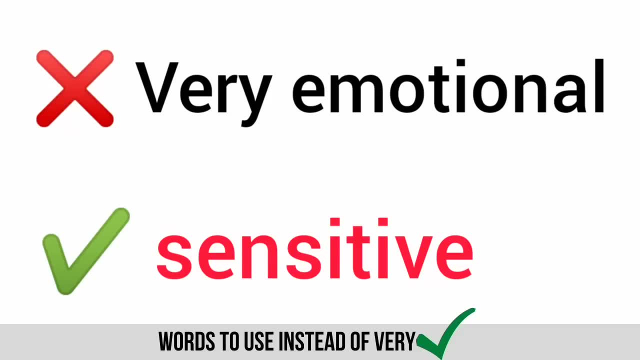 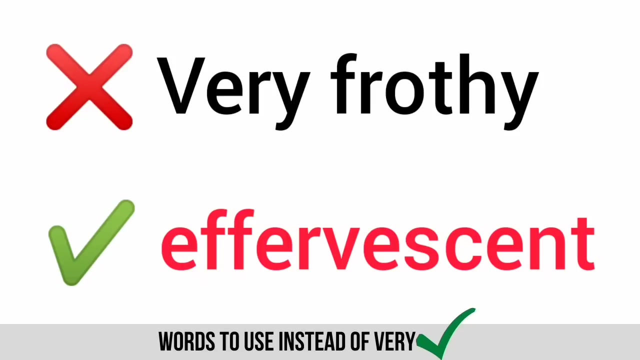 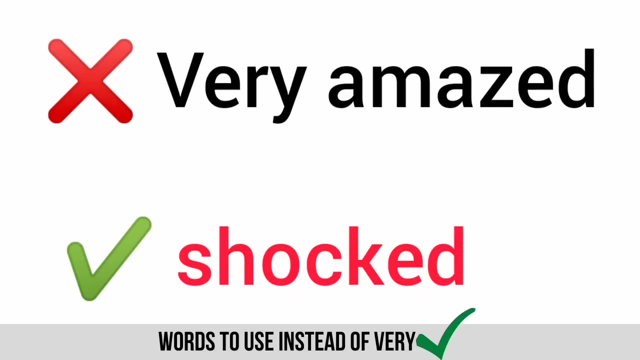 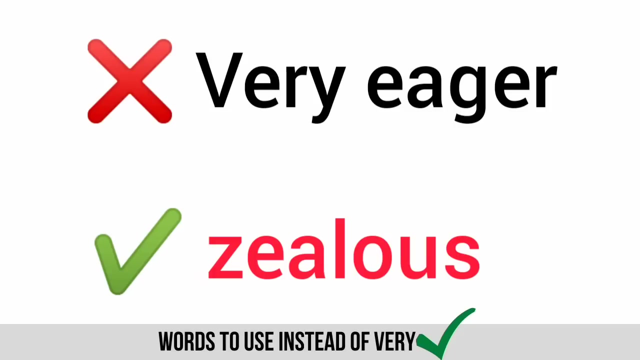 aggressive, Very emotional, sensitive, very emotional, sensitive, very frothy, effervescent, very frothy, effervescent, very amazed, very amazed, amazed, amazed, very amazed. Very low, Very low, shocked, very amazed, shocked, very eager, zealous, very eager, zealous, very fluffy. 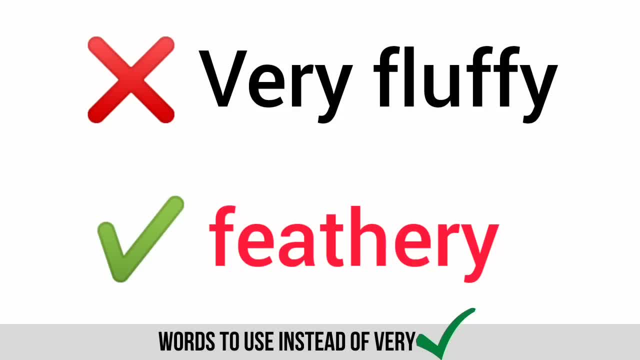 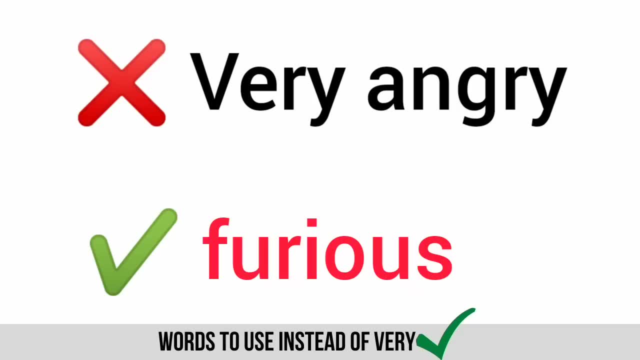 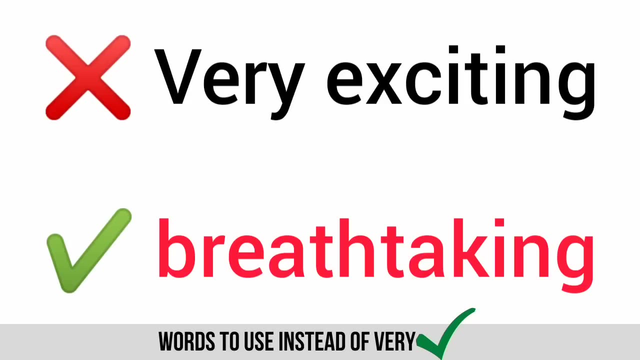 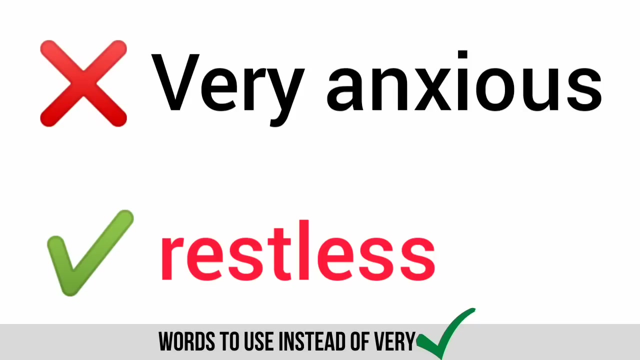 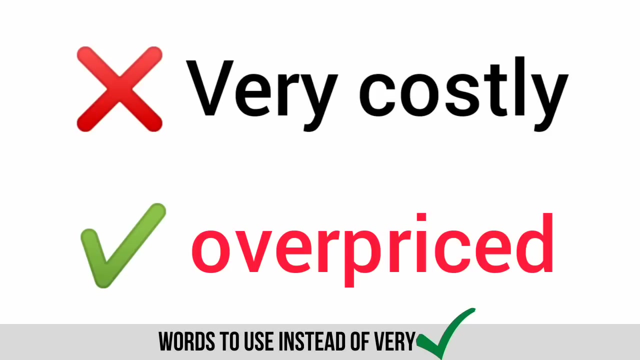 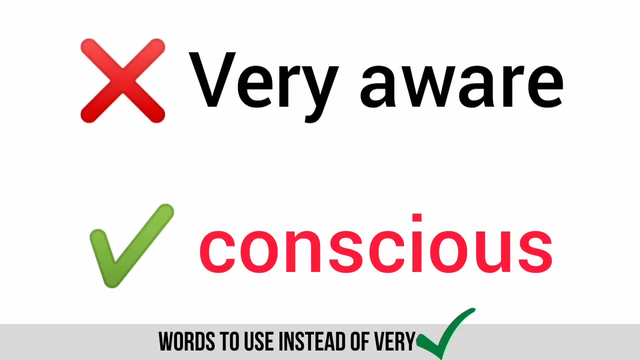 feathery, very fluffy feathery, very angry, furious, very angry, furious, very exciting, breathtaking, very exciting, breathtaking, breathtaking. very anxious, restless, very anxious, restless, very costly, overpriced, very costly overpriced. very aware, conscious, very aware. 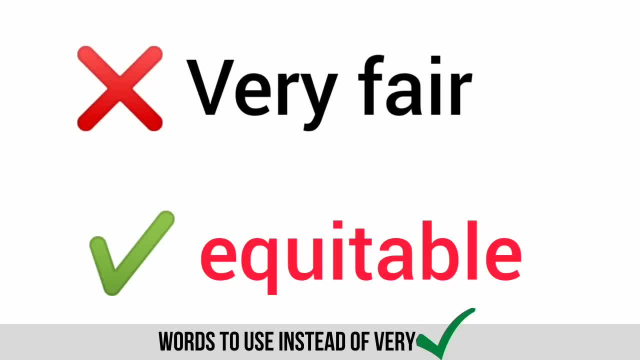 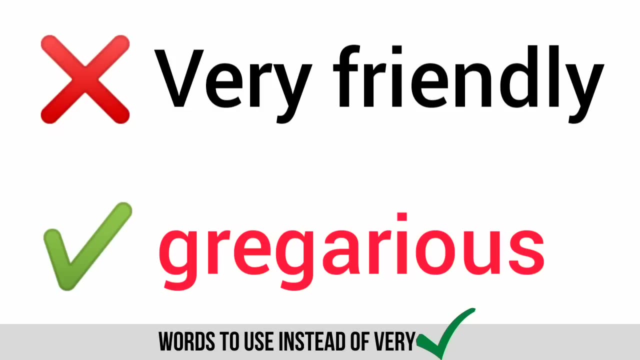 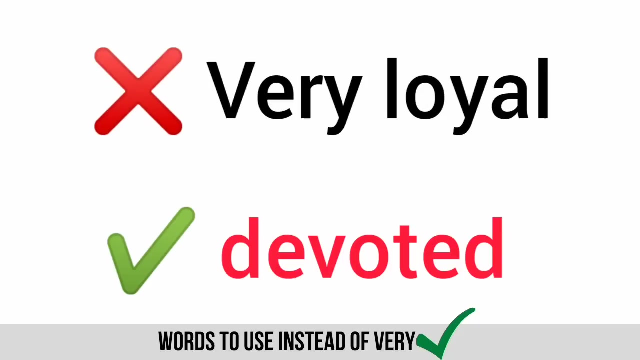 conscious, very fair, equitable, very fair, very friendly, vigorous, very friendly, vigorous, very loyal, devoted, very loyal, devoted, very loyal, devoted, very loyal, devout, very loyal, very friendly, 10 per cent very loyal. 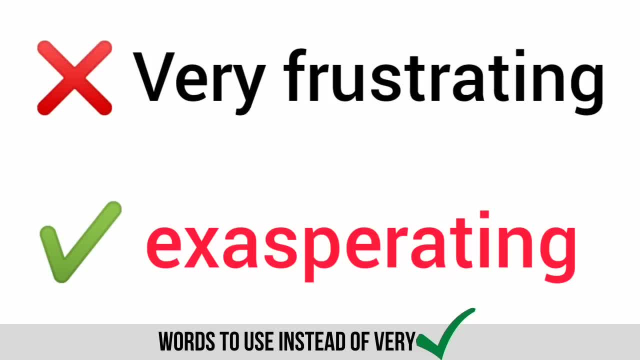 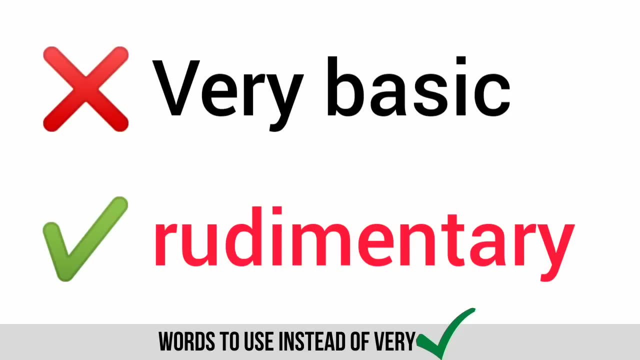 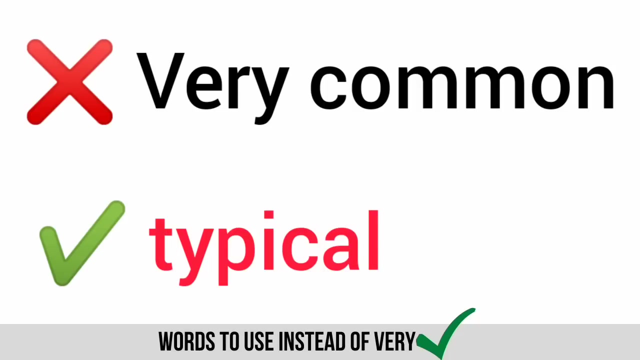 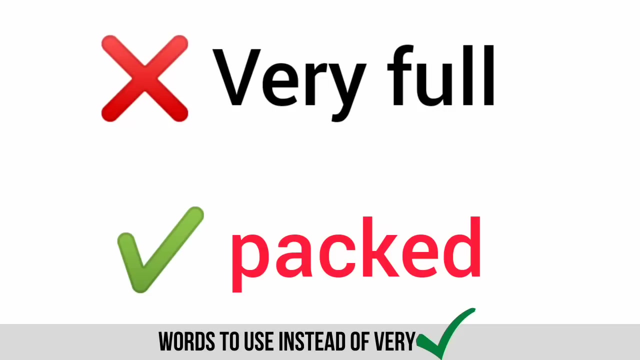 Devoted. Very frustrating, Exasperating, Very frustrating, Exasperating. Very basic Rudimentary, Very basic Rudimentary: Very common, Typical, Very common Typical. Very full Packed, Very full Packed. 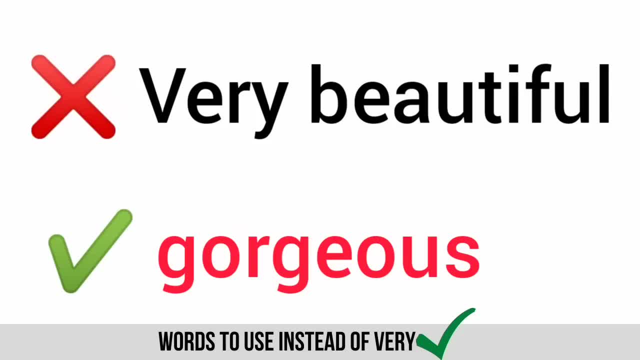 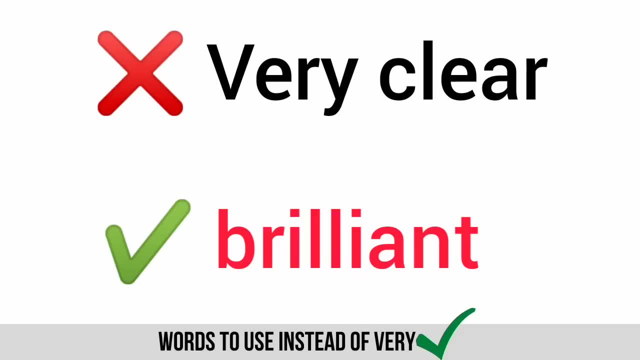 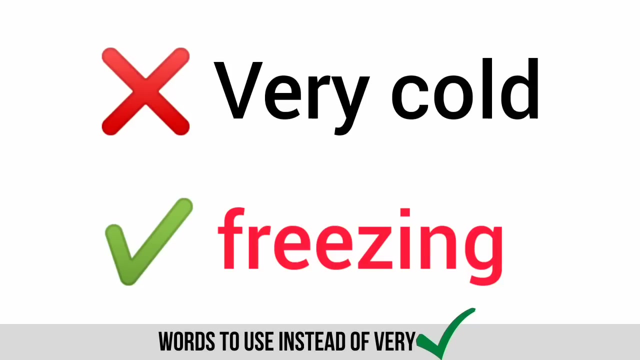 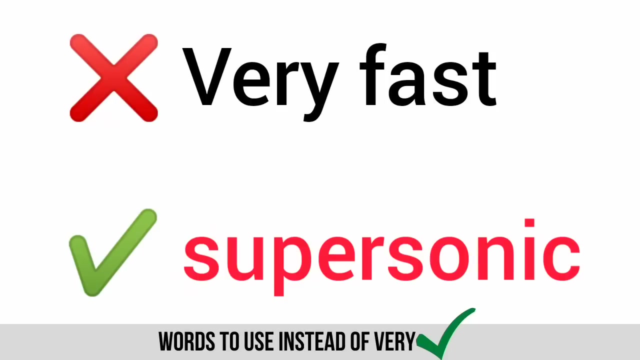 Very beautiful, Gorgeous, Very beautiful, Gorgeous, Very clear, Brilliant, Brilliant, Very clear, Brilliant, Very cold Freezing, Very cold Freezing, Very fast, Supersonic, Very fast, Supersonic, Very logical, Very logical. 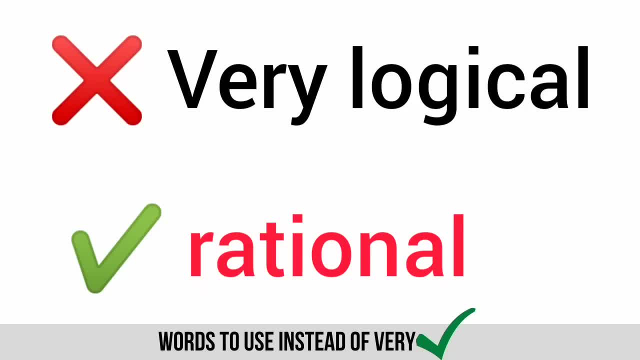 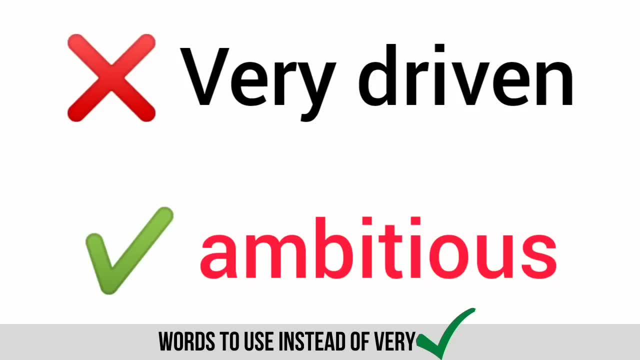 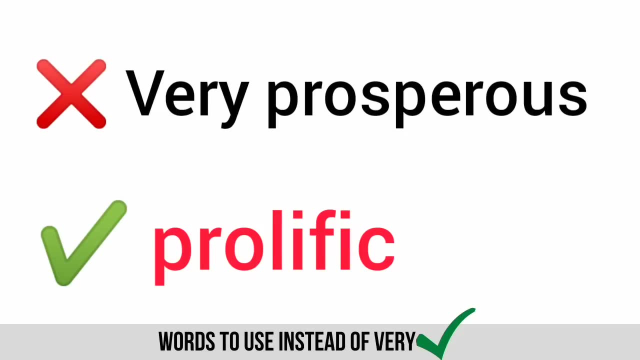 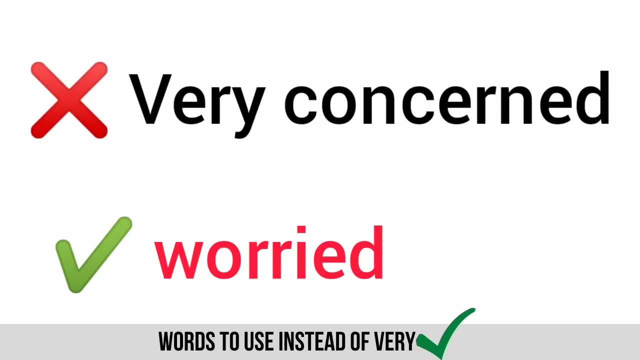 Right, Rational, Very logical, Rational, Very driven, Ambitious, Very driven, Ambitious, Very prosperous, Prolific, Very prosperous, Prolific, Prolific. Very concerned, Worried, Very concerned, Worried. 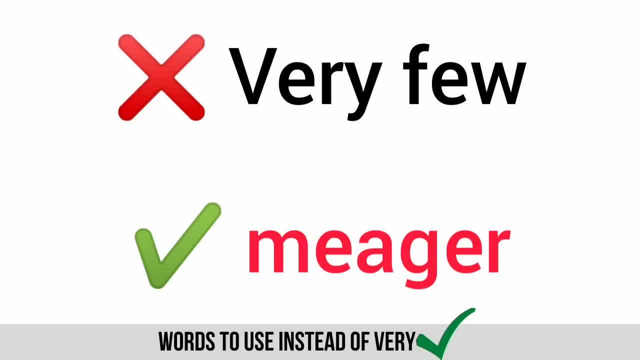 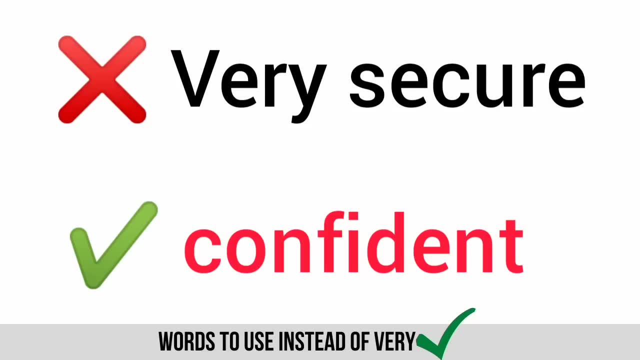 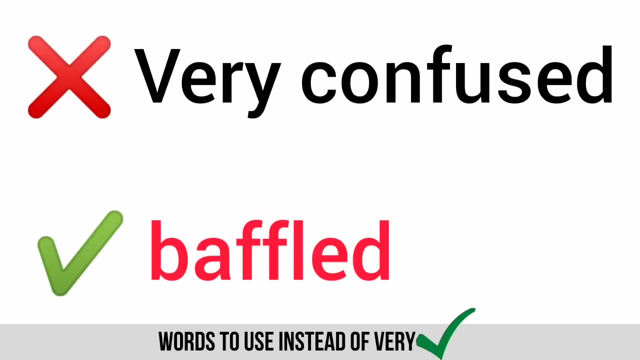 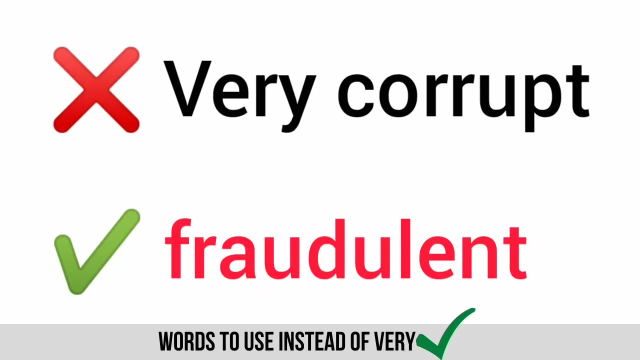 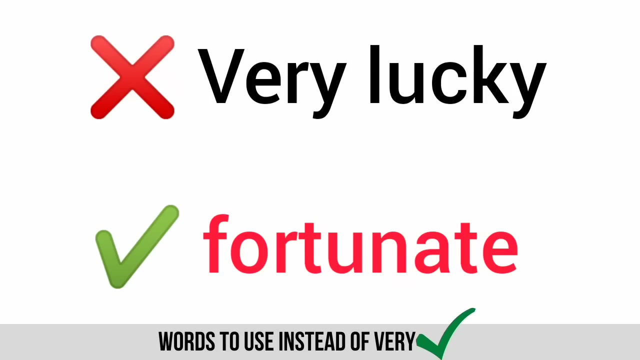 Very few, Meager, Very few Meager. Very secure, Confident, Very secure, Confident, Very confused, Baffled, Very confused, Baffled, Very corrupt, Fraudulent, Very corrupt, Fraudulent, Very lucky. 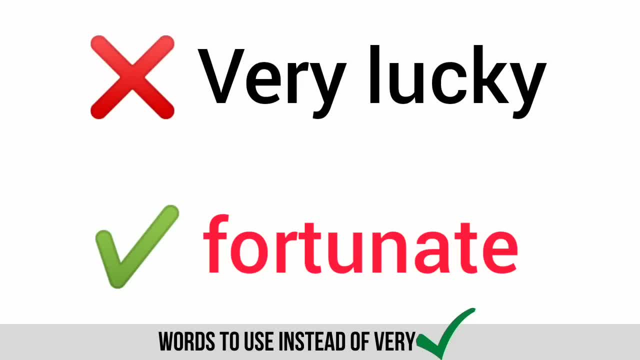 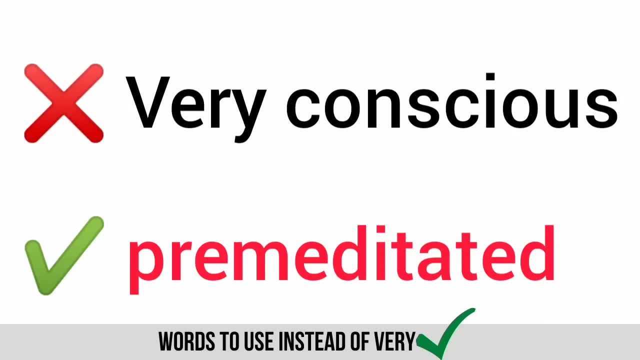 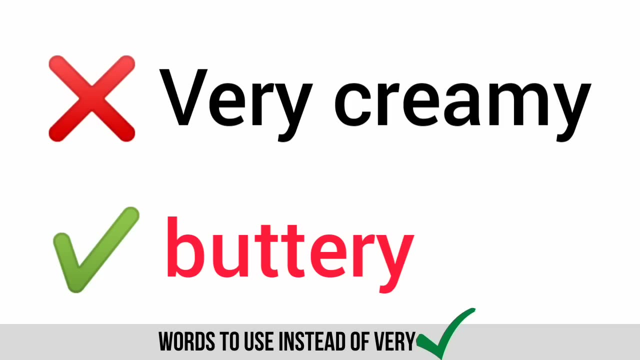 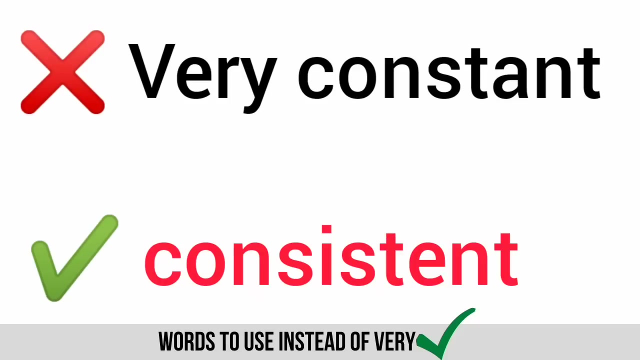 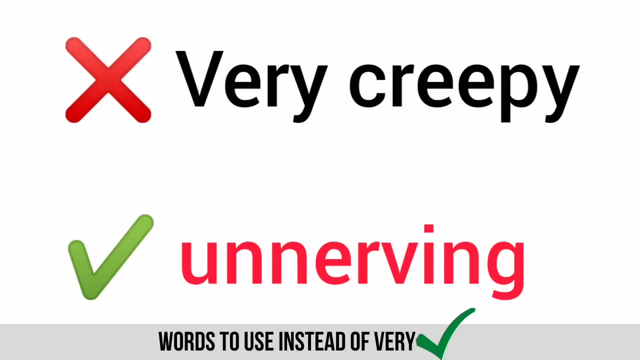 Fortunate, Very lucky, Fortunate, Very conscious, Premeditated, Very conscious, Premeditated. Very creamy Buttery, Very creamy Buttery. Very constant, Consistent, Very constant, Consistent, Very consistent, Very consistent.